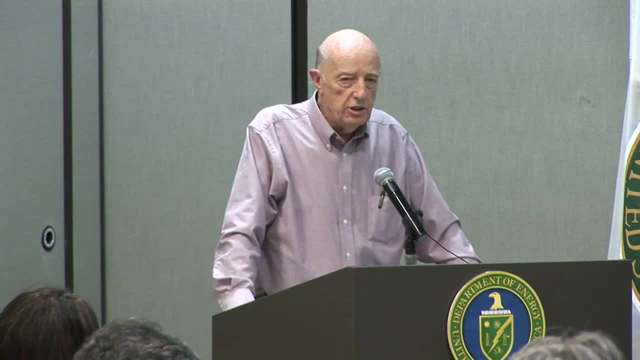 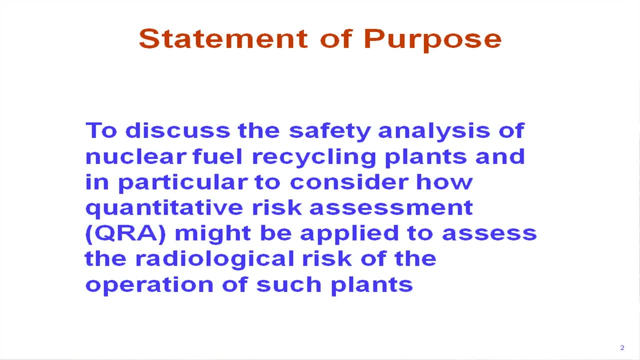 the risk of all manner of facilities. The methodology I'm going to share with you today- some of you are very familiar with it. The methodology I'm going to share with you today- has evolved over the last four decades. Our goal, the goal of basically the team that I've been associated with throughout my career, 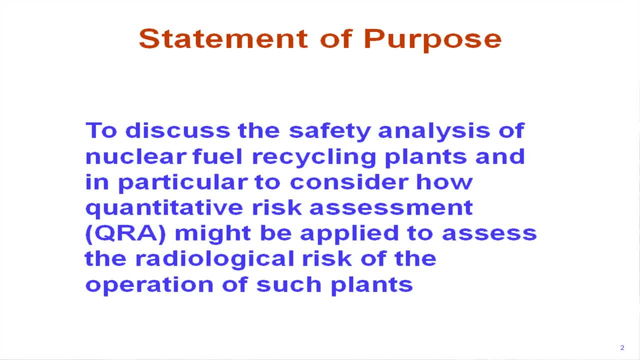 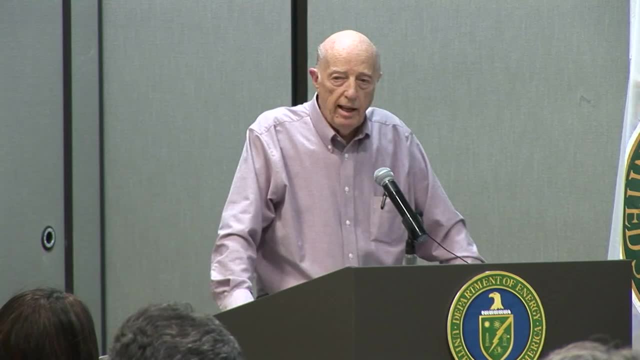 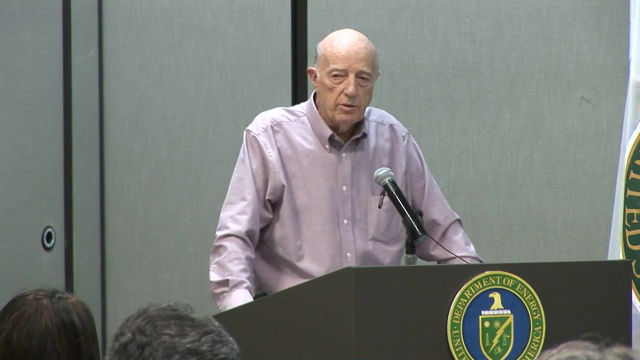 has to allow it to evolve to a general theory, a theory of risk assessment that can be applied to any kind of problem And while the boundary conditions are very different and the phenomenological issues are very different, and therefore the risk team should be made up differently for each application, there are certain principles, certain process steps. 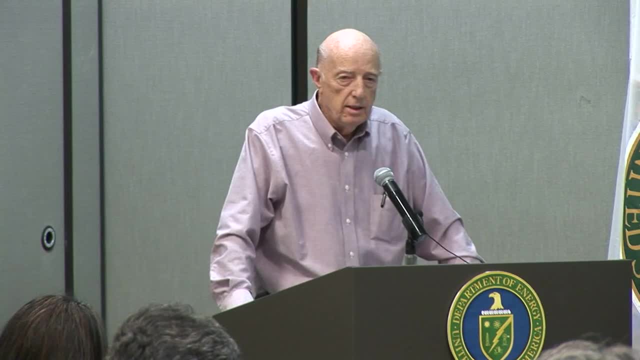 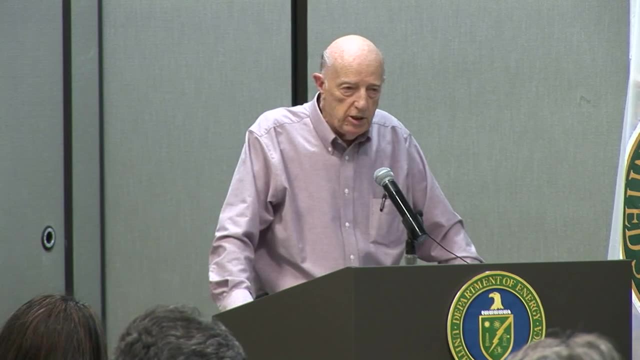 that have surfaced that seem to work well, Whether it's a nuclear power plant, which is where we've had most of our experience, a nuclear waste facility, which we've had quite a bit of recent experience, a chemical plant, analyzing such far out things as the import, the job market, things like that, education. 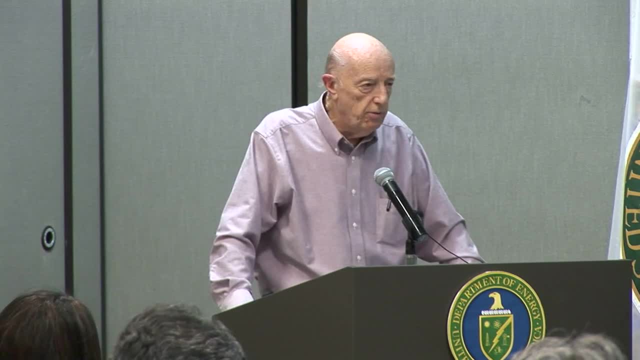 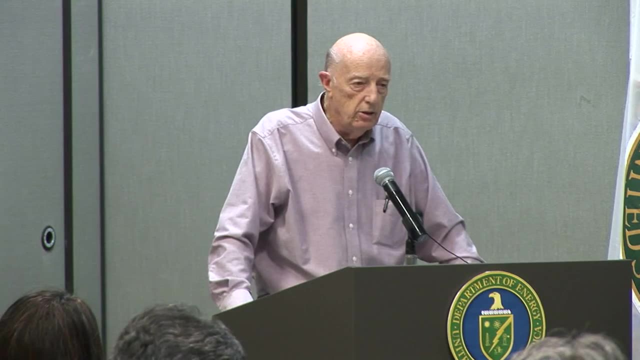 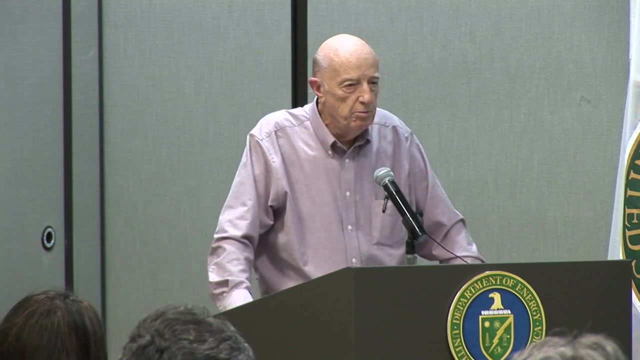 a chemical plant, analyzing such far out things as the import, the job market, things like that education risk of importing certain animal species into a population where that species doesn't exist. even did risk assessment in a cost-benefit trade-off of such 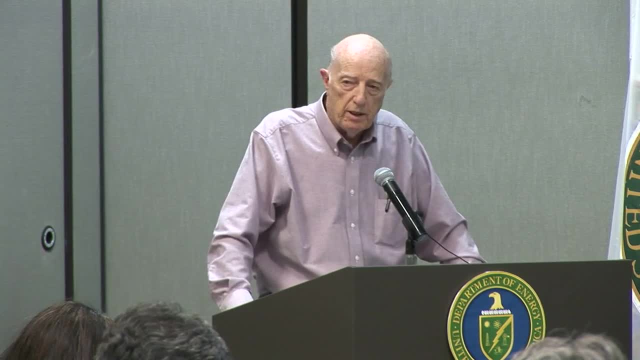 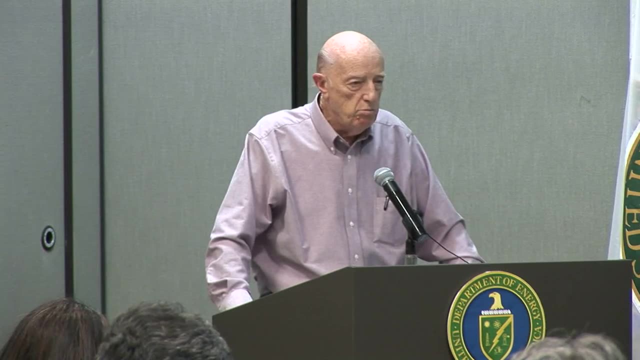 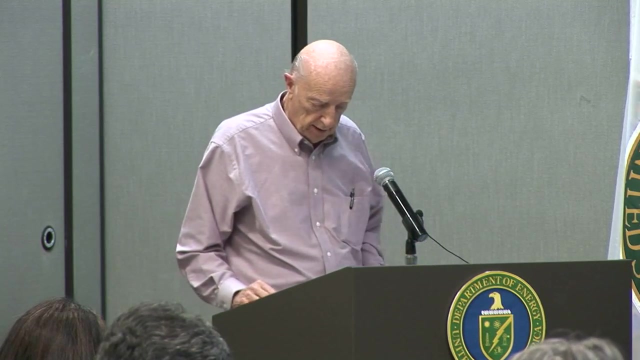 transportation issues, as the cost-benefit of going from special trains to regular trains, and some 50 or 60 nuclear power plants around the world, And so obviously you'd think that it would stabilize, and I think it probably pretty much has, and this is what I plan to do today When I say it has sort of stabilized. it's kind of stabilized at the high level, at the process step, and what seems to be at work each time is the implementation of some six basic steps. The first step is to create a system that can be used for the production of nuclear power plants. 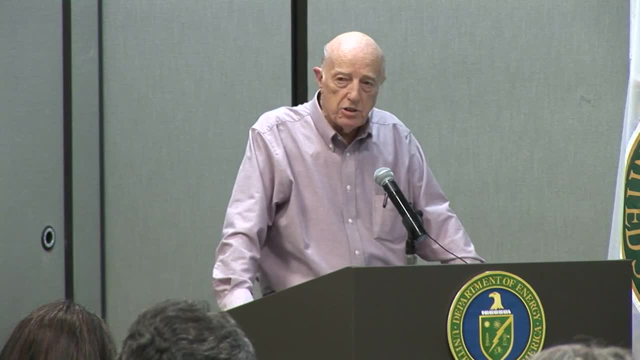 The second step is to create a system that can be used for the production of nuclear power plants. The third step is to create a system that can be used for the production of nuclear power plants, And so our goal, our hope of this evolving to a general theory, seems to be. 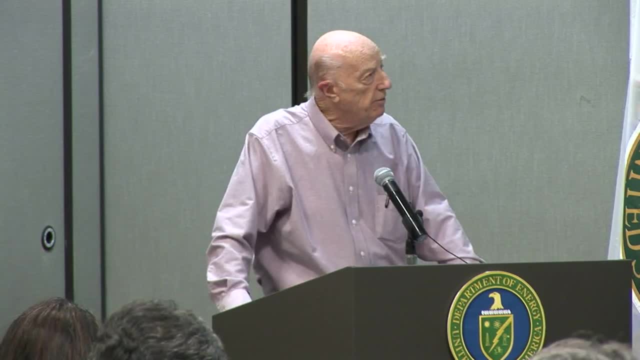 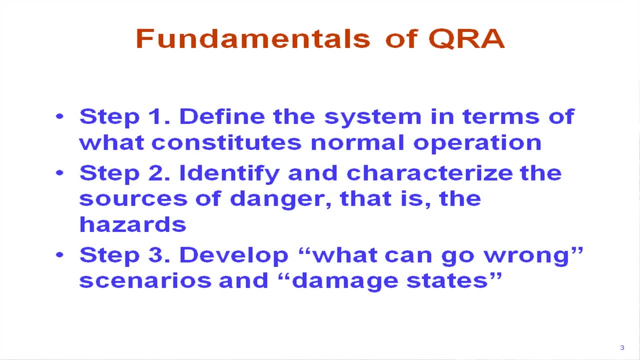 coming into fruition. First thing you have to do, of course, is understand the system that you're dealing with, And the biggest challenge of that in many instances is quantifying, if you wish, the success states of that system, And if it's a complex system, it gets particularly. 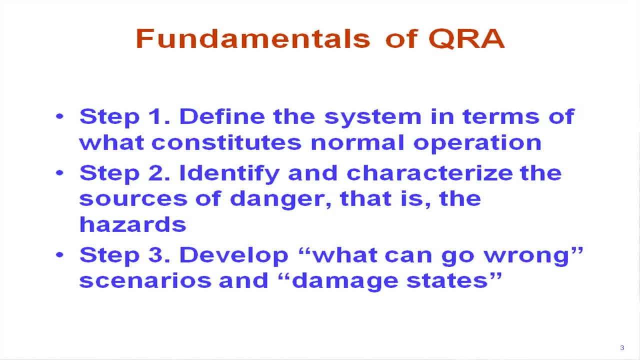 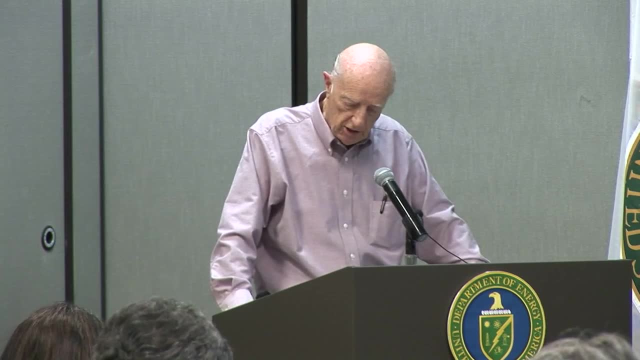 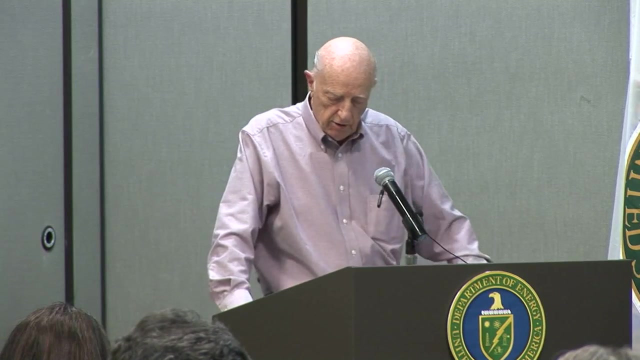 challenging, But you certainly need to know what represents an upset of any system, And so any departure from what you might define as a successful system is what you want to be able to expose. Number two: identify and characterize the sources of danger. We've done risk assessments. 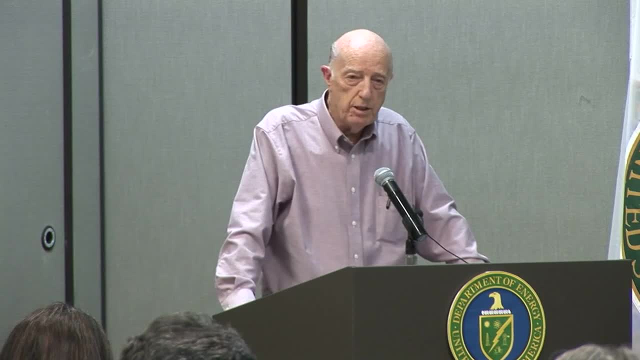 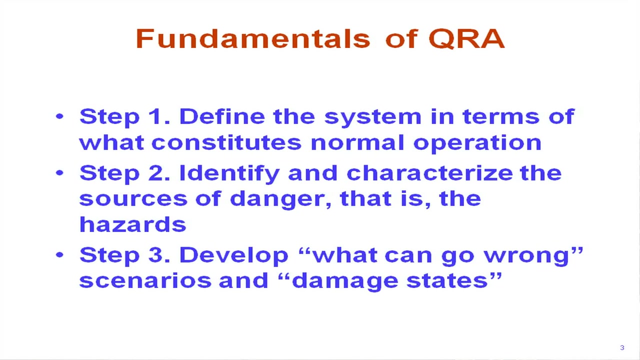 where the risk measure is the number of people who have been exposed to nuclear power plants. The risk measure was toxic, chemical or an explosion, or injuries or fatalities or disease or almost anything that was of particular interest to whomever we were doing the risk assessment. for In this case it's very easy: We're talking about radiation. 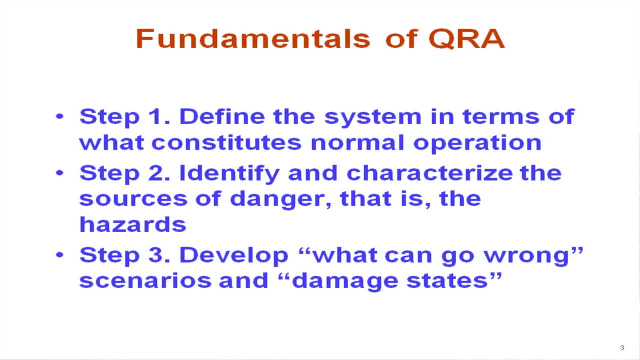 Develop what can go wrong scenarios and damage states. The methodology that I'm talking about is sometimes been referred to as the scenario-based approach to risk assessment, And so the cornerstone of the whole analysis is to develop the scenarios that represent as complete a set as you can develop with the things that can go wrong. 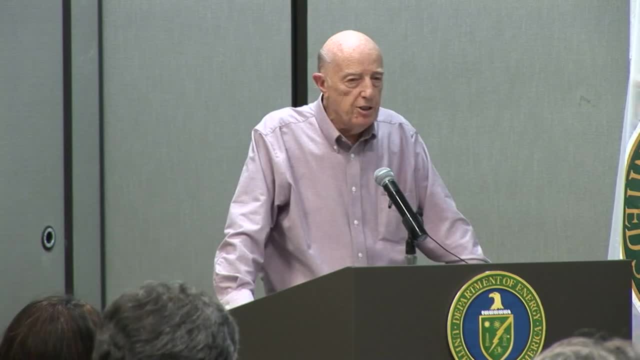 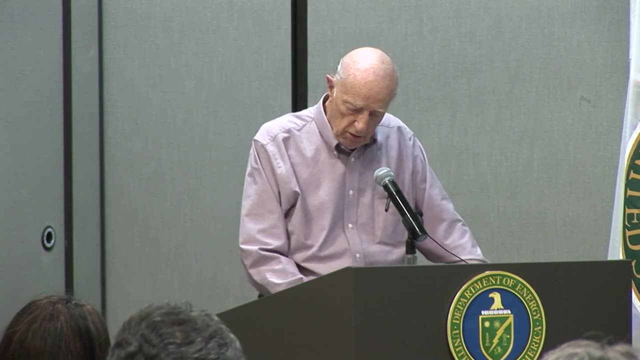 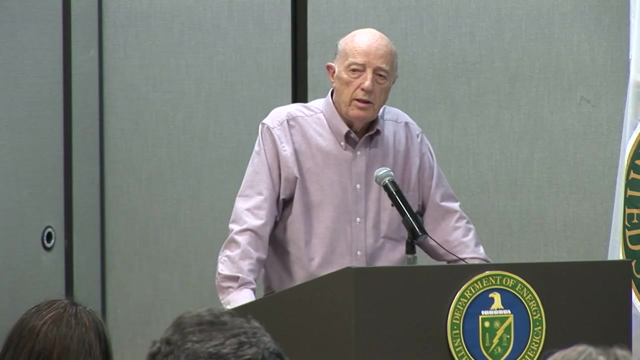 with the system And then the mathematical part, the development of the scenarios being created part. the mathematical part is the quantification of the likelihoods of the scenarios and the end states are the scenarios of the damage states. So when you quantified the 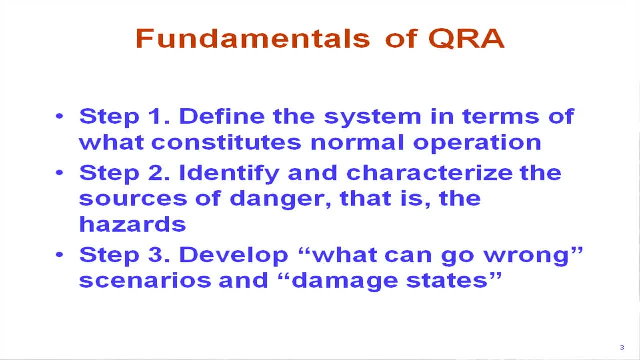 scenarios, you quantify the damage states And then, even after, you have the likelihoods of individual scenarios, which is an enormous amount of material, especially in case of some complex facilities. the number of scenarios may vary, few to millions, just depending on how the model proceeds. 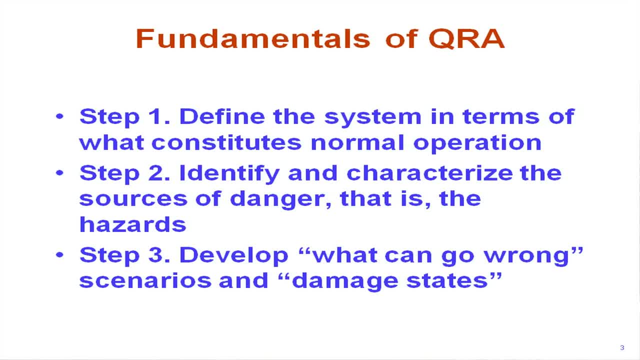 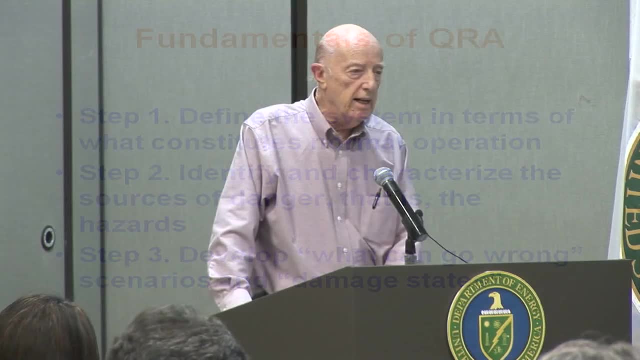 and how you've designed the risk measure that you want to compute and the level of detail you want with respect to the components and systems of what you're analyzing, And then so you need to assemble, have a means of assembling those scenarios into an integrated 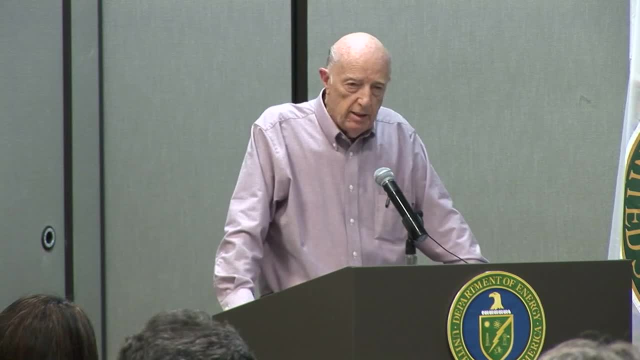 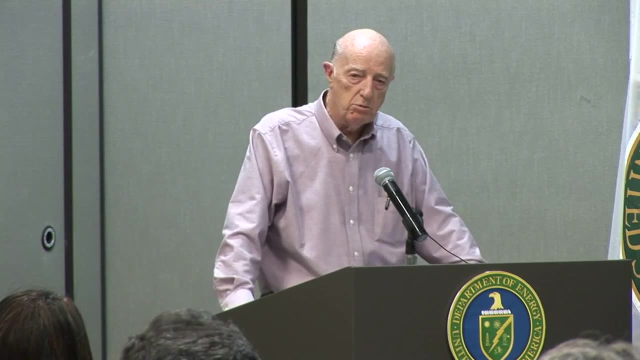 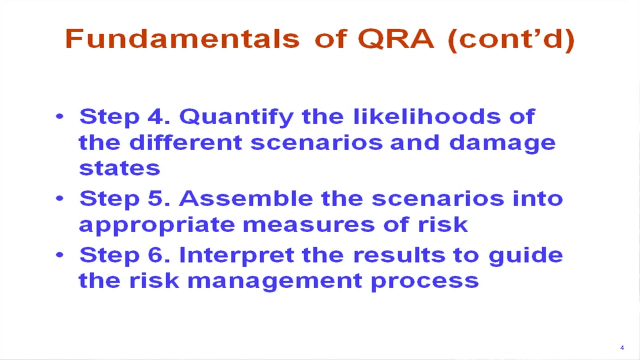 or complete statement of risk, and you want to do it in such a way that you can backtrack and provide some very important outputs with respect to risk management, such outputs as the relative contribution of the issues that are contributing to the risk. So the core concept of risk management, 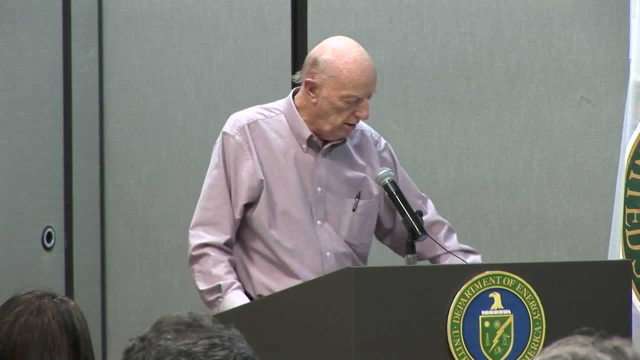 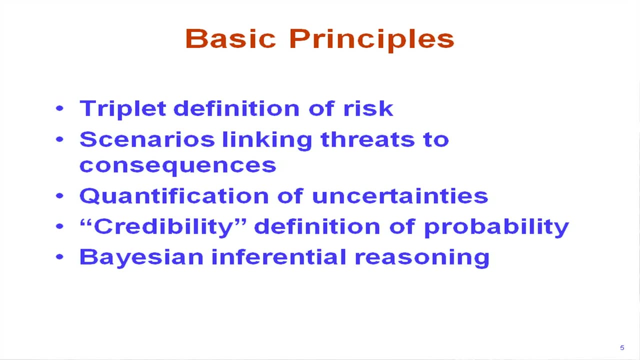 and the cornerstone of the process are these break-basic principles, and one thing I'd like to point out is that, of course, the reactor safety study represented a turning point in the way we think about nuclear safety, but most of the internals of this methodology were developed in the private sector. 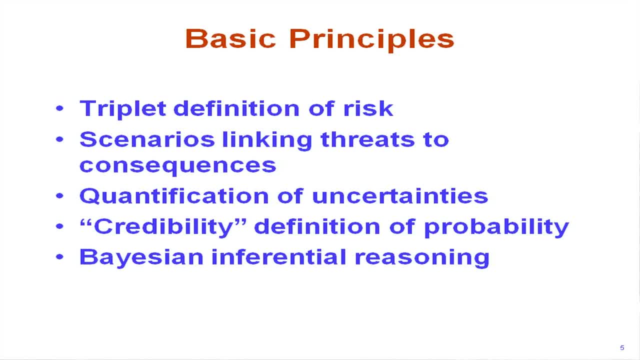 The first big boost we got my company many years ago was we dominated the risk assessment business in the nuclear power field. Our little team- and it was a little team and we had about 150 employees total- we were responsible for something like 45 US plants and another 10,. 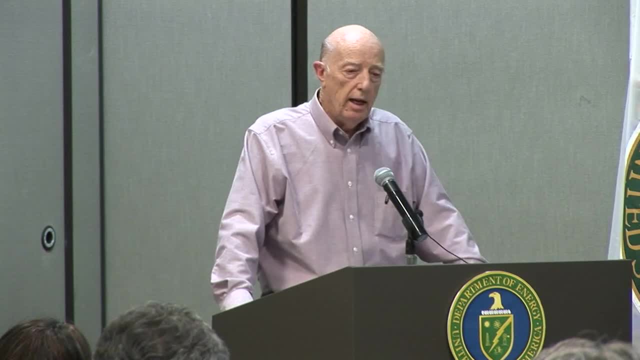 15 international plants and we just couldn't- almost couldn't- keep up with the business during the 70s and the 80s And then when we got to the end of the 20s and the 30s, 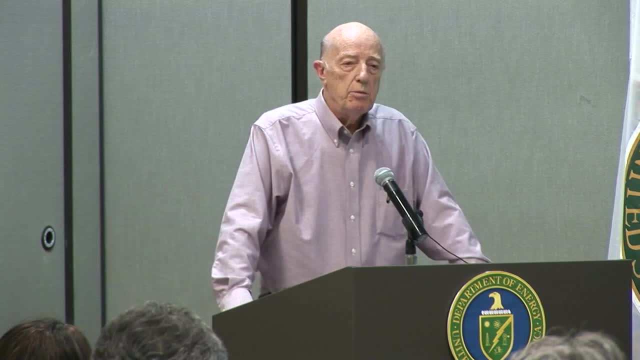 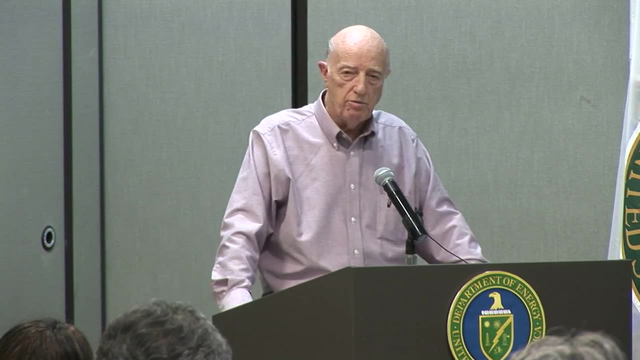 we were able to do a lot of things. We were able to do a lot of things. When the NRC got in the business, things changed a little bit, because our whole thrust was to what we called full-scope risk assessments. We indeed wanted to quantify the health effects. 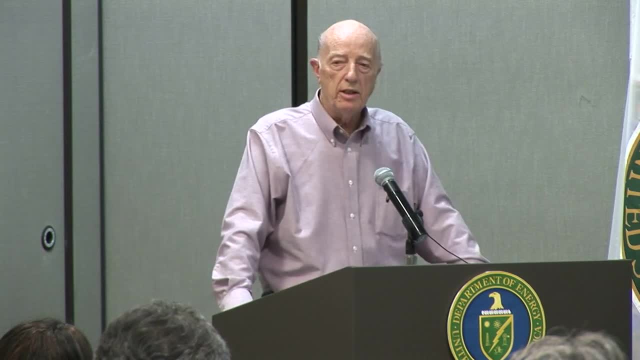 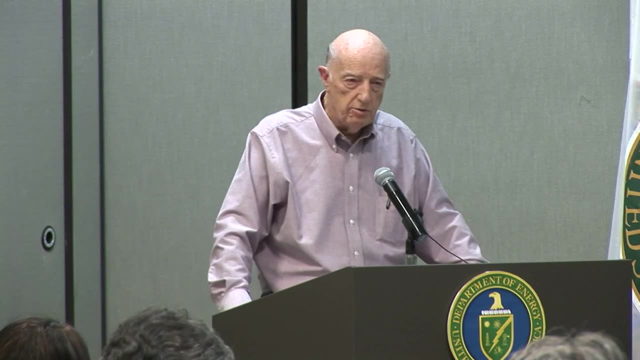 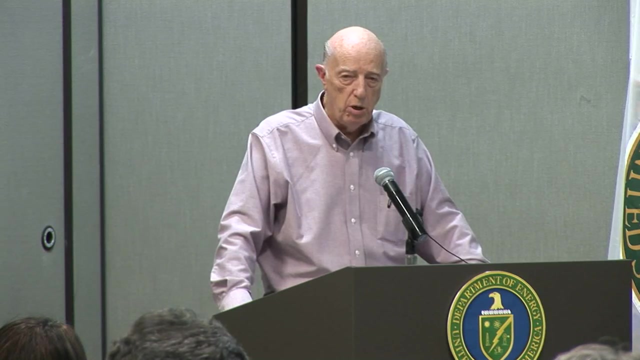 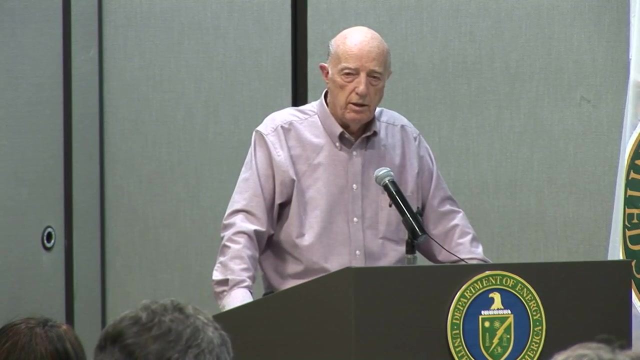 and while there was lots of grumbling and grousing in the business about the inadequacies of the models, particularly the health effects models, with what we had done with respect to uncertainty, we felt confident that the amount of information we could get would be enormously beneficial. 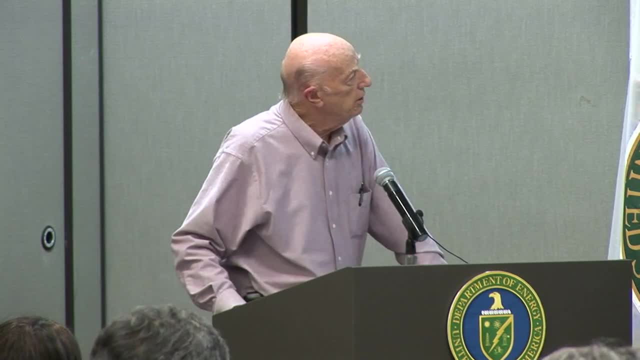 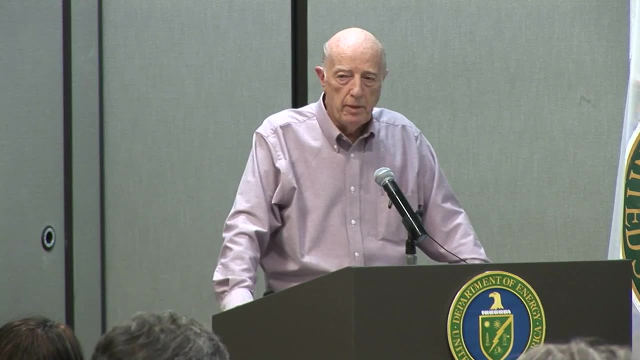 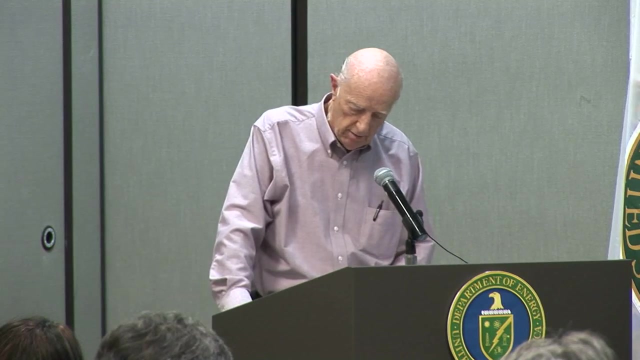 So this is what is the backbone of the approach: The triplet definition of risk. this started in my PhD thesis, which was really given substance in 1981 with my colleague Stan Kaplan, who, by the way, just passed away from Alzheimer's. 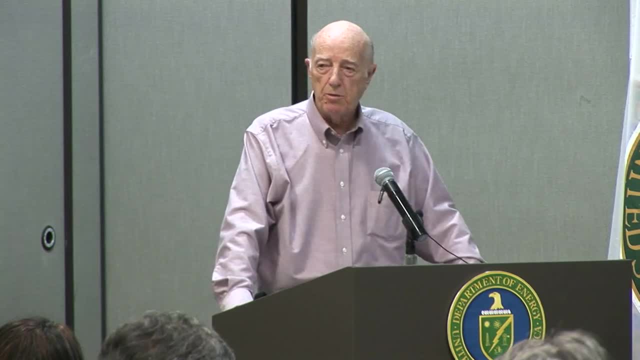 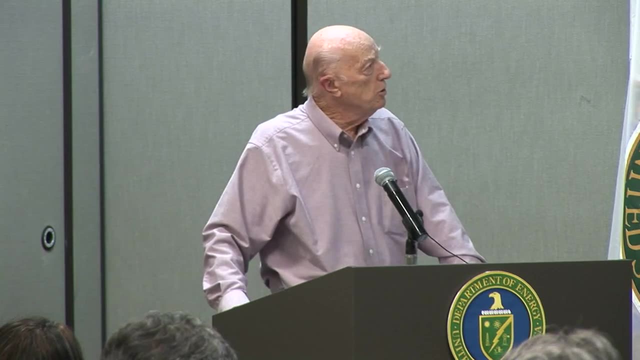 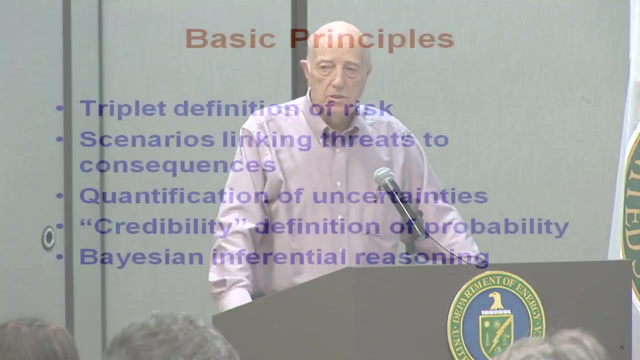 Alzheimer's disease, when we published the first paper in the first journal, in the Journal of Risk Analysis, which was, by that definition, a quantitative definition of risk Scenarios. scenarios are the foundation, cradle-to-grave scenarios from initiating events. 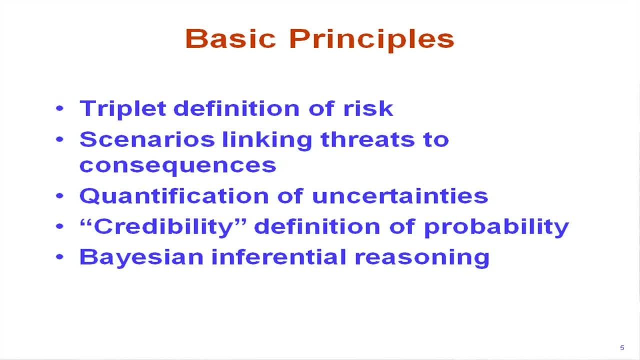 to damaged states or, if you wish, from initial conditions to damaged states. And then the thing that we spent the most analytical energy on was our uncertainty models. We were really the first to put uncertainty in our fundamental risk models, not as an afterthought. 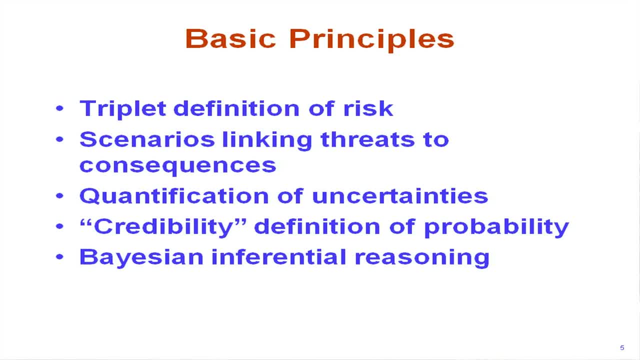 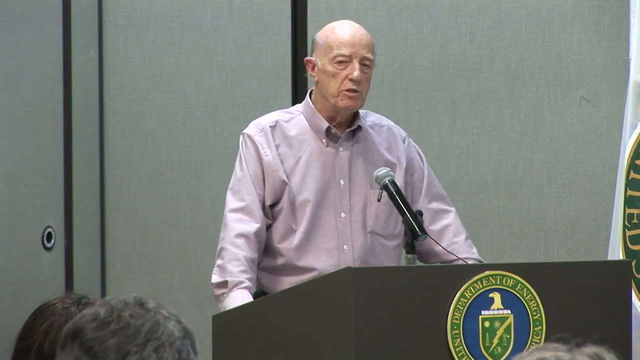 but as an inherent feature of the modeling process. And then we did something else. We adopted what I would call- and I'm not going to go into too much detail on this- but we adopted an engineer's definition of probability, Not a classical definition, not a frequency-limiting definition. 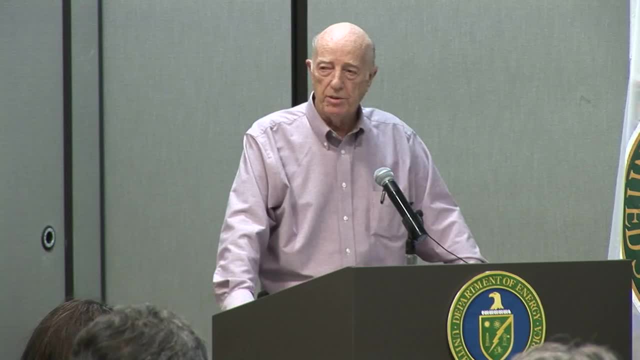 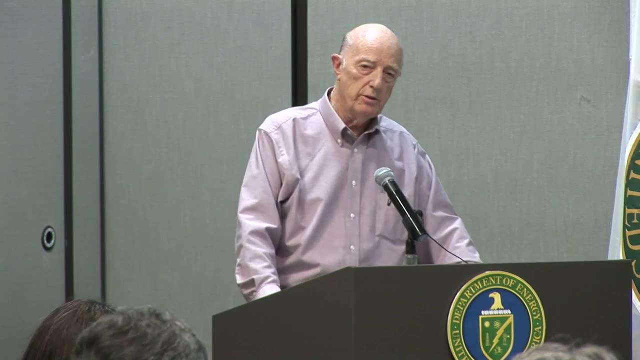 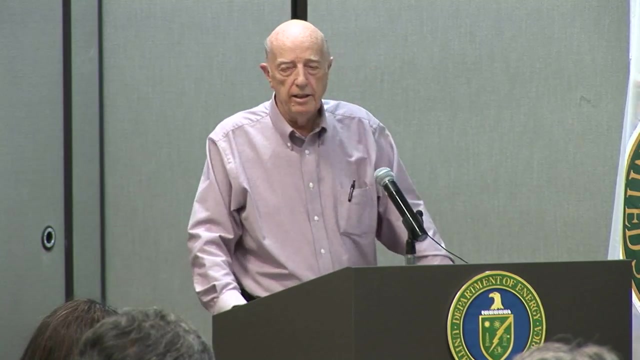 but a definition that was very simple but enormously helpful, And that was that we even considered the idea of not using the word probability but rather using the word credibility. But we decided we'd leave it as probability And that definition, of course, is just simply the credibility. 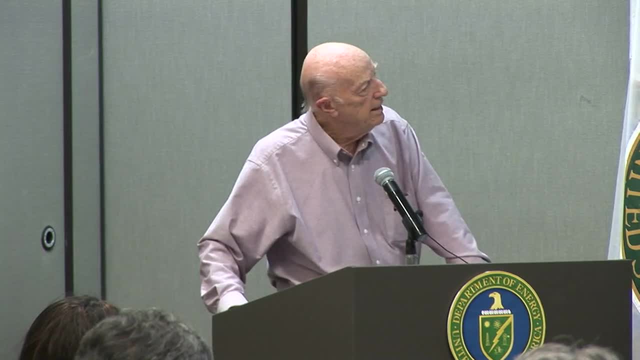 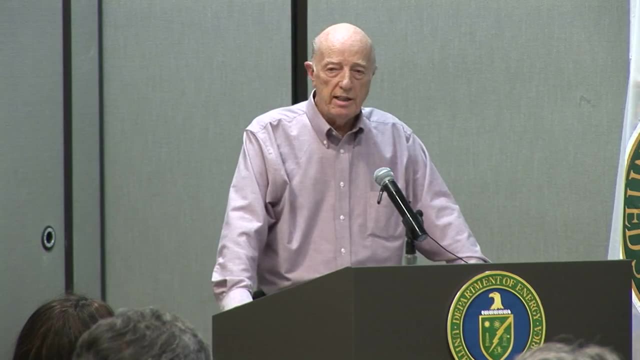 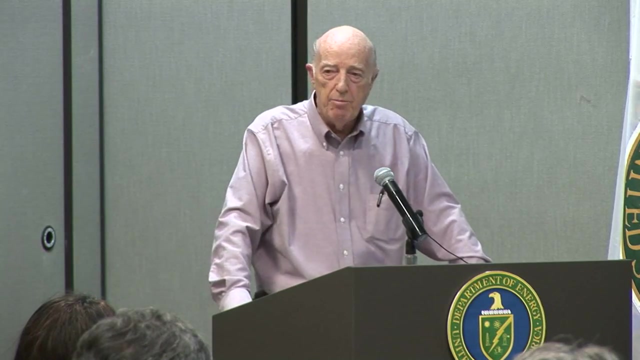 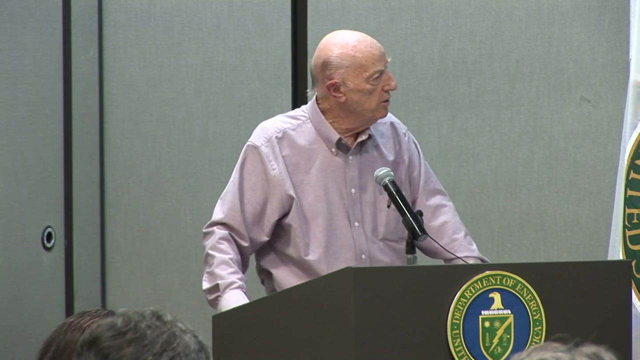 of a hypothesis Based on the supporting evidence in the form of a number from zero to one. And then, since Bayes' theorem embodies the fundamental rules of logic and plausible reasoning, we became very Bayesian and had to be sure that all of our probabilities obeyed Bayes' theorem. 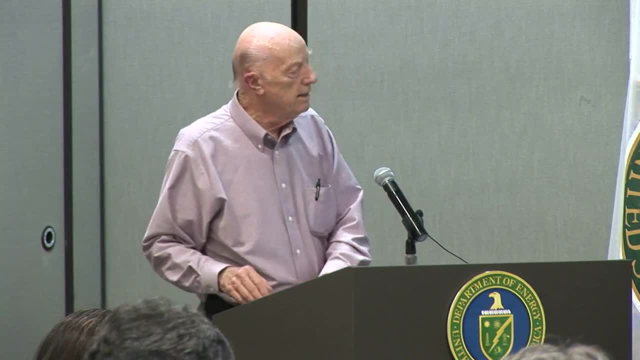 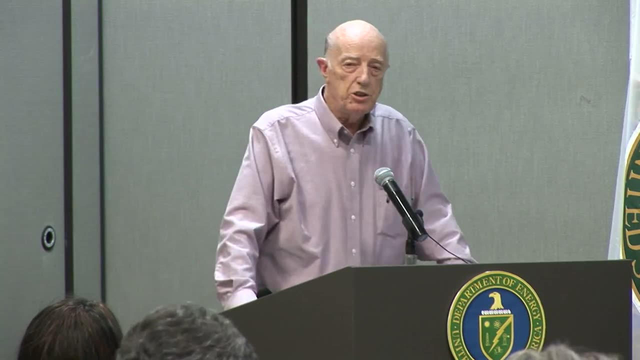 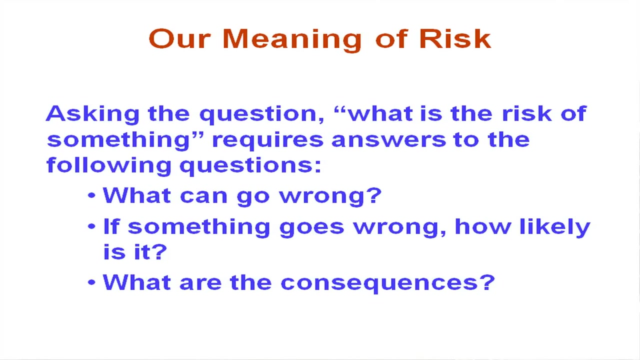 So this was the process. Now, what do we mean when we talk about the triplet definition of risk? Well, that could be a short course in itself, and it has been in the past at MIT and at UCLA and other places, But at a high level. this is what it's all about. 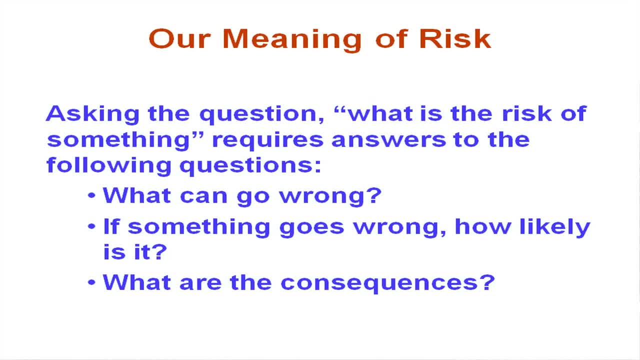 When we ask the question, what is the risk? we're really asking three questions, And they are: what can go wrong with our system? And the system can be a natural system, or it can be an engineered system, or it can be a natural system. 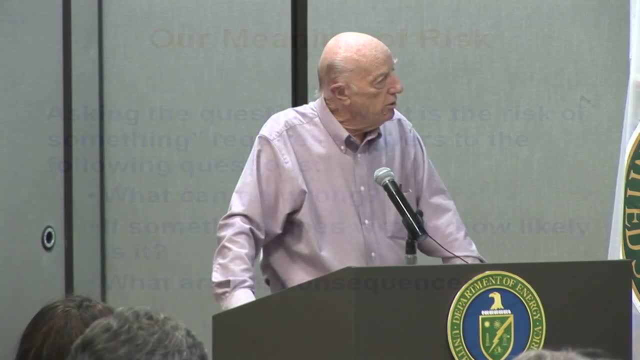 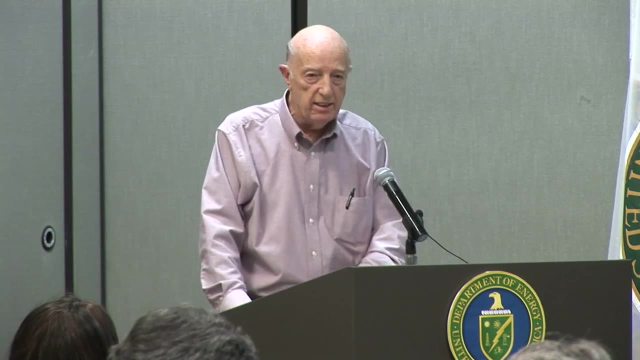 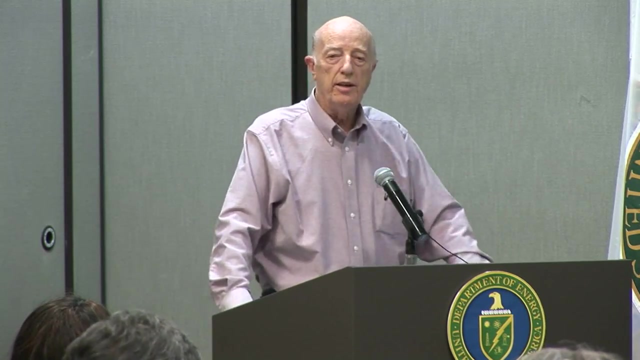 And if something does go wrong, how likely is it And, of course, what are the consequences? Now, there's been a tendency over the years, as people have referenced this paper or this approach, to want to add other bullets, For example, another bullet that you'll see. 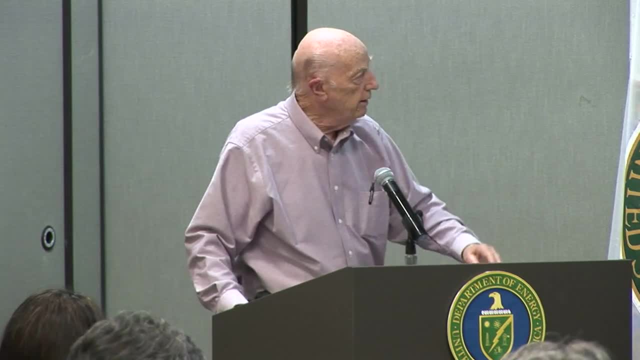 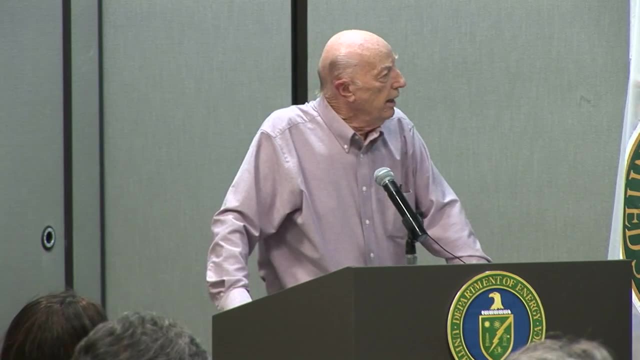 in the literature is: what are the uncertainties? Well, that's embodied in the second bullet, in how you define your likelihood function. We always include the likelihood function, We don't include uncertainty. And they also add that the bullets sometimes take corrective action. 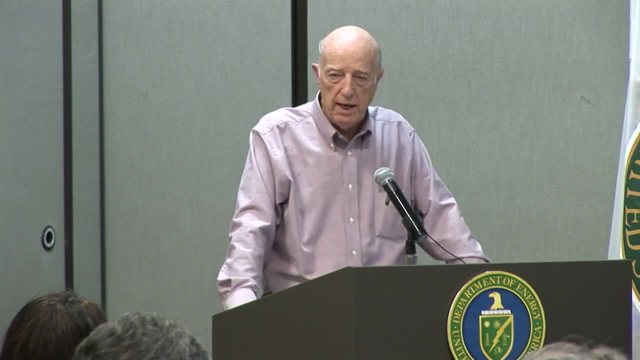 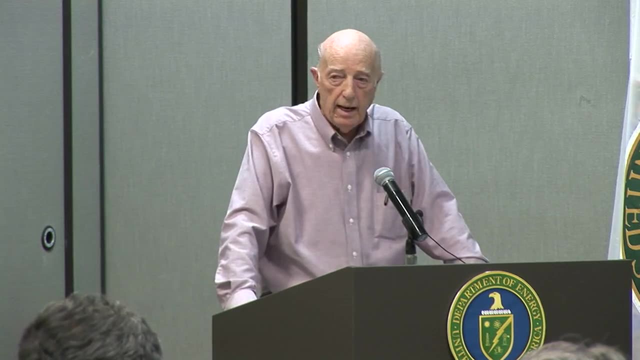 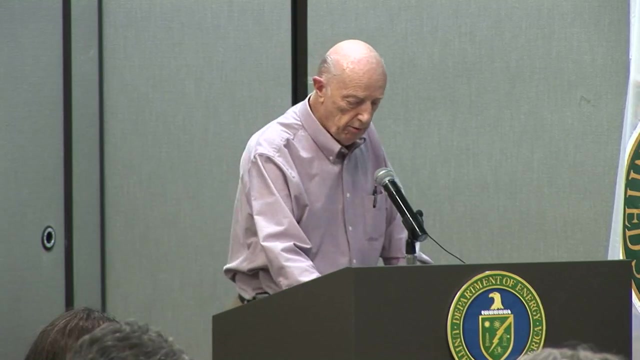 Well, that's not a risk assessment action, That's a risk management action. So we tried to keep it very clean, very compact, and built the analytical infrastructure around that, And so this is a little bit of an example. This is our notation that we've adopted. 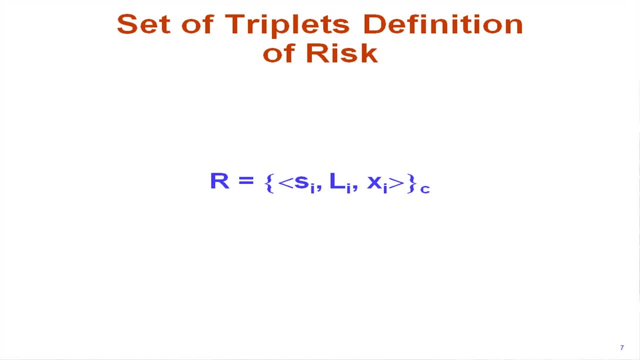 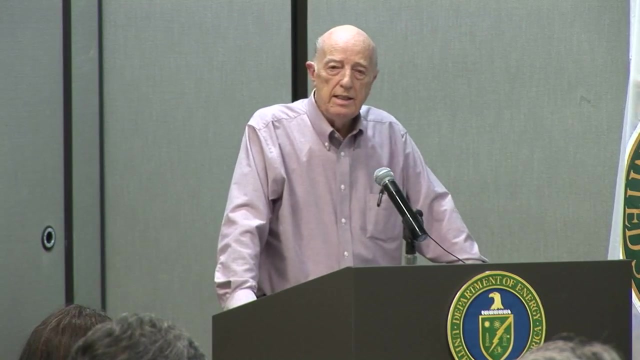 for what we mean by risk: The inner brackets really enclosing the triplet, the outer brackets implying the set of and the subscript C implying the complete set of. Now, of course, you don't always find the complete set, but we've found that we can have very good luck. 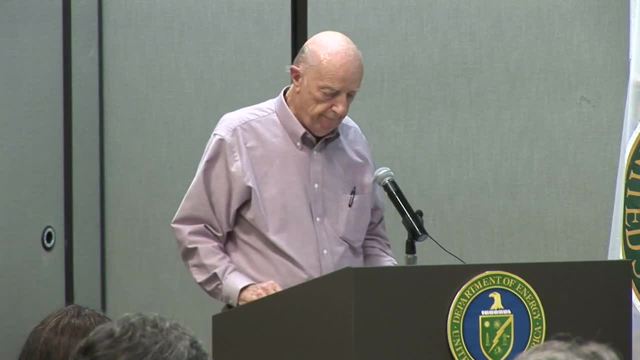 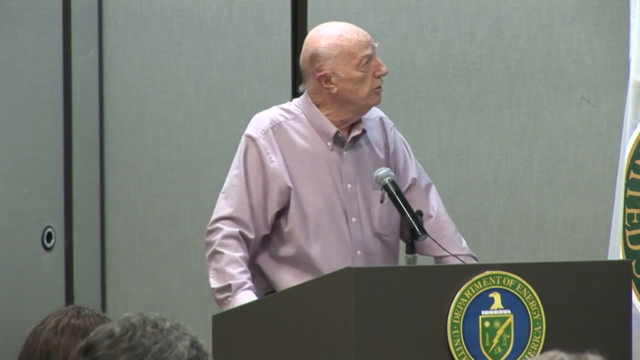 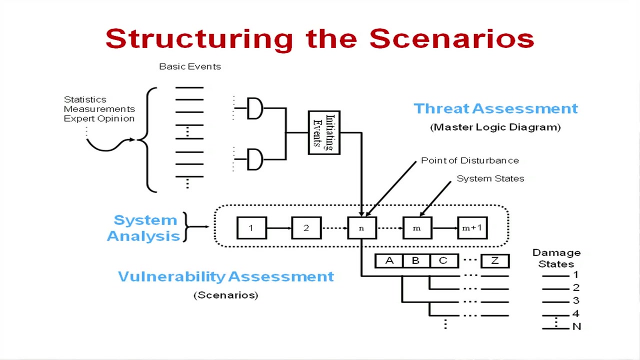 at getting the most mostly important ones. So, So let's go into it a little bit and just ask ourselves: what process do we go through to structure the scenarios? And it really the six steps that I outlined for you tend to collapse into three major analytical activities. 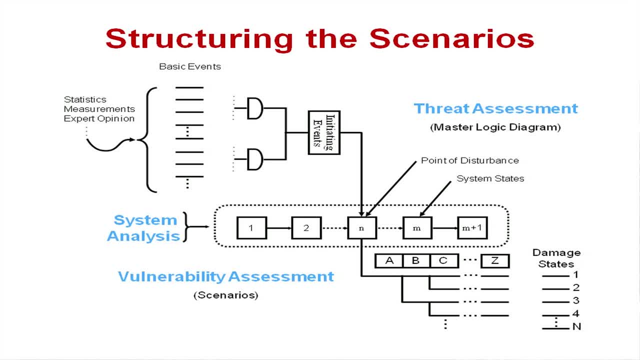 The first one is the middle one, understanding what the system is, And, of course, something we learned very early was that you know we're going to have a lot of problems, And the first thing we learned was that the more you can linearize the system, 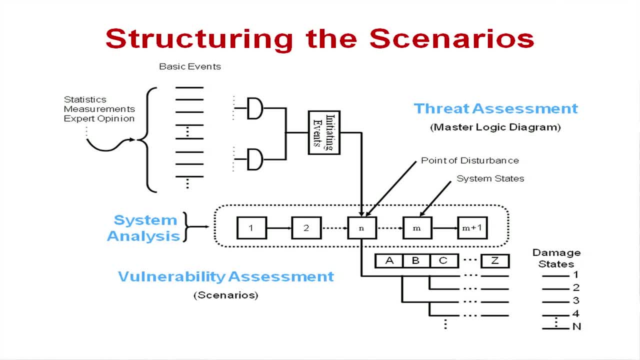 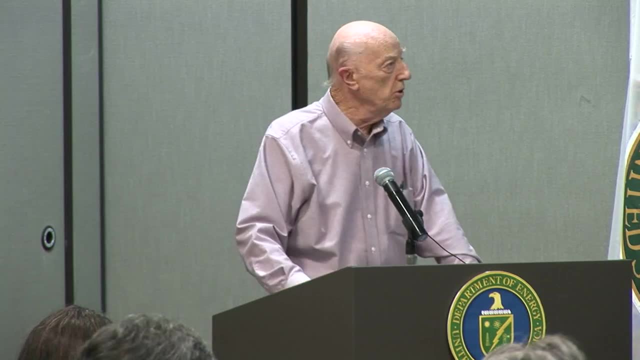 the better off. you are such that in a system that's A, B, C, 2, or 1,, 2,, 3,, 4, that 1 leads to 2 leads to 3, and so forth. In other words, you try to cast the system whether it's a natural system. 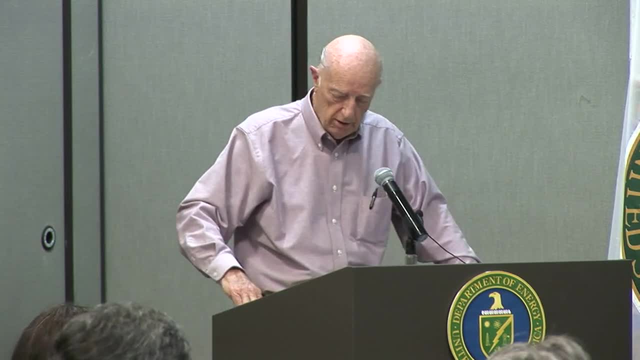 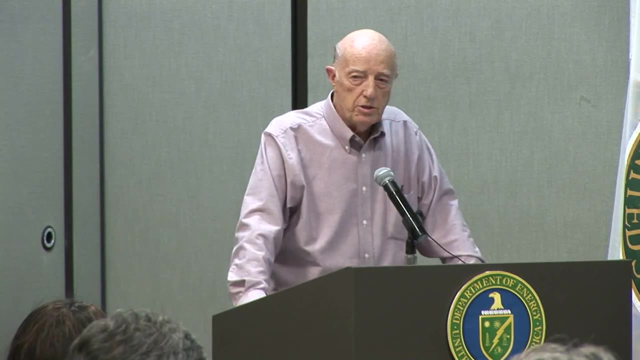 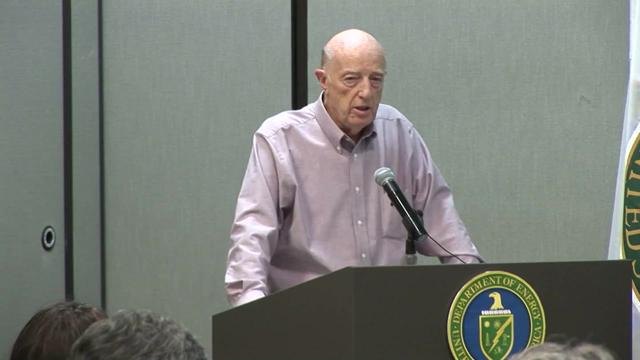 or an engineered system into what the mathematicians might call a linear vector space, And you want to do that because it gives you- you know, it gives you- the whole arsenal of matrix mathematics at your disposal, And that becomes enormously beneficial, which you can't do. 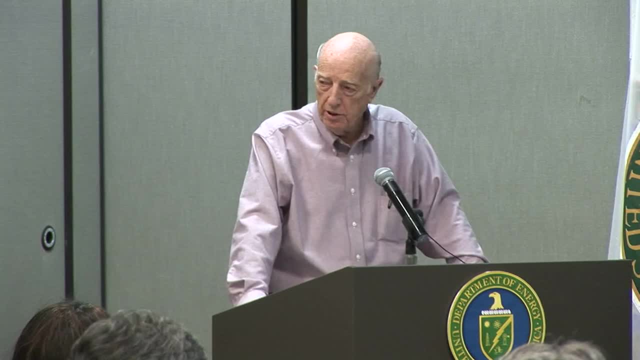 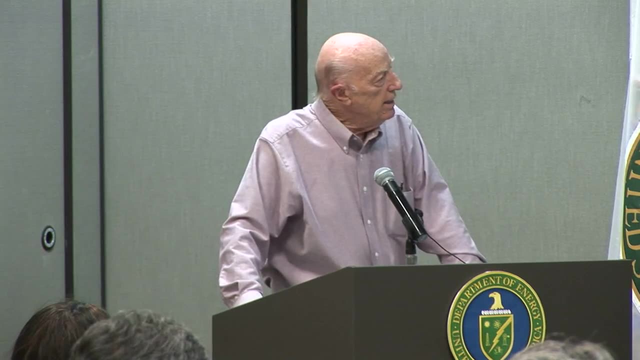 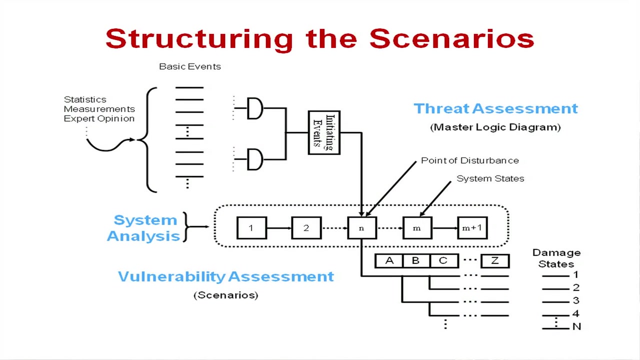 if your risk assessment is just fault trees, Because a fault tree space is not a linear vector space, But an event tree is a linear vector space, And so you would like to have your model such that you structured it in a way that you can define the output states. 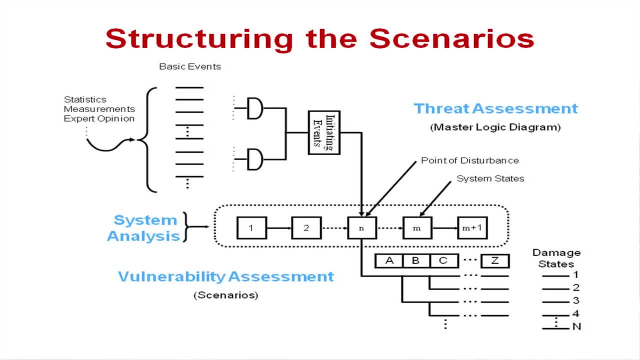 in each, from each of those boxes. For example, in the nuclear power plant case we had the, we had the plant model and we had the containment model and we had the site model. So the end states of the plant model were plant damage states. 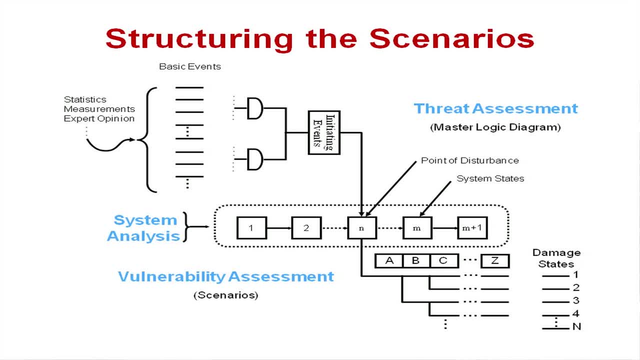 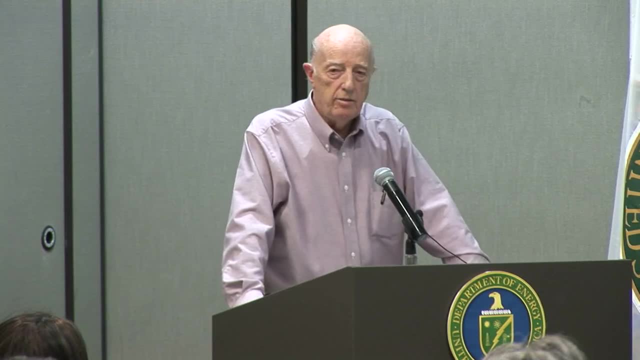 The end states of the containment model were the release categories And the end states of the site model were the was the dose ranges. So- And that is where a lot of the risk assessments fall down- Is that they have not taken the time that's needed. 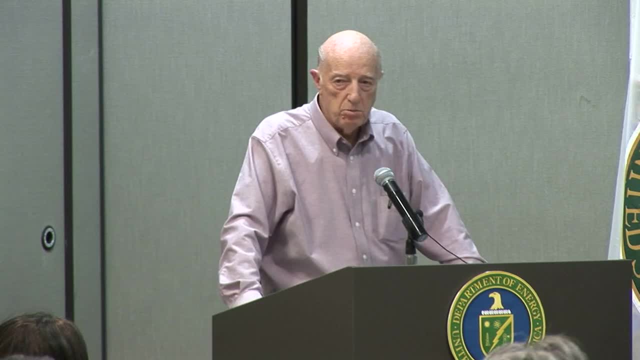 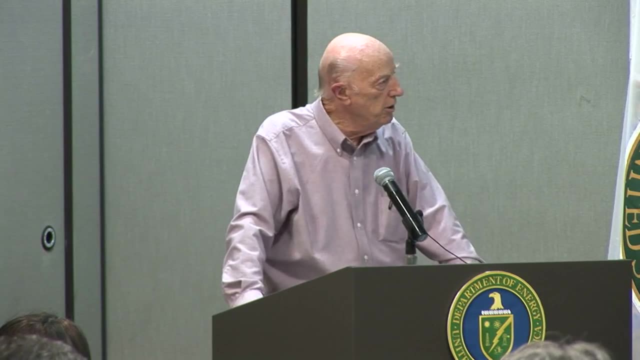 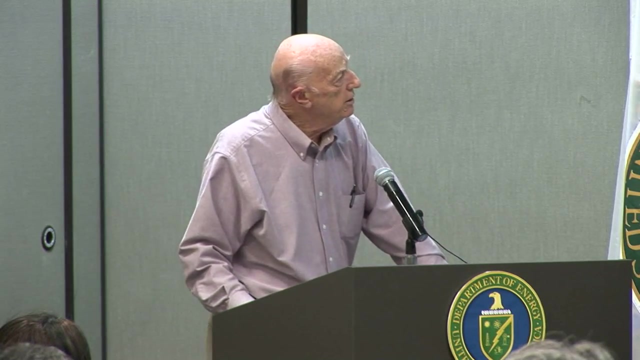 to characterize just exactly what the system is And the part- the part of it- that's often neglected is the part of it that turned out, in the nuclear power case, to be the most important, And that is the support systems, The, the one that's sometimes the most difficult. especially in the nuclear power system, is the support systems. The one that's sometimes the most difficult, especially in the nuclear power system, is the support systems. The one that's sometimes the most difficult, especially in the nuclear power system, is the support systems. 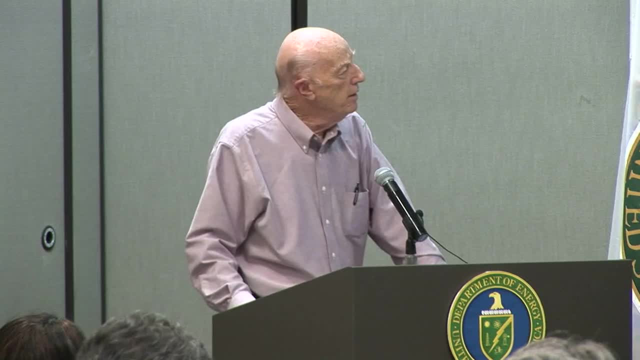 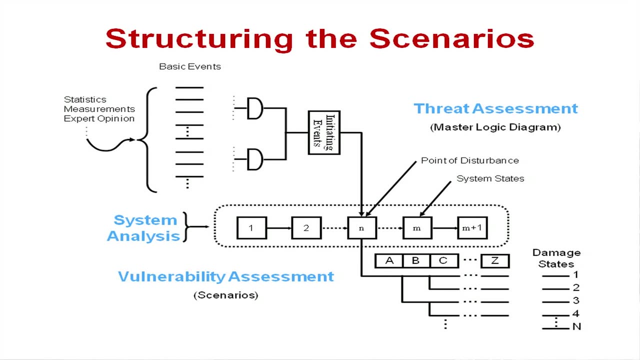 And that's the part that is most difficult, especially if it happens to be a terrorism risk problem- is the threat assessment. We, we sort of have adopted a kind of a master logic diagram. It takes the form of a of a fault tree, as as where the top event is the initiating event. 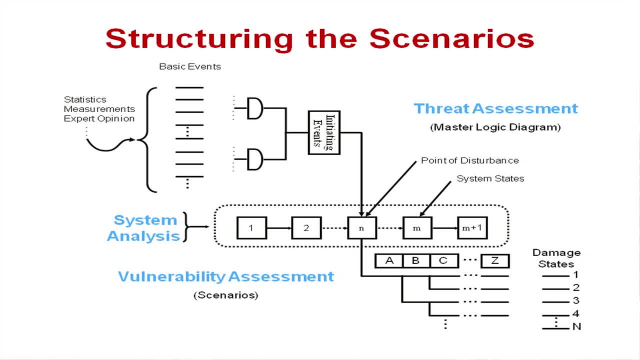 or an event that could disturb the system at any part of the system, And the kind of information that you require in that is not just things like failure, but also it's not just things like failure, but it's also the role of the system. 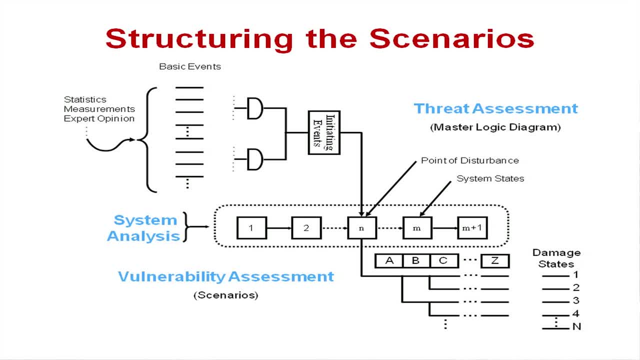 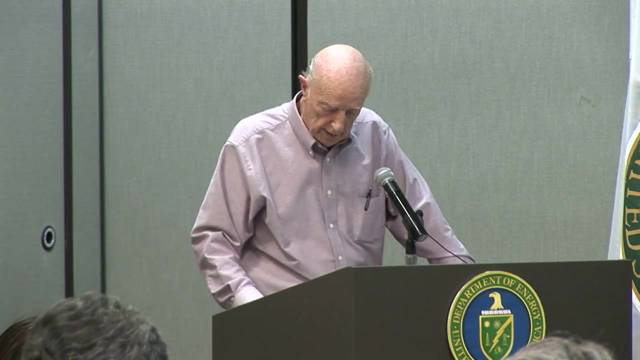 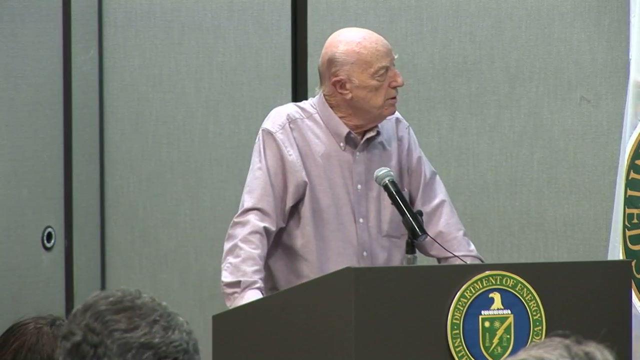 rates and so forth. it's whatever information seems to be relevant to leading to a threat to your system at any point along the sequence of the system. The most developed part of it in many respects is the vulnerability assessment. This is where now we have the initiating condition or the initiating event. but we know that that initiating event that the facility is usually designed to intervene with, the continued pathway of that initiating event and corrective actions are built into the system. The ABC, et cetera are the so-called intervening events or the top events, and you need to. 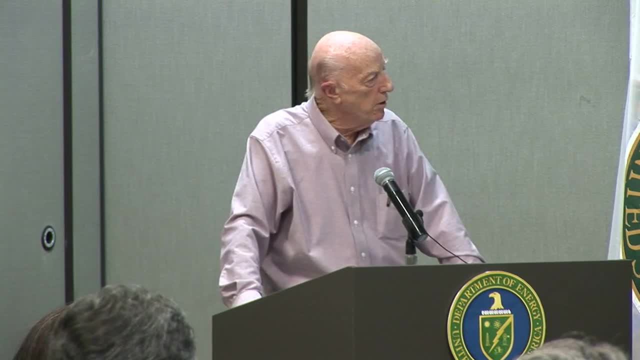 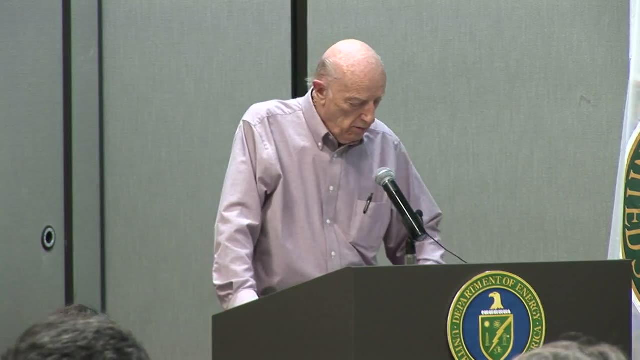 incorporate that into the system. You need to incorporate them in the whole structuring of the scenario process. So what kind of threats do we consider? Well, I think everybody's very familiar with that and I'm not going to spend much time on it. 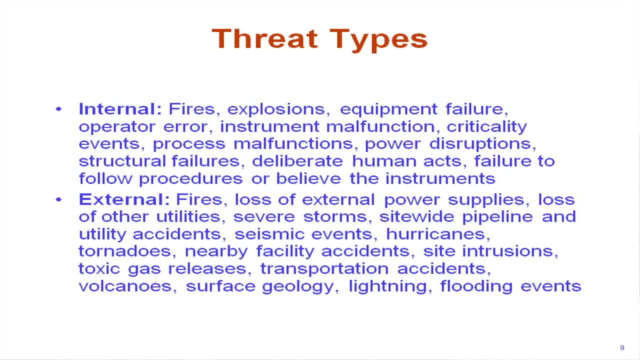 but there are two types of threats we worry about, and they are the internal, that is, the threats that come from the facility itself, and external. Some are common to both. You can have a fire internally initiated and you can have a fire externally. 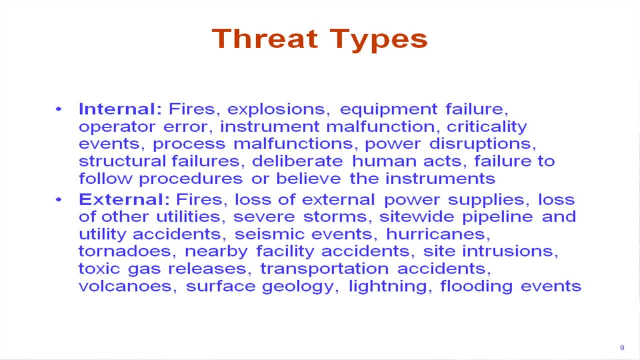 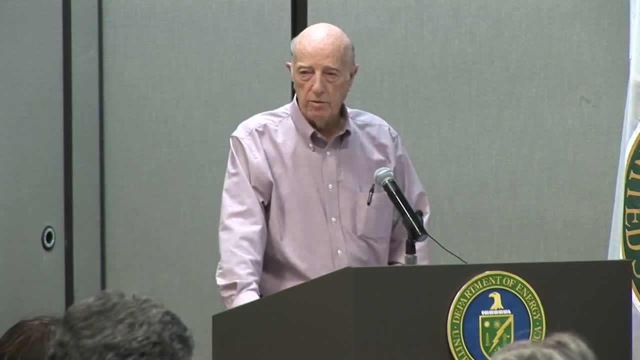 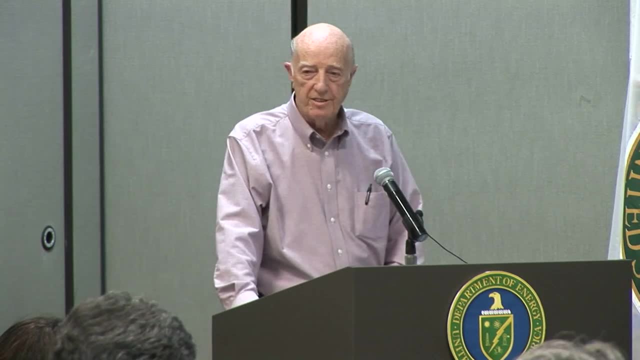 But these, you don't put limits on this, and every location, this list is different, And of course, you've got to also, as we have very much aware from the Fukushima event- worry about collateral events such as tsunamis from earthquakes and what have you. 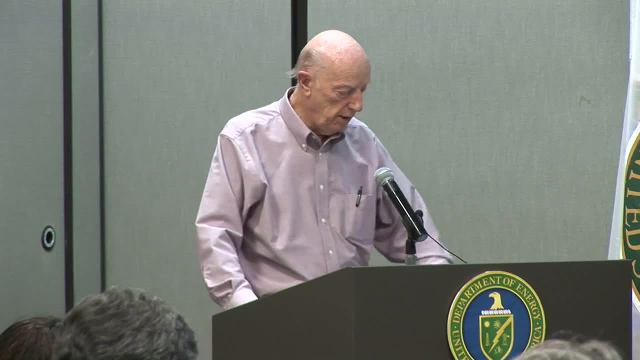 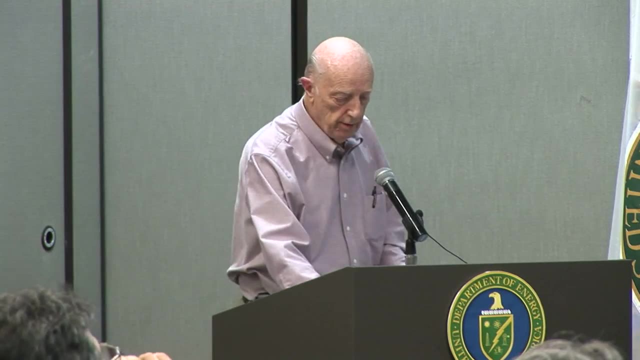 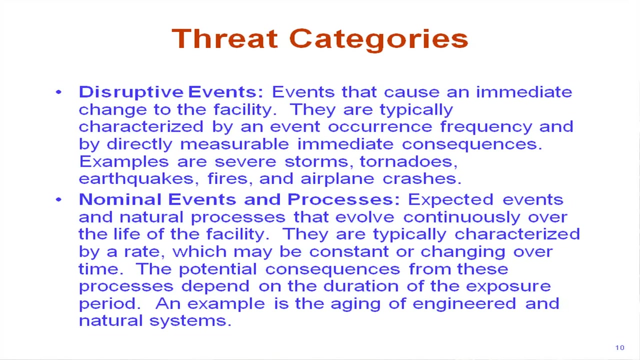 tsunamis from asteroid impacts is one of the big is a big issue on the coastal cities. Now we categorize these threats into two broad groups and this is. this was done extremely well in the Yucca Mountain Performance Assessment. 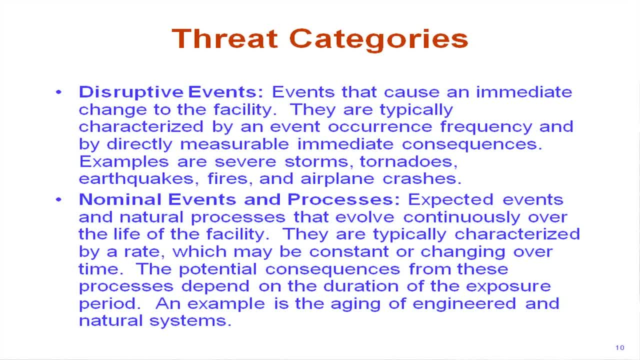 But we like to define disruptive events and nominal events and processes. Now, by disruptive, we mean something that happens that can cause a significant change with a very short time, constant, and that is the usual expected event, such as severe storms, tornadoes. 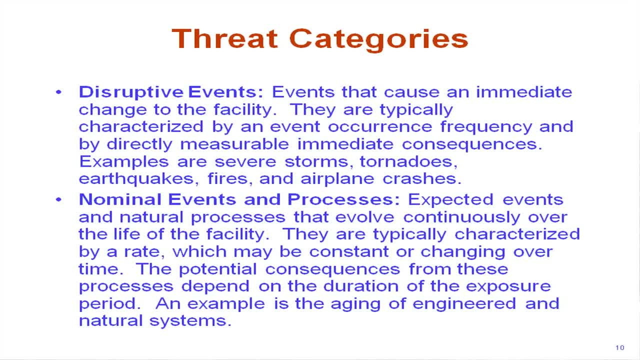 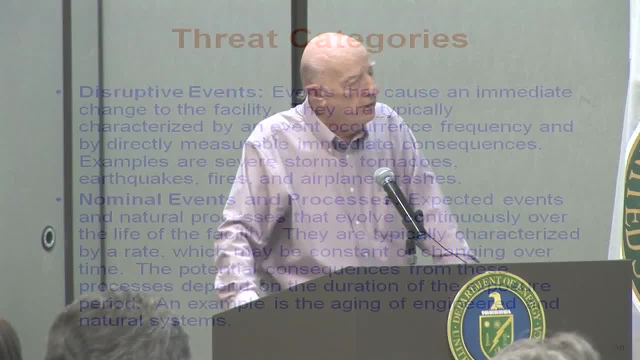 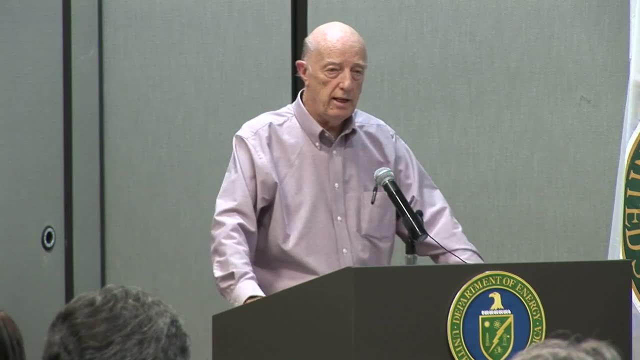 We just did a risk assessment of a radioactive waste disposal system in West Valley, New York, and it was quite amazing the number of things that that were unique to that site, and that's always the case whether you have a high-pressure gas line traveling through the site or whether it's. 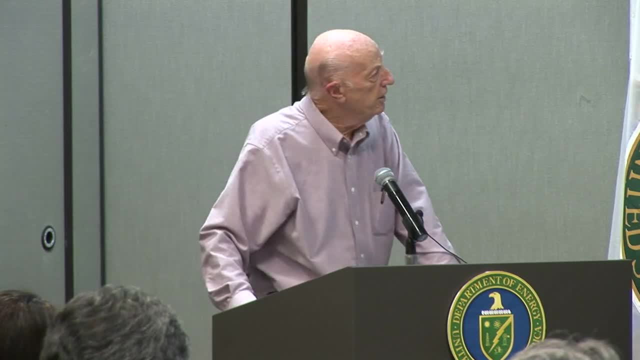 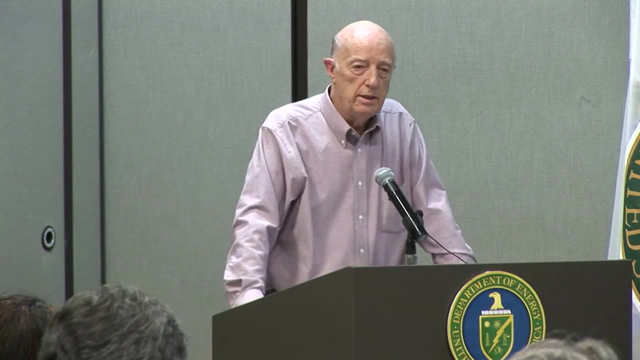 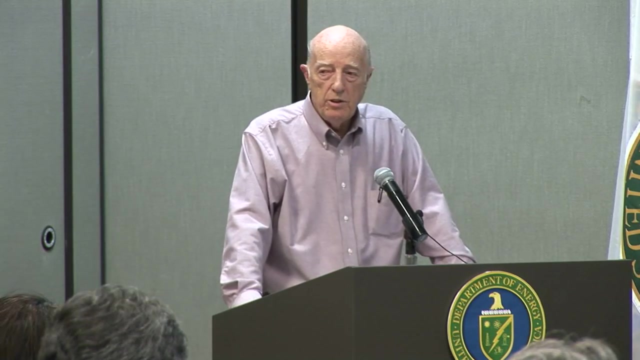 in the path, approach, pattern of a military base or what have you. Nominal events are kind of what you expect to happen with respect to the facility. These are usually aging effects, degradation effects, but very often you can develop a, an expression of that. 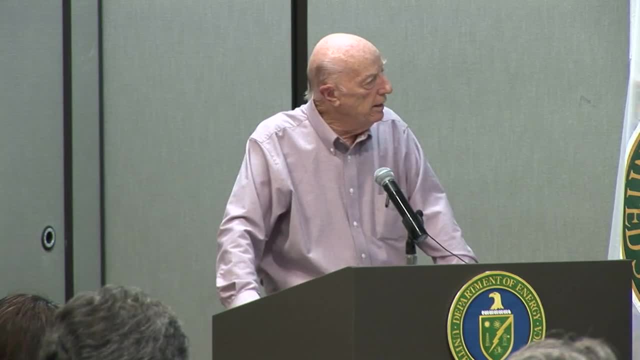 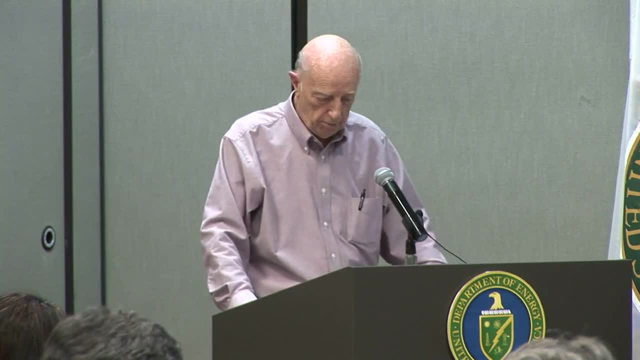 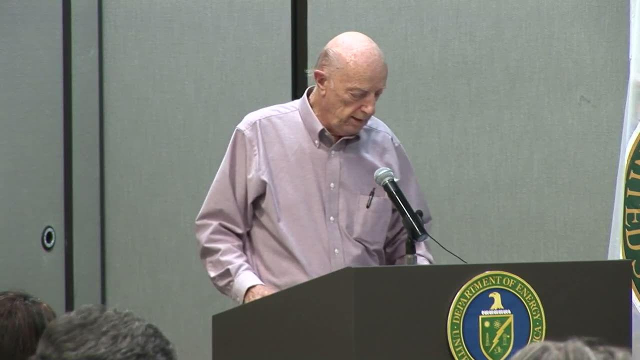 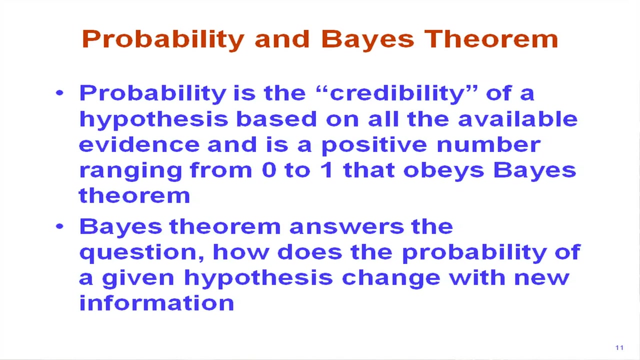 Sometimes it's constant and sometimes it's not. So what about probability? It's a very controversial topic, but in on the other hand, I don't understand why. Because it's it's it's: everything has a probability associated with them. 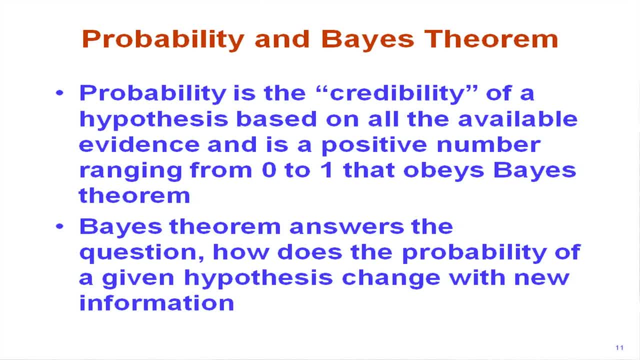 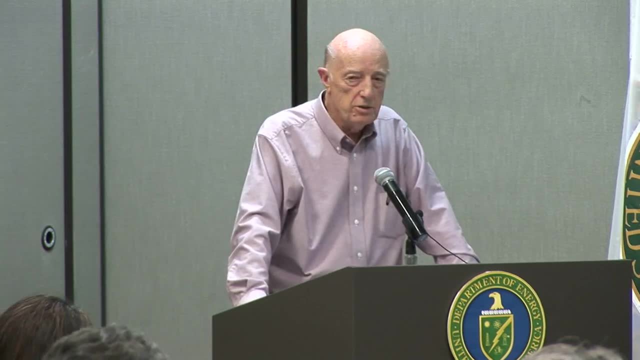 associated with it And, as I said earlier, what we took to be the meaning of probability was actually an extension of the famous professor at Stanford and Washington University, St Louis, Ed Jaynes, And in fact he's one of the reasons I got interested in this business. 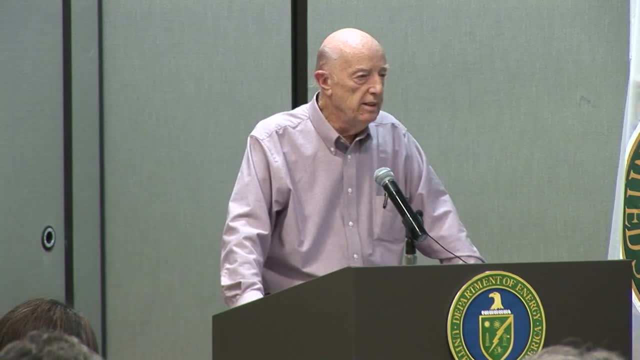 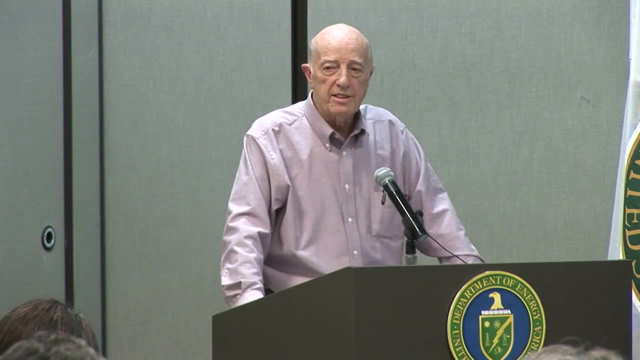 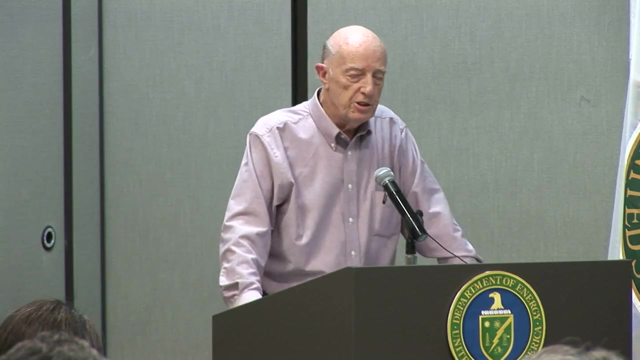 Is that my colleague and I, Stan Kaplan, attended a shark course at UCLA put on by Jaynes and Myron Tribus, And it was just a great experience because here was a genius with respect to the Boltzmann equation, which was the cornerstone of my early work. 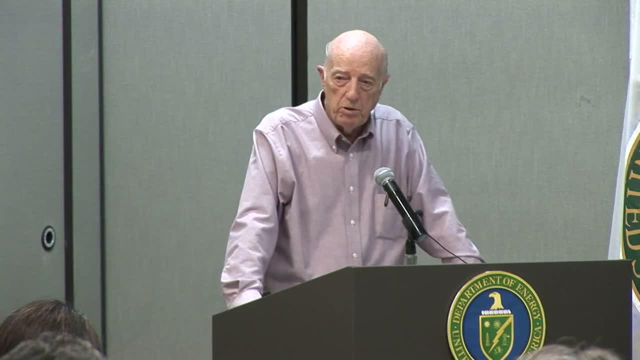 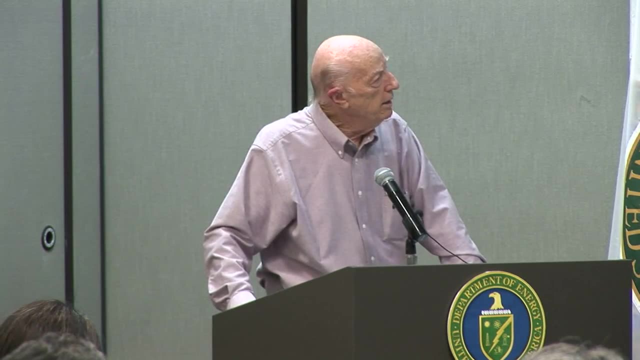 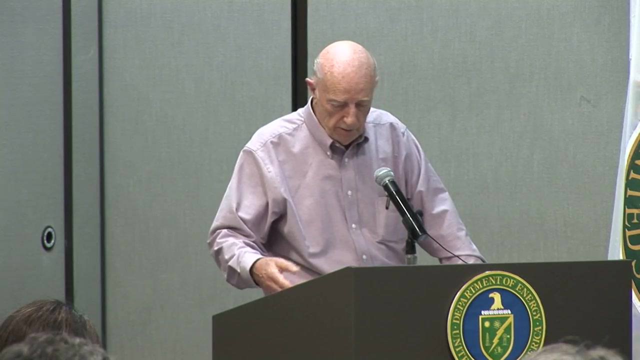 saying that most of the way people look at probability is not very productive, And he sparked really a long-term relationship and what I would say a major contribution to what we're now tabulating. Tabulating is a general theory of QRA or PRA And, by the way I 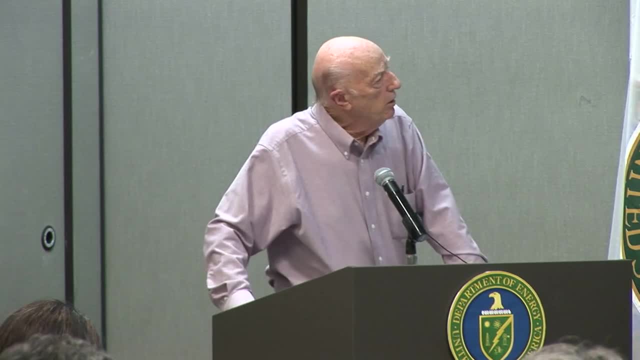 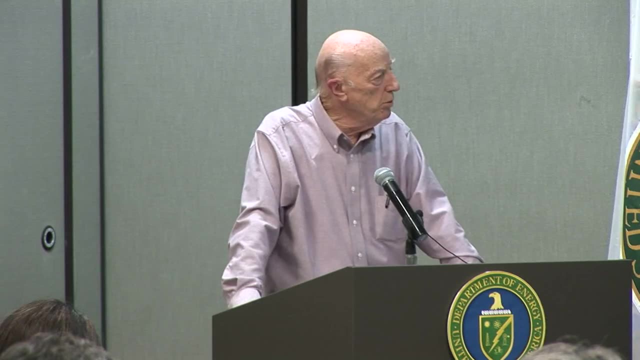 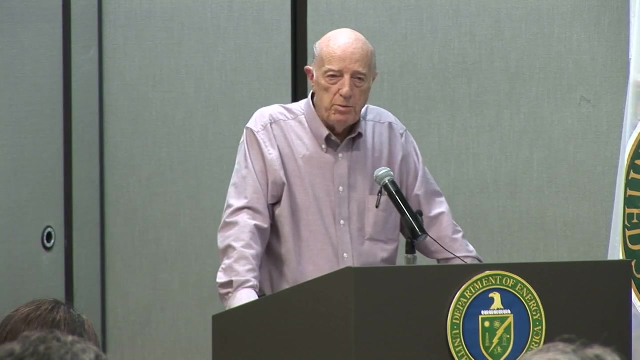 take QRA and PRA to be the same thing, Quantitative risk assessment and probabilistic risk assessment. Bayes' theorem answers the question: how does the probability of a given hypothesis change with new information? Very powerful, very simple theorem, One that can be derived in two steps, and probably one of the 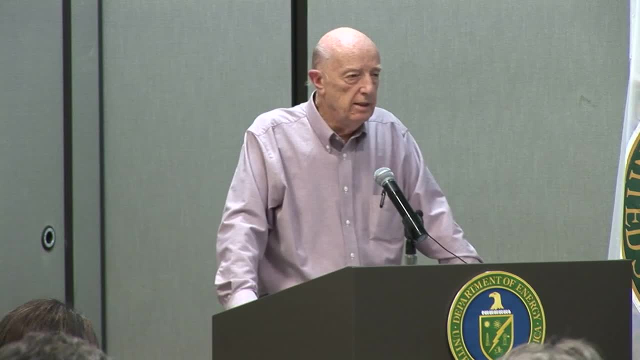 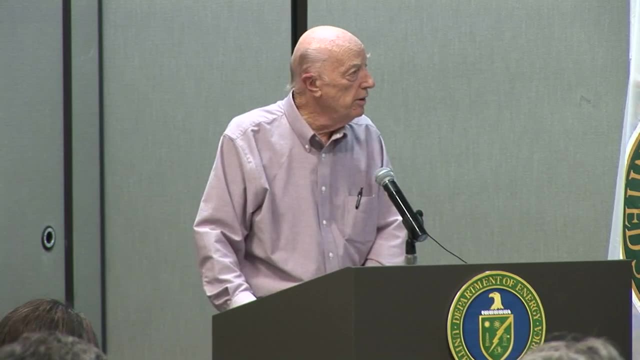 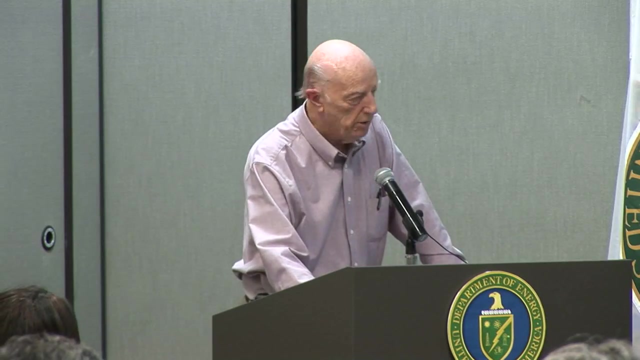 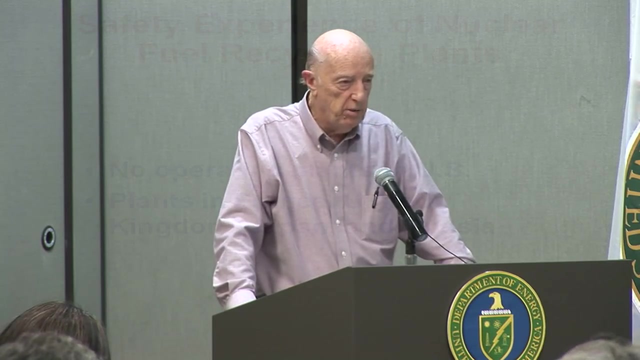 most profound probability theorems that exist, And it really is the cornerstone of any risk assessment that attempts to quantify uncertainties. Okay, that's all I'll say for the moment about the methodology. Let me talk a little bit about the safety experience of nuclear fuel recycling plants, And I'm not going to talk. 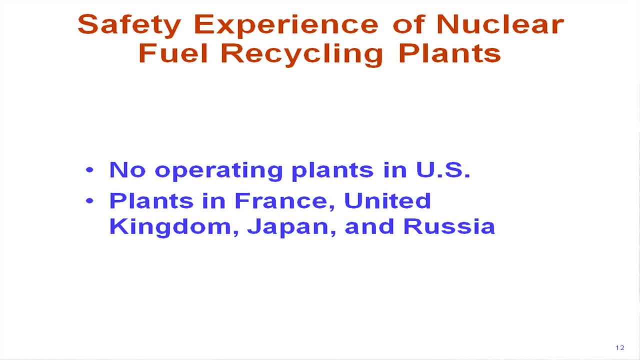 much about this, because you've had a pretty good dose of this in the last couple of days, But we know that there are no operating plants in the US, although there might be an argument that the H-Canyon at Savannah River is still doing. 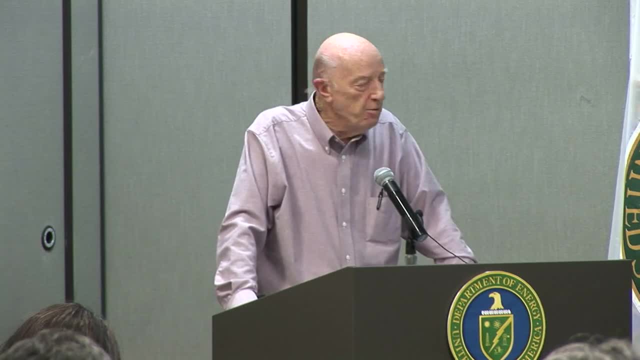 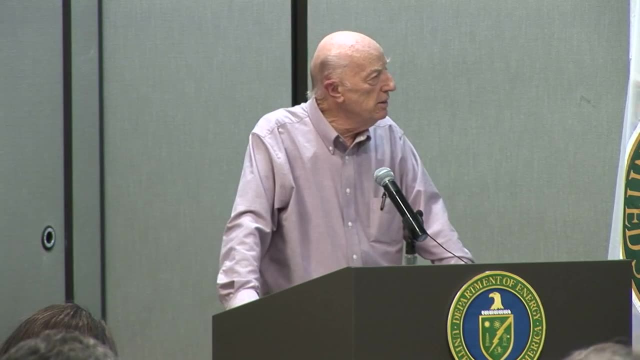 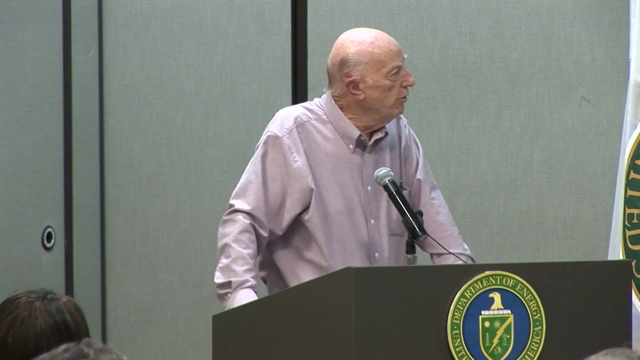 useful processing and let's hope it is and hope it continues. There are plants in France, United Kingdom, Japan and Russia. Many of them are having problems and issues and some of them are not even running right now. I guess the one that's 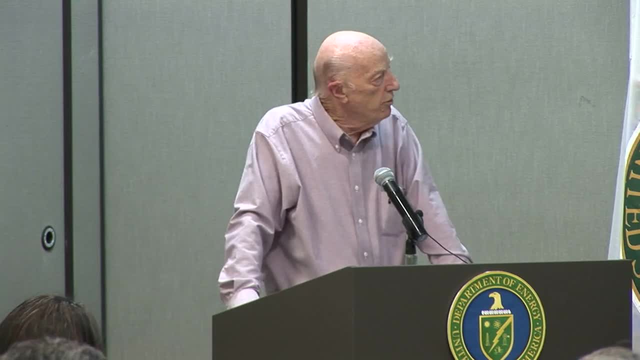 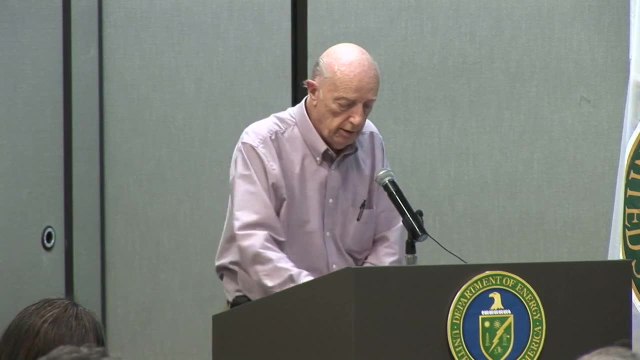 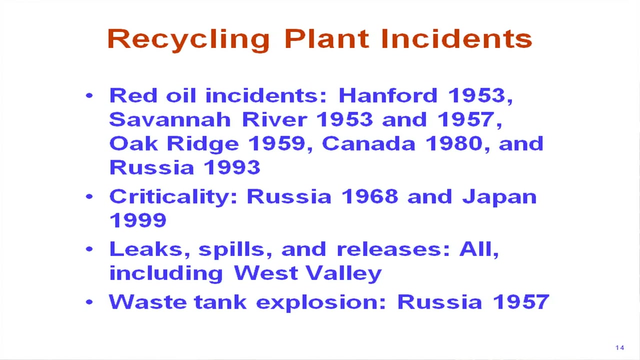 the most successful is in La Hague in France. Certainly it has by far the most experience And, as far as recycling plant incidents, is all of the plants, whether they're the government plants or the private plant in West Valley, are the plants in the UK and 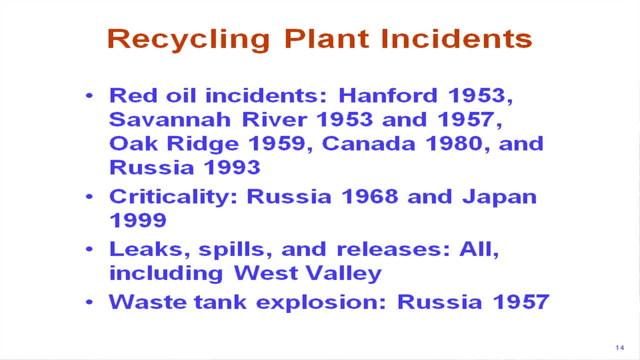 France and Japan, and there are some plants in India, but nobody seems to know much about those- At least I don't, and I couldn't get the kind of information that was needed to really make any kind of assessment of them. But all of the plants as 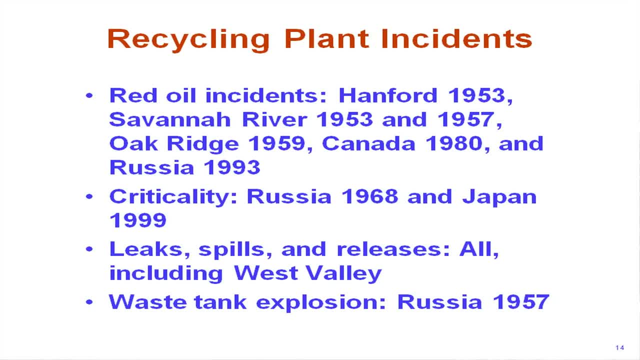 indicated in that third bullet experienced leaks and spills and releases and fires and resin fires and all kinds of little events. As far as I know, none of them were catastrophic. none of them resulted in fatalities. There's two outstanding criticality events, and one in Tomsk, Russia, and the other one in 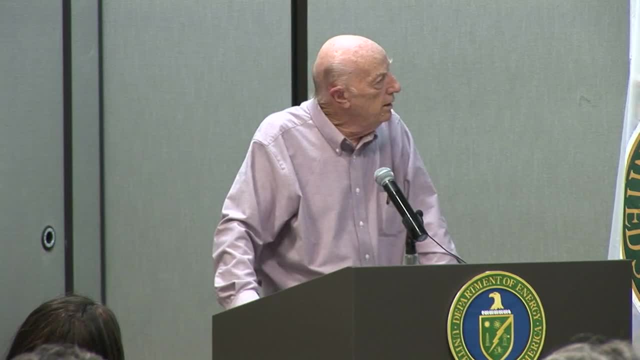 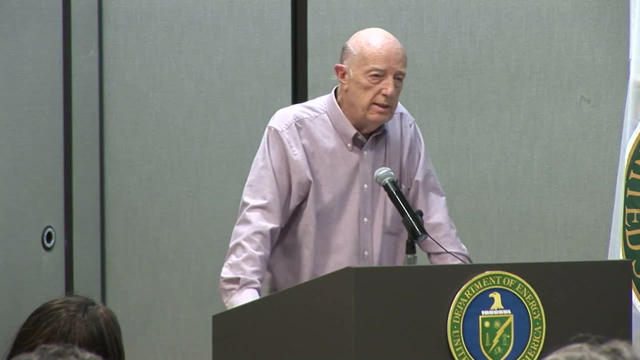 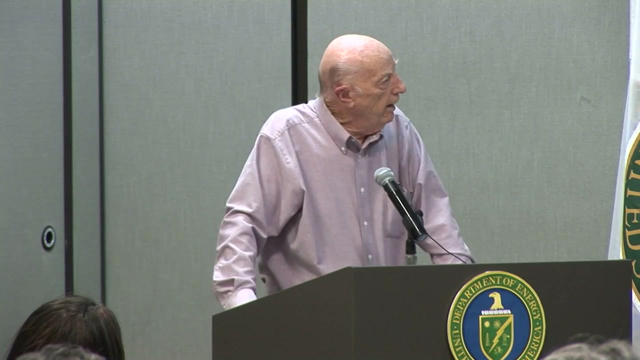 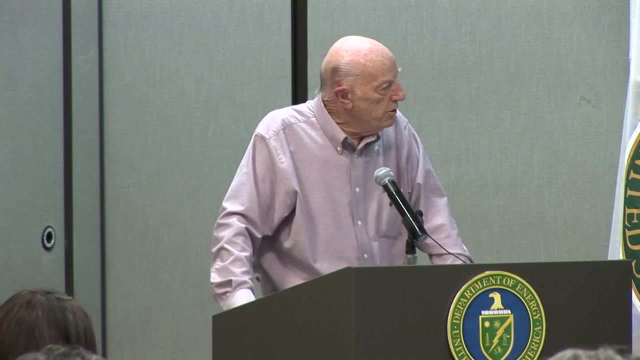 Tokimura, Japan, And they both involved the same mistake of moving safe, unsafe material from a safe geometry to an unsafe geometry. And in the case of Japan, there were two people killed in the in the accident, Perhaps the most devastating one. it was the waste tank explosion. 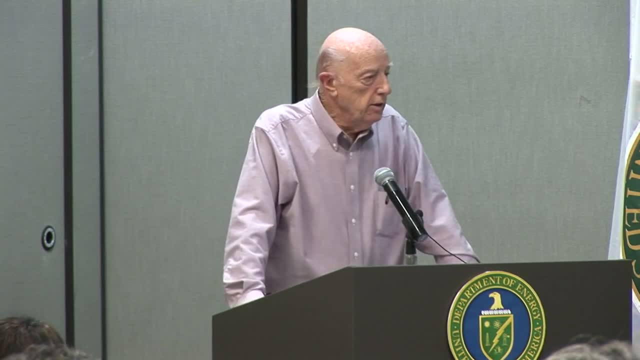 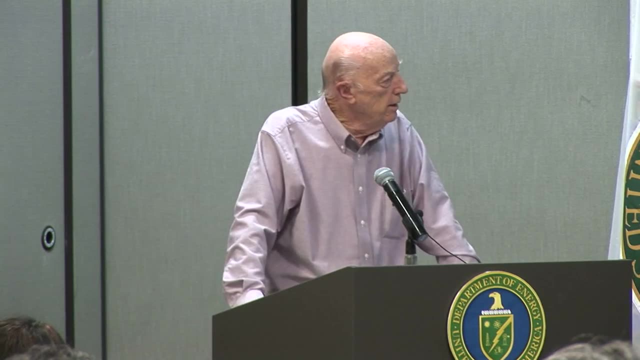 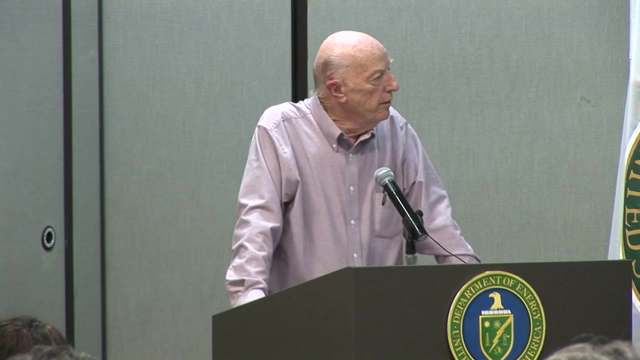 in Russia, And this was a case where the cooling system for the waste tank was not in operation. It was very high level waste, a lot of heat being generated, And it eventually dried itself out and it's basically ended up being ammonia nitrate and acetates and eventually 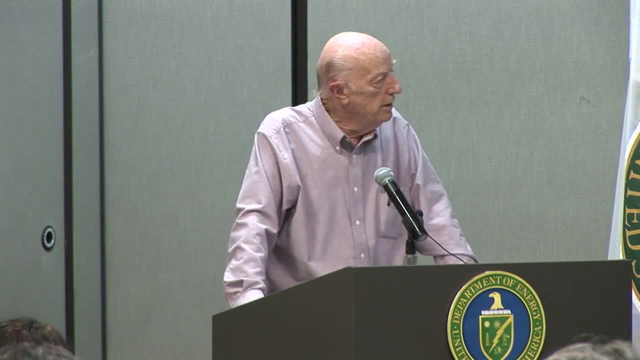 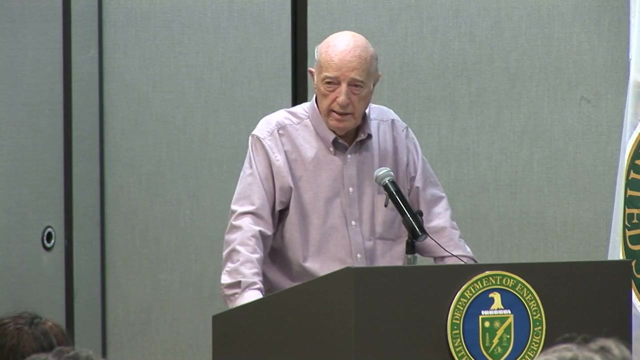 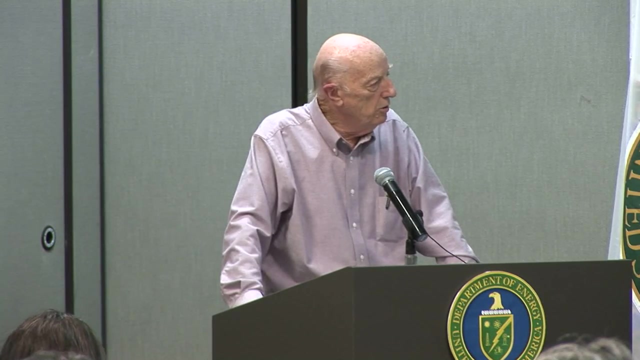 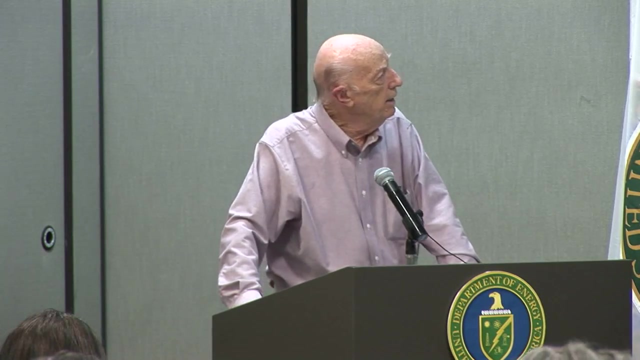 exploded And that explosion lifted the tank from a buried condition and caused what Some media reported as lots of fatalities, but they were latent fatalities. It's very fuzzy on just whether or not there was any acute fatalities, But in the nearby, the nearby communities did suffer from that event. 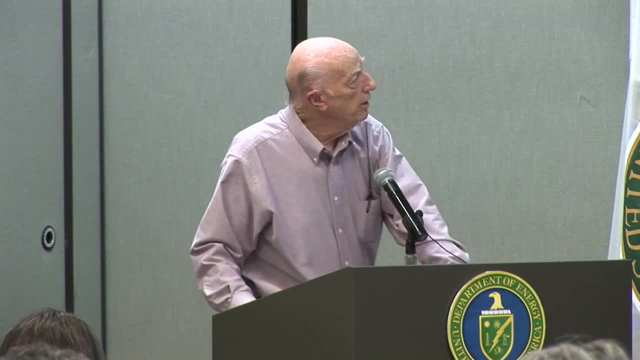 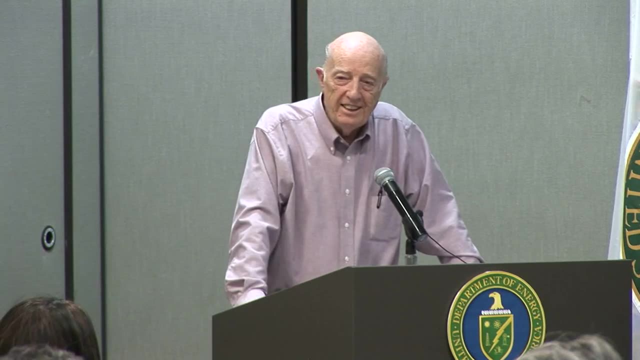 The most high profile event are the red oil incidents, And there were a lot of those. I don't think there would be in a new plant. I think that we'd be using deluents and other methods to keep the temperature and the pressure. 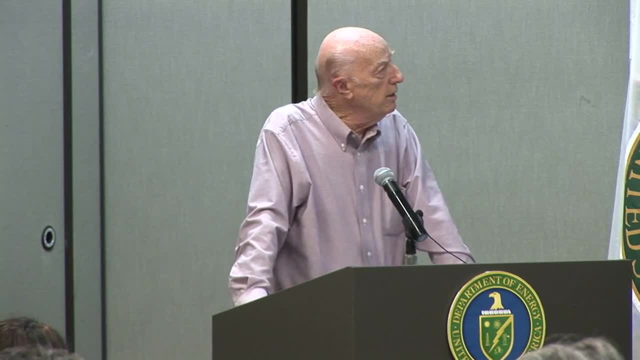 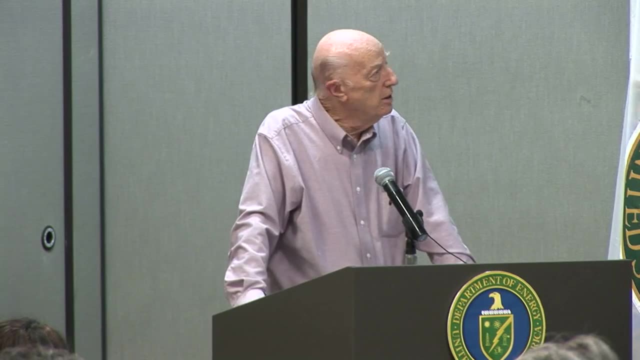 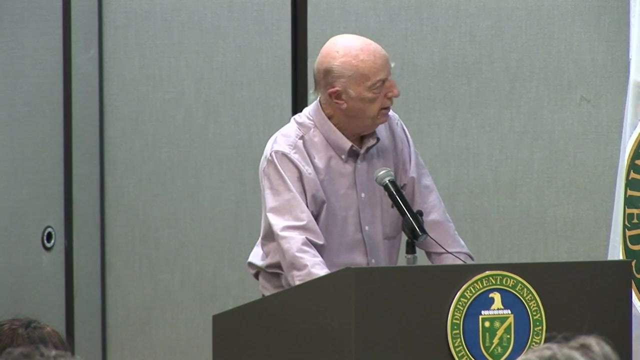 under control, But we had them at Hanford, Savannah River, two at Savannah River, Oak Ridge. we had one Canada and Russia, And so these are the main things that seem to seem to have happened in the reprocessing field. So let me go back to my original. 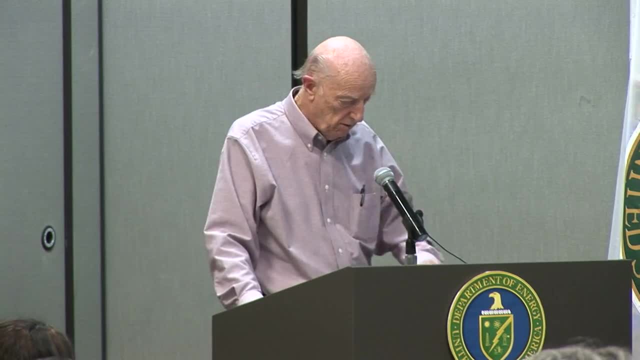 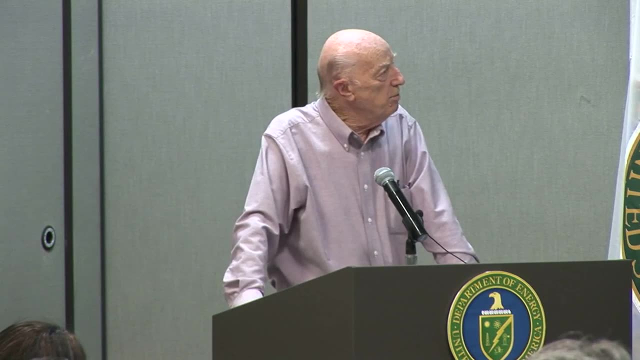 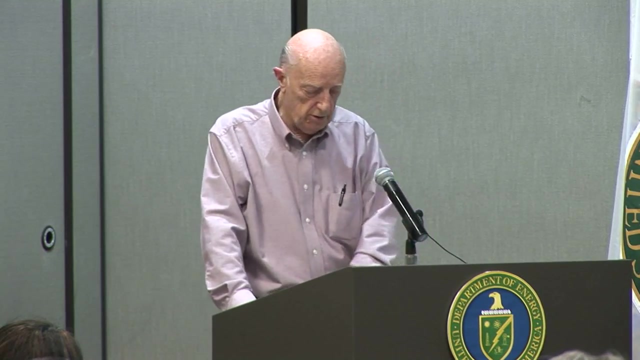 I'm sorry, This is my main job of telling you how you might address this on a system on a step-by-step basis. So this is the third part of my top. So the first thing we say you should do is define the system. 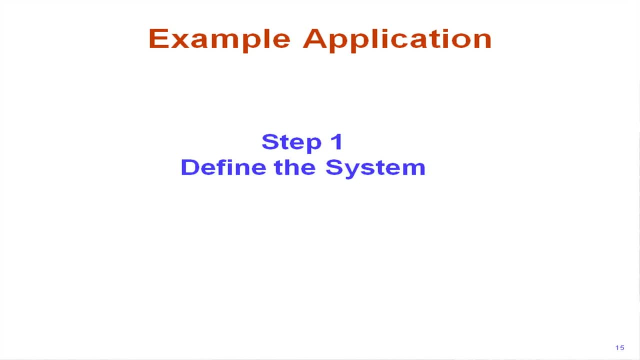 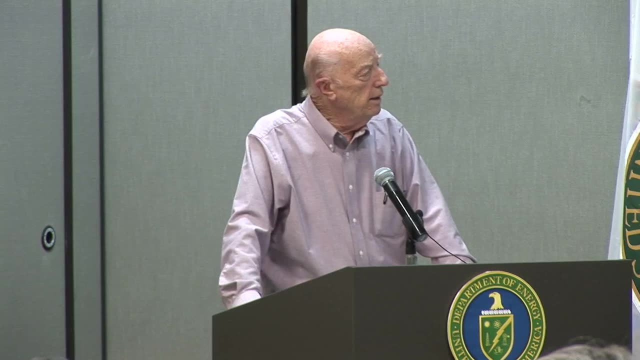 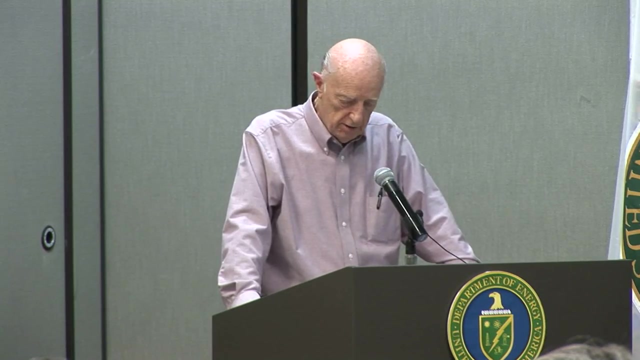 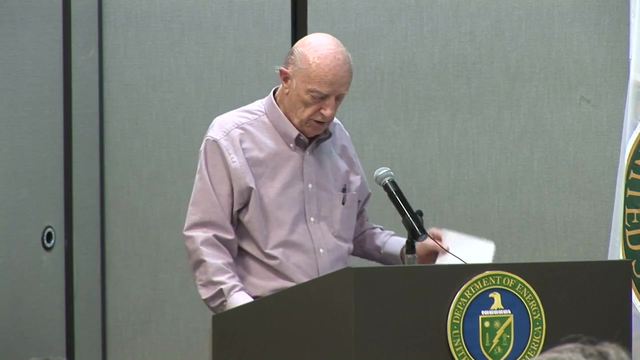 And we always spent maybe more time on this part than any other part, except in developing the scenarios. but unless you did this right, you weren't going to have much success in developing the scenarios. So how do you go about defining the system? Well, you do a lot of things. 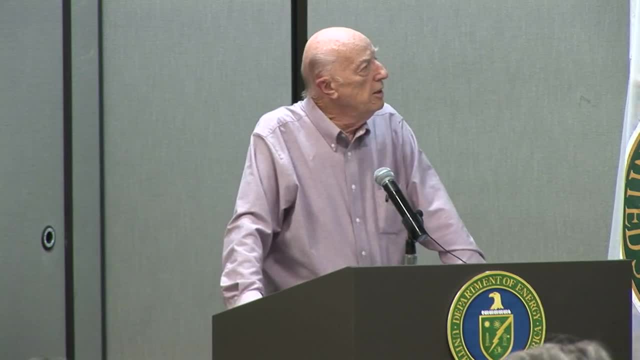 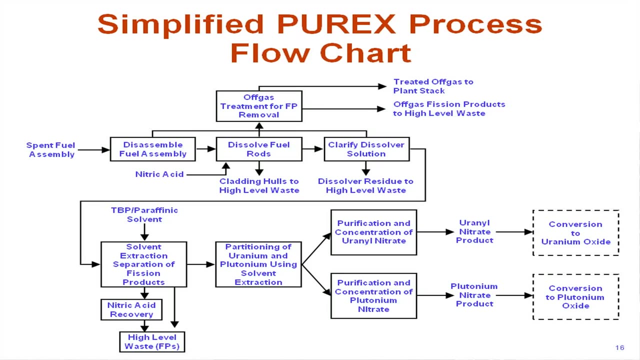 I'm not going to walk you through, for example, a typical pure explant flow sheet, because you've had that, I think Jubin Bob Jubin covered this the other day. But except to point out that process flow diagrams- 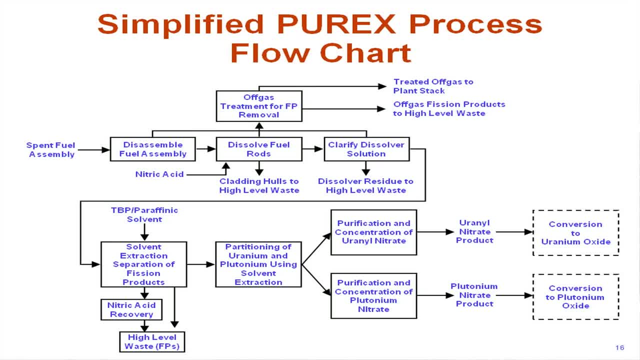 in a much greater detail than this are critically important to understanding the system, But there are other things that are just as important, And one of the things we found- that's probably the most important data source- was something we were denied in the early, early days. 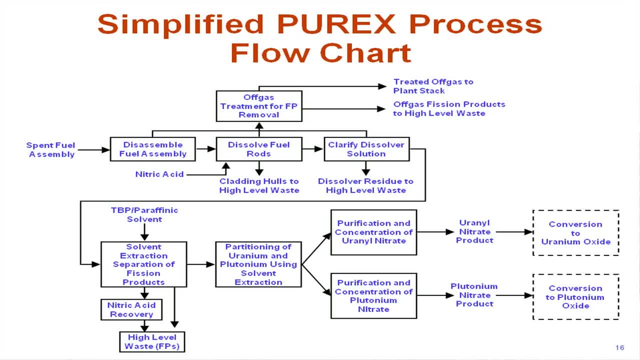 and that was maintenance Data is amazing what you can learn from the maintenance data about the performance of your plant. But maintenance data, or operating procedures, are absolutely critical And being able to think out of the box one of the things I learned as a director of a risk assessment team. 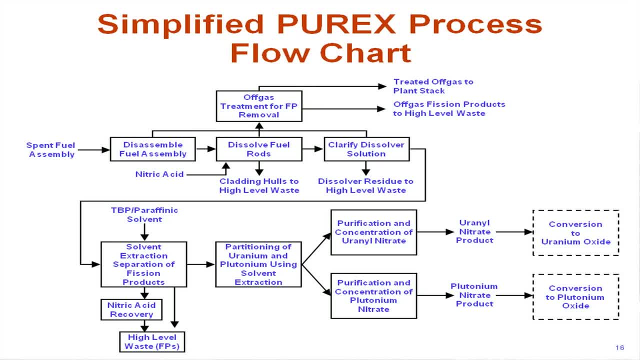 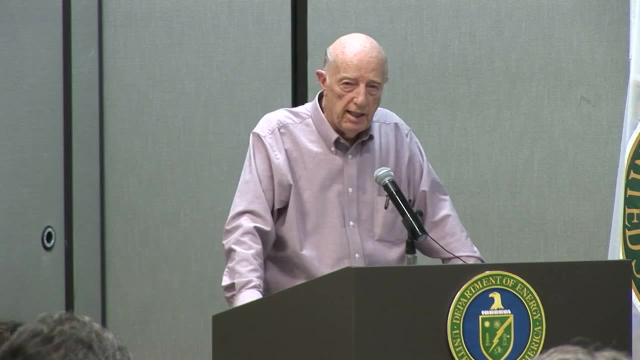 over two or three decades Was that you've got to think out of the box in the creation of the scenarios, And generally I didn't have much luck with people we hired that had a lot of licensing experience, Because they kept trying to think. 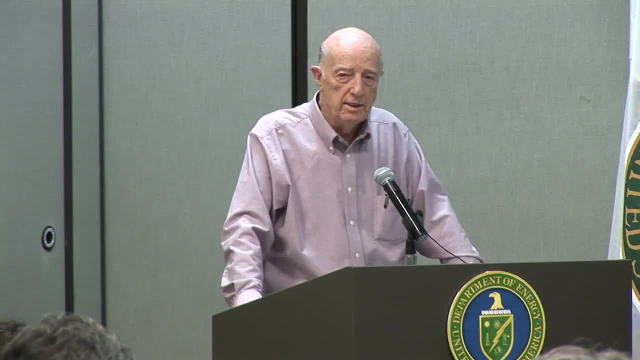 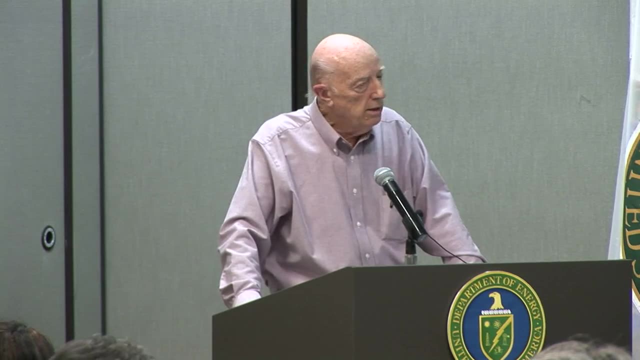 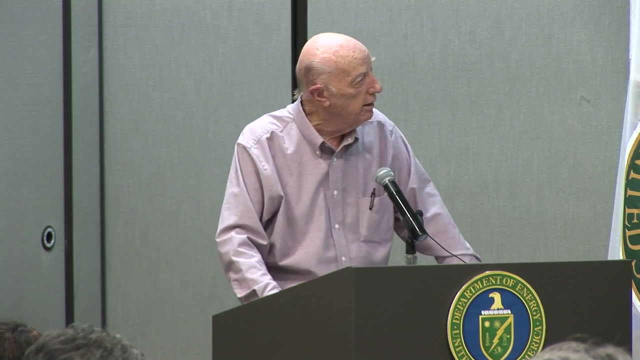 within the box of licensing And that's not what we wanted. And you really want to think as fundamentally as you can about what can go wrong with whatever it is you're analyzing And the other thing that we found that was critically important, that was not analyzed. 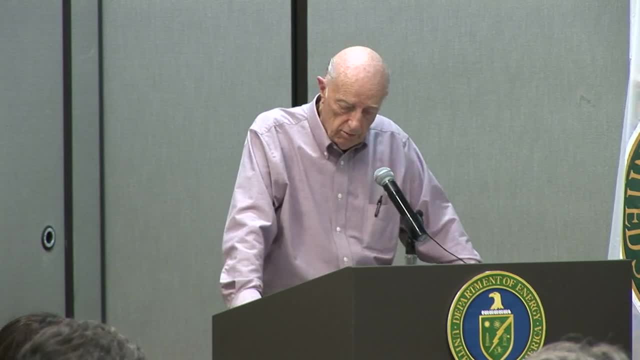 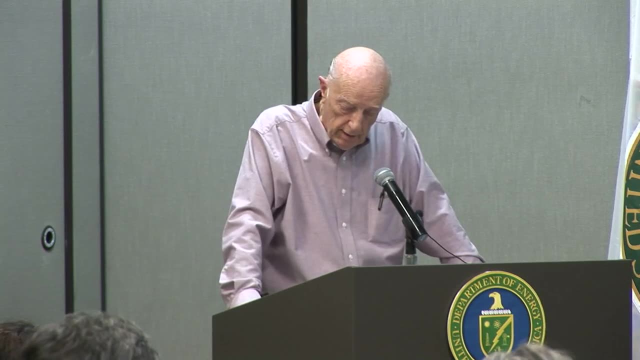 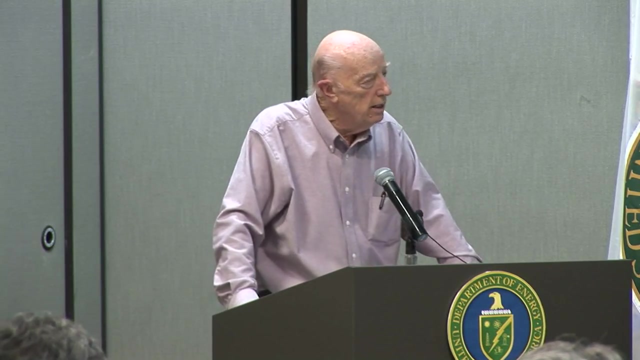 in a lot of detail in the early reactor days and that was support systems. And in the case of a reprocessing plant, you have a lot of support systems. You have off-gas systems, You have high-level waste systems, You have acid recovery systems. 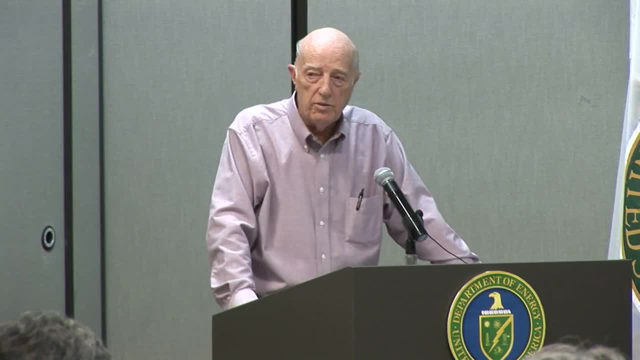 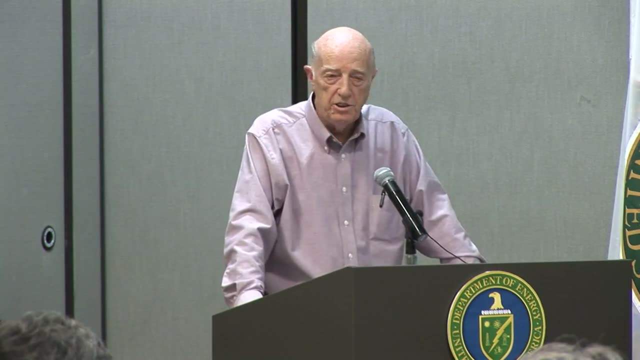 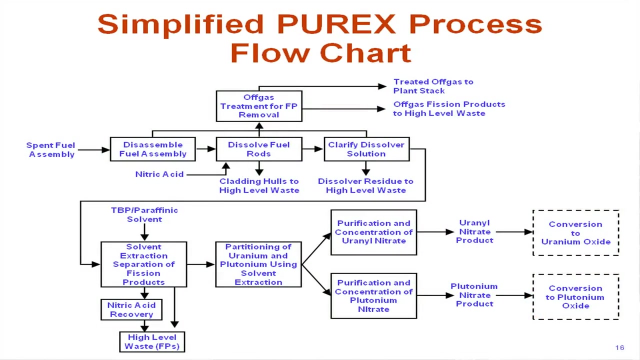 You have clean-up systems, You have solvent recovery systems And the usual process systems like instrument, air, steam, electricity and what have you And those. you really need to look in the dark corners of those to have any great comfort that you have been comprehensive in your analysis. 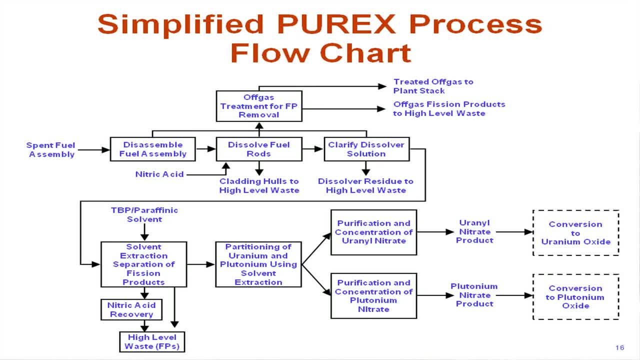 This was the biggest lesson learned, probably in the nuclear plants. In the nuclear plants, because everybody was kind of married to the design-based accident concept, the guillotine brake concept, And so what led to Three Mile Island? A simple relief valve and not good knowledge. 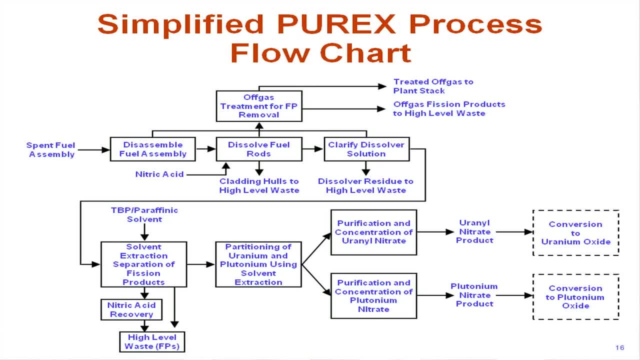 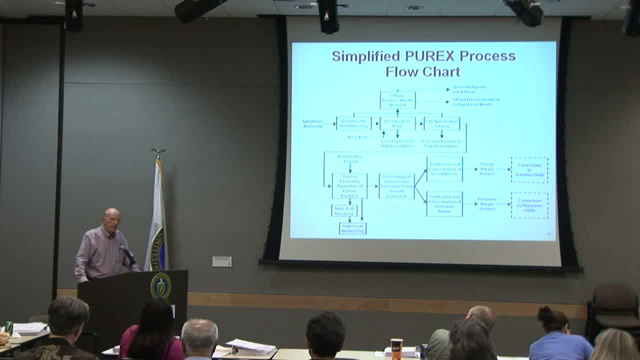 about the disposition of that relief valve at all times and the support systems. What led to a lot of other accidents was the failure of the chilled water system in the satellite, The idea that it was one of those systems that you could do the reactor on your own. 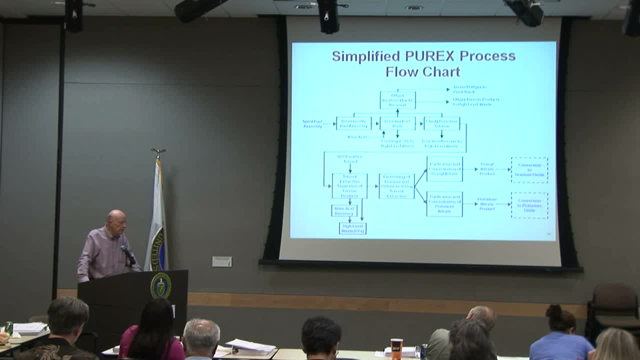 and that you could do that without having to go through separate and independent changes, A system that you can go back to the early reactor safety studies and you'll see it never mentioned. So these are the things that can trigger, things that can cascade. 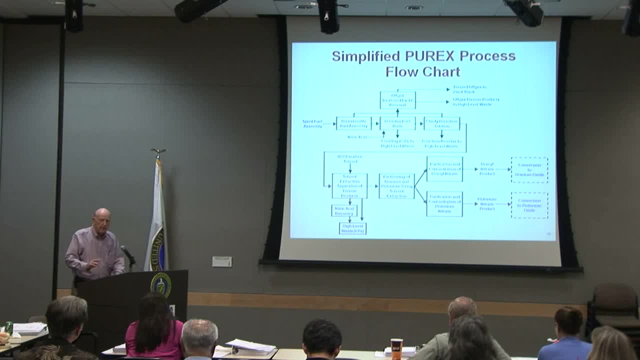 And that's why the scenario thought process is so valuable. One thing I forgot to mention: I said I was not any of the disciplines that seemed to be relevant to reprocessing. maybe short change there. I had an experience with reprocessing that I don't think anybody in this room. 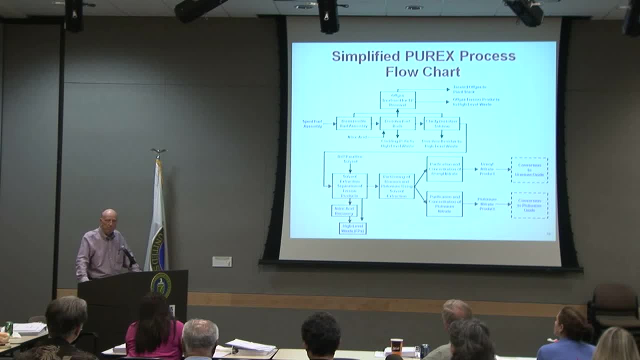 had, And I was on the startup team, and now I'm revealing my age. I was on the startup team for the Idaho Chemical Reprocessing Plant, But I wasn't hired for process work. I was hired to worry about the physics problems associated with that. 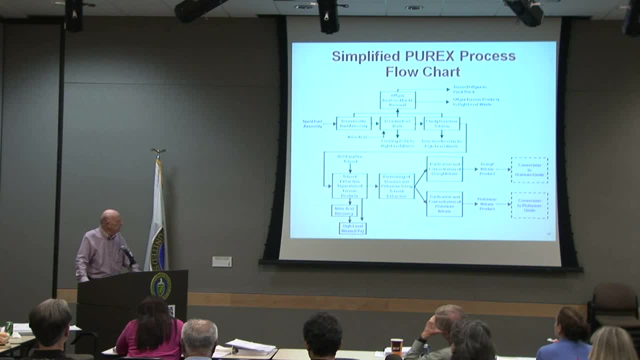 plant and namely mostly criticality. And it was the first. we put together the first criticality team for the site and we not only had the criticality concerns about the plant, the chemical plant, but the reactors, and we even interacted with the Navy people. 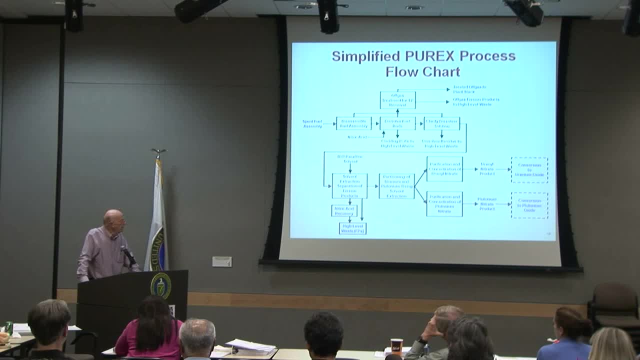 and certainly the EBR people. It was an exciting time because everything we did was the first time And when we put the product of the plant through its first paces, from a radioactive standpoint, it turned out that the product was hotter than hell. 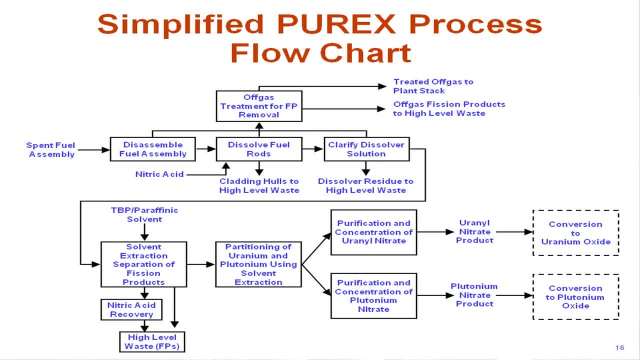 And what do we do about that? Because nothing seemed to come out the way it was supposed to. Well, they put together a team of about six of us and said: fix it. And I don't think this is what you could do today. 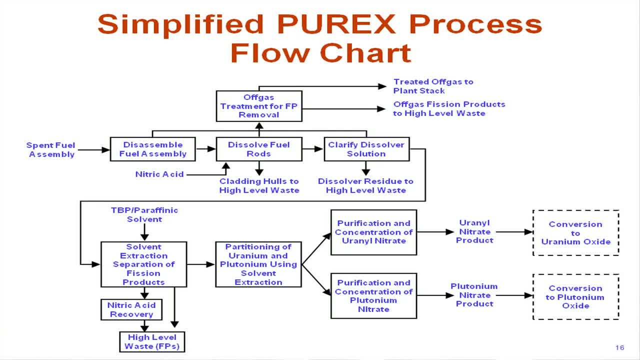 So we kind of slept with this system. So we kind of slept with this system For about 12 weeks. first we had to develop what the culprit was. I think Ray will know what that is. We discovered that for some reason or another. 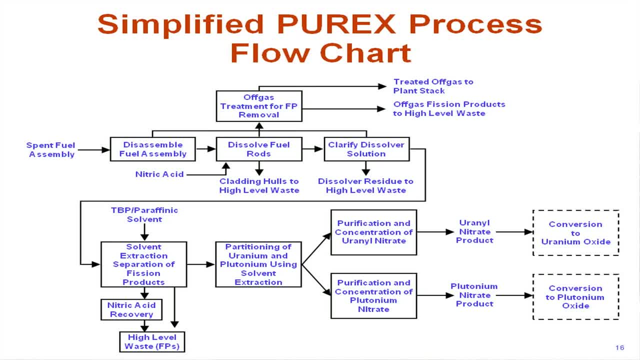 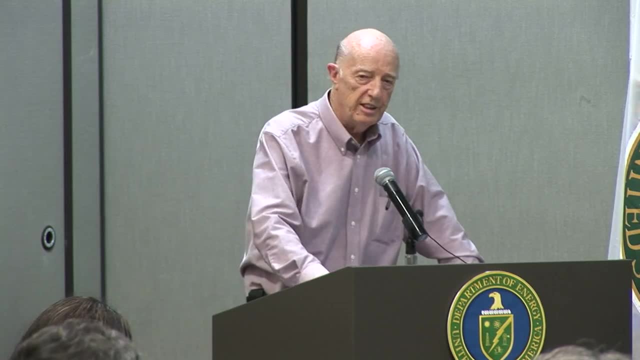 we weren't scrubbing out a couple of the key fission products, one of which was ruthenium- ruthenium 106. And so we simultaneously were doing distribution coefficient studies and height of transfer unit studies and all these kinds of things. 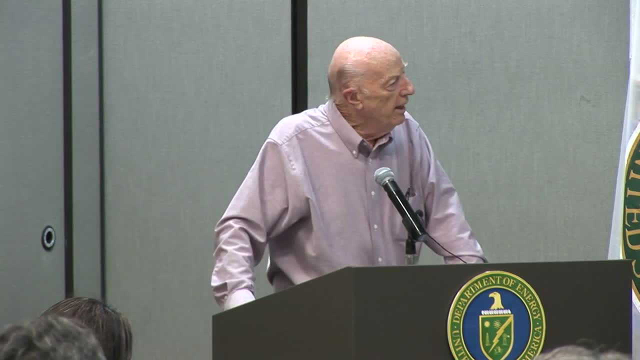 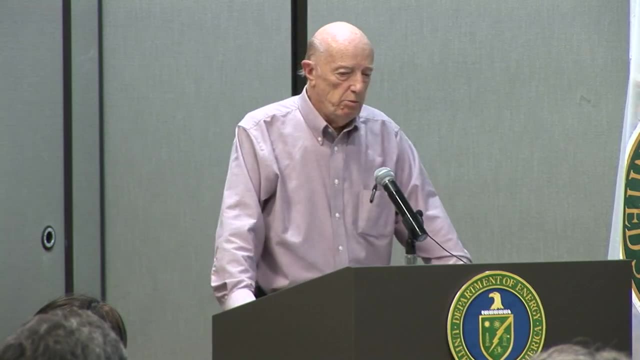 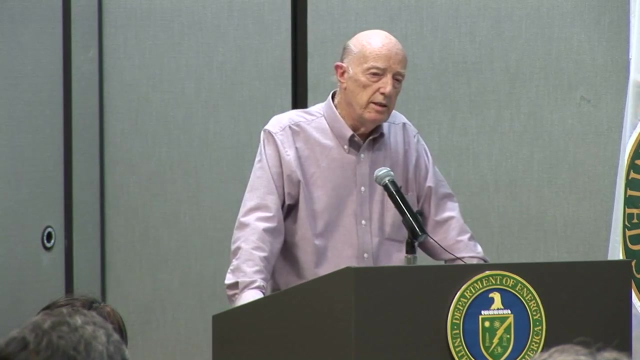 all these chemical engineering exercises that I was learning as a very, very young and green scientist. But we did put a team together that came up with a tail-end process based on precipitating out the ruthenium with an H2S-based process, although we had to use a cupric ion to make. 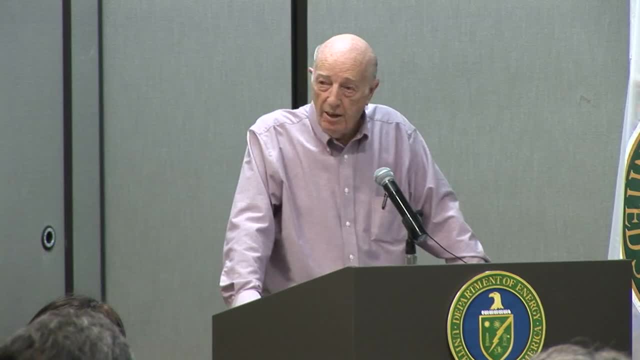 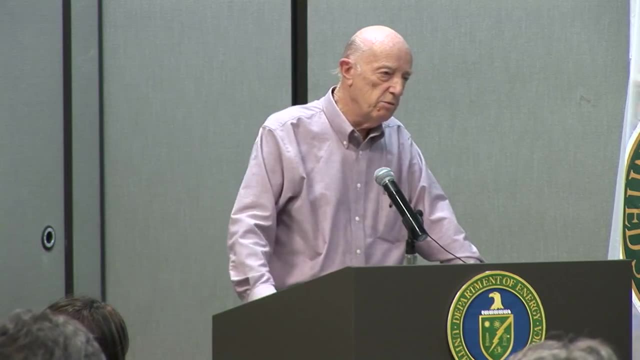 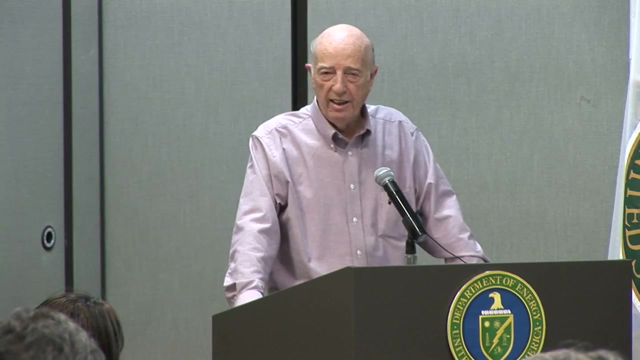 sure that the precipitation actually took place And we cleaned up the product And we developed, designed, built and processed that product in a period of about seven weeks And that was a great, great experience And we don't see a whole lot of that kind of activity these days. 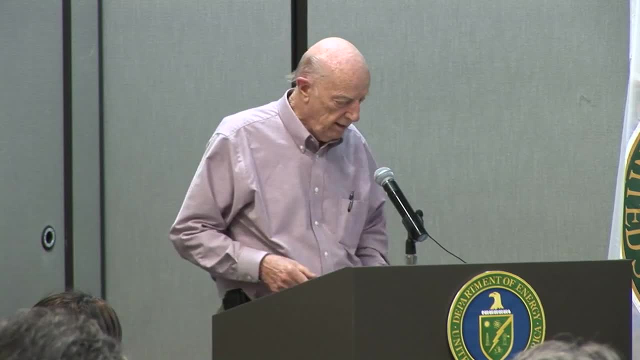 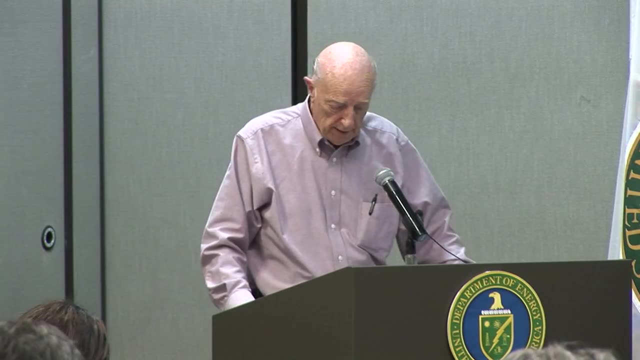 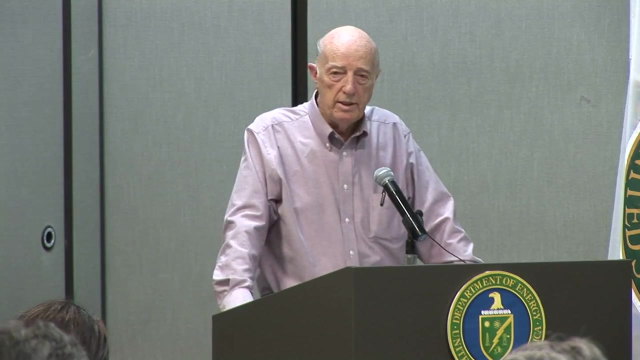 But anyway, this is just to tell you, when you design, when you're trying to define the plant, That you really need to spend the time that's necessary to do it, And in most cases our risk assessments were pretty expensive as a result of that. 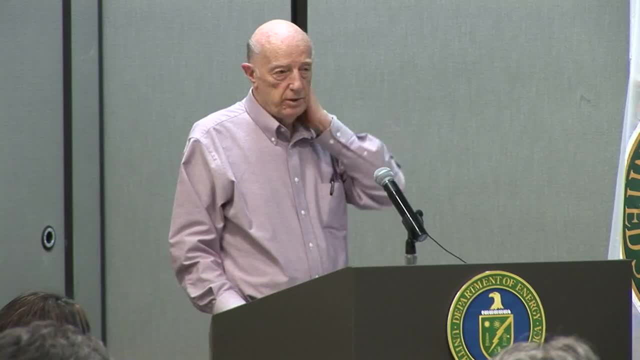 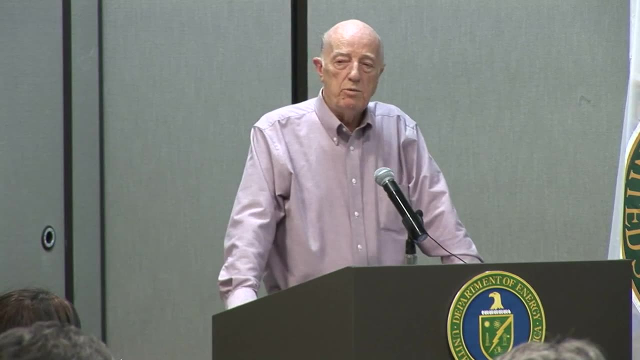 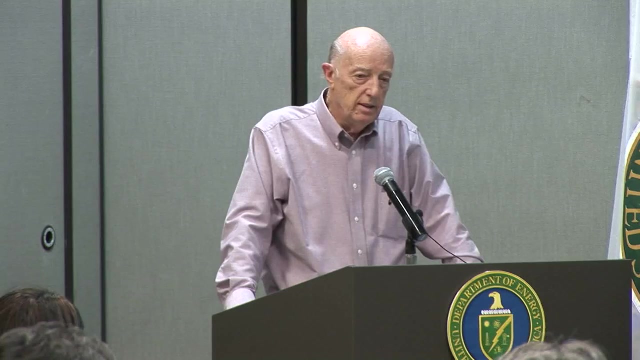 I remember meeting with the CEO of Pacific Gas and Electric. He says: we want you to do a PRA of Diablo Canyon, but we don't want you to bother any of our staff. And I said: well, I don't want to bother any of our staff. 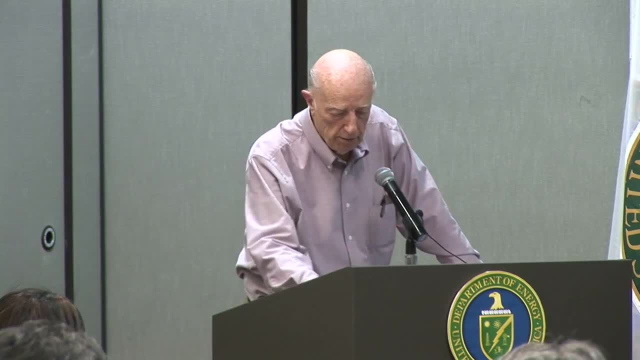 And he said: we want you to do a PRA of Diablo Canyon, but we don't want you to bother any of our staff. I mean, I wish he had the guts to stand up and say: well, and you don't want us. 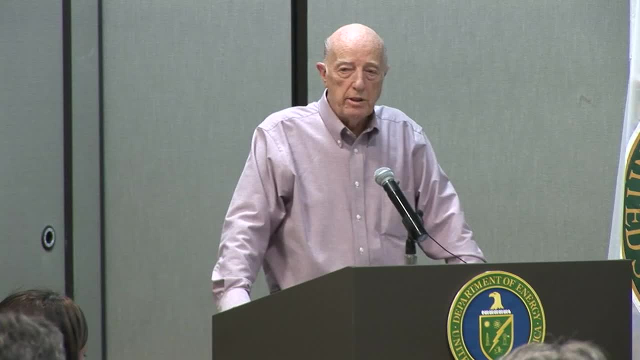 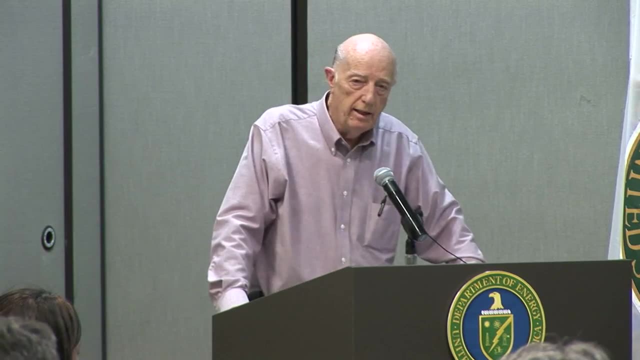 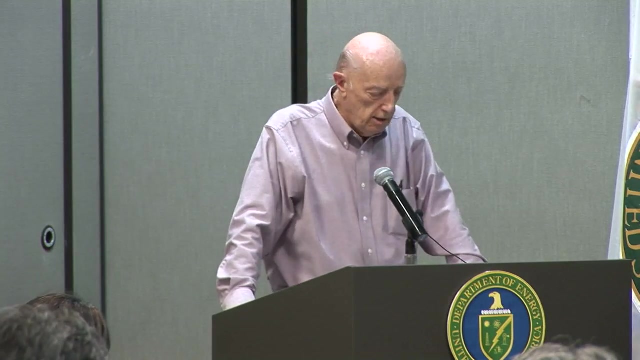 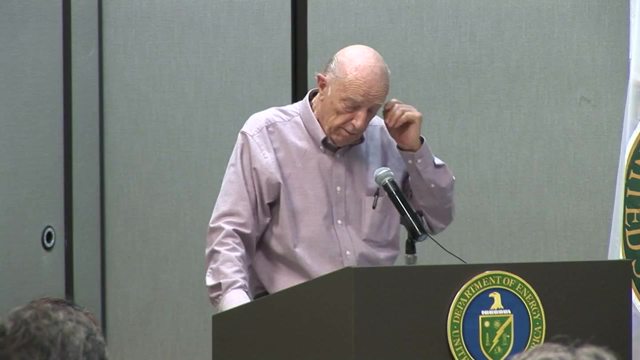 We have to involve the senior reactor operators in the process. They know the plant better than anybody And, just like NASA, they asked us to do a special study on the space shuttle And later on, on the space station. I kept getting these presentations from people and I said: 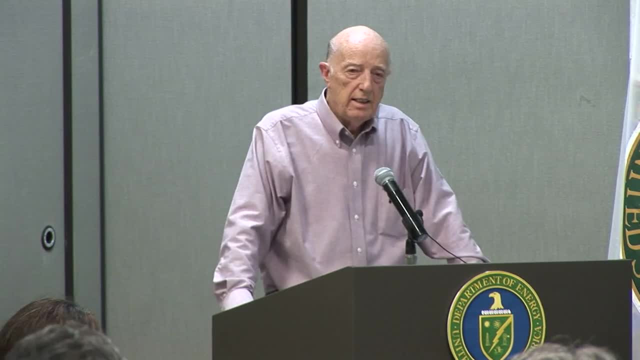 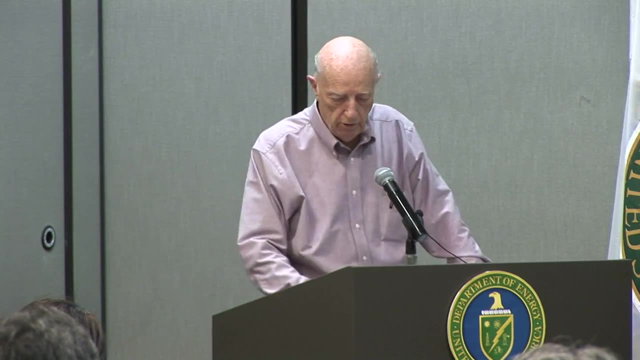 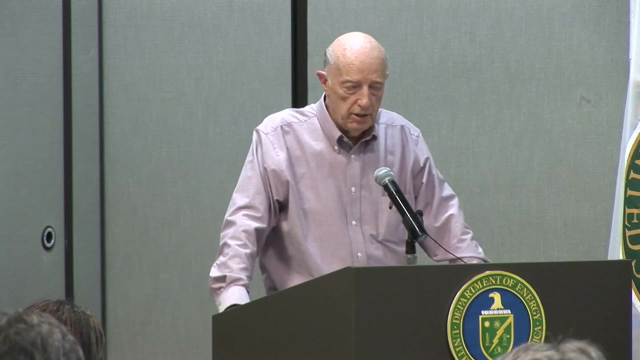 how come I don't see more emphasis on the scenarios of what can go wrong? And they said, oh, that's somebody else's problem. And so they invited me to attend a training session of the astronauts. and here they were going all through these scenarios. 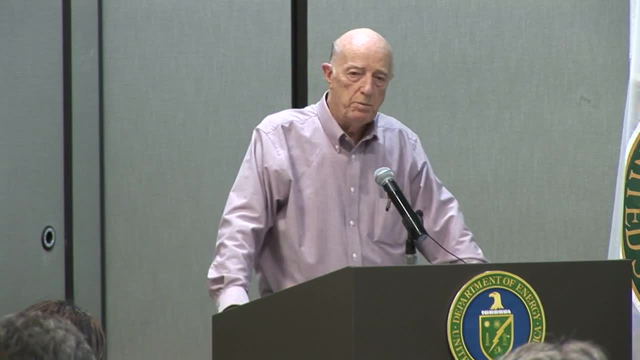 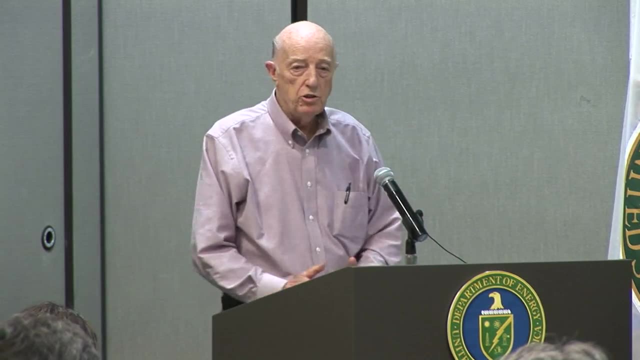 This is what structure can do for you in terms of being an obstacle. And I went back to the safety people. I said: why aren't you doing what they're doing? Why aren't you analyzing each of those scenarios? They said, well, that's not our. what was the word? 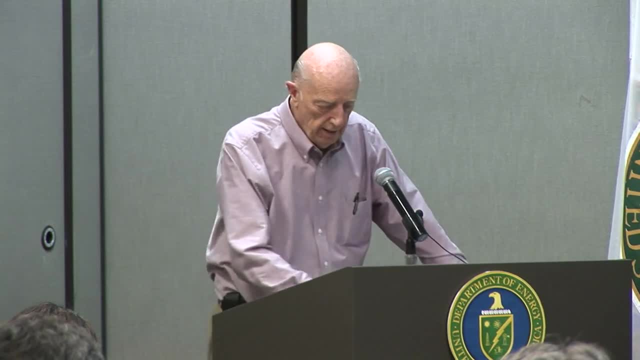 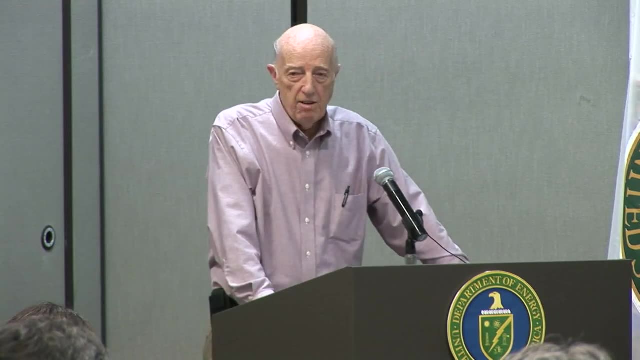 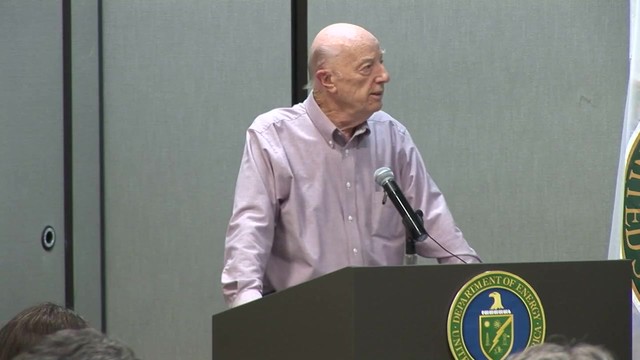 It's not our requirement, It was some such thing. So, anyway, I switched from working with the safety people to working with the astronauts, And that was a great experience because they thought the way we were. they were thinking in terms of the shuttle and how it could perform. 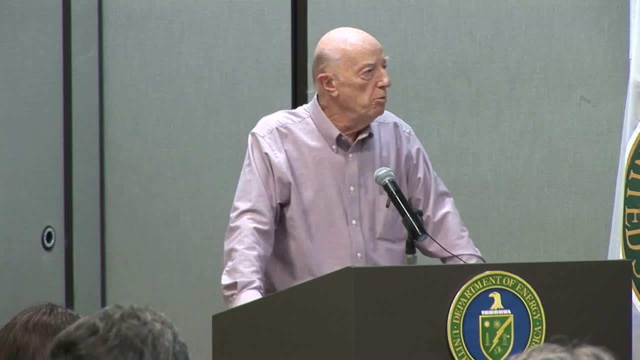 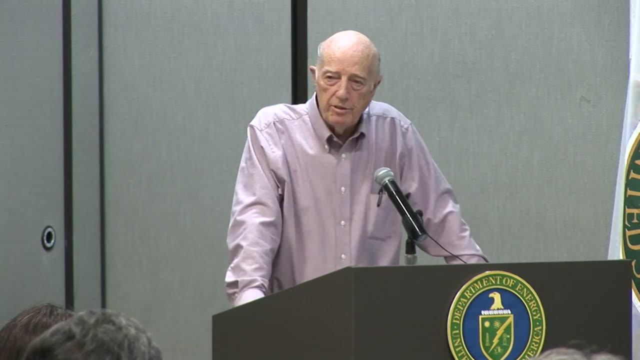 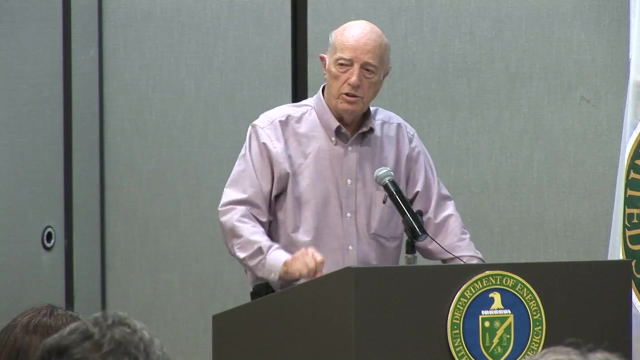 We were looking particularly at the auxiliary power units, because the auxiliary power units in the space shuttle are not auxiliary at all. They are absolutely essential. You have to have them for every operation on the shuttle, from thrusting the main engine to all the control surfaces. 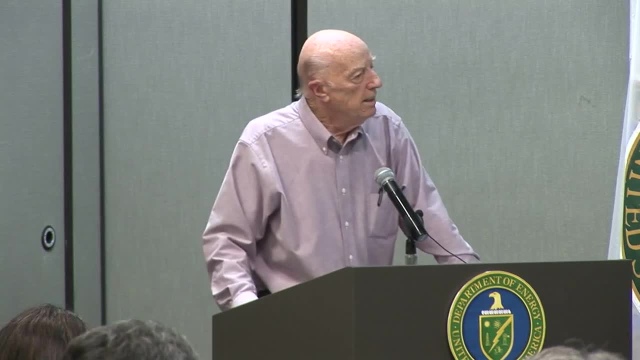 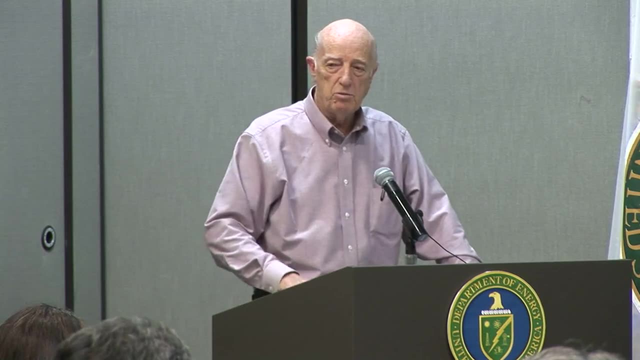 to deploying the landing gear to you name it. So that became pretty exciting because our little team would be working on a scenario We'd call up and we now had some actual scenario or astronaut contact And they'd say, oh, I need more flying time. 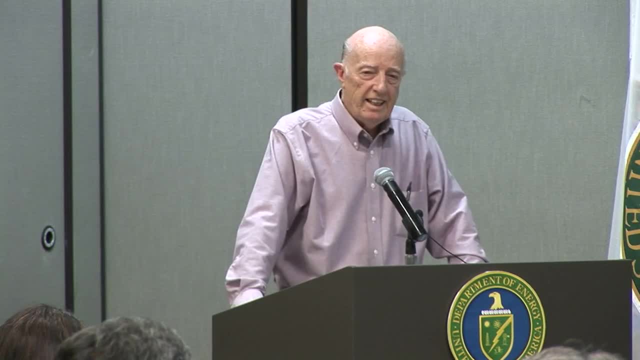 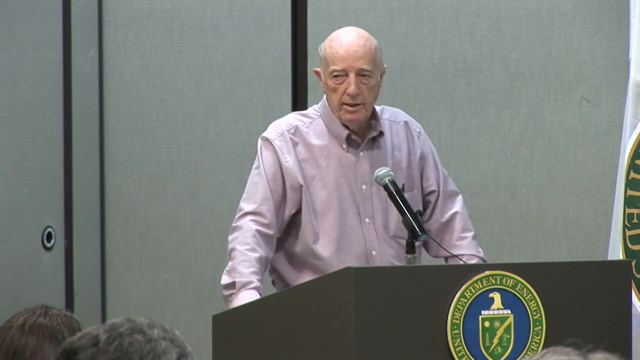 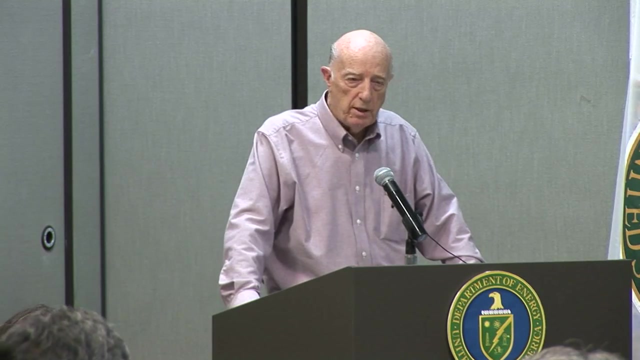 I'm coming out and work with you for a couple of hours And that was a great experience And we built a kind of a first of a kind model on the risk of losing a shuttle as a result of failure of the auxiliary power unit. 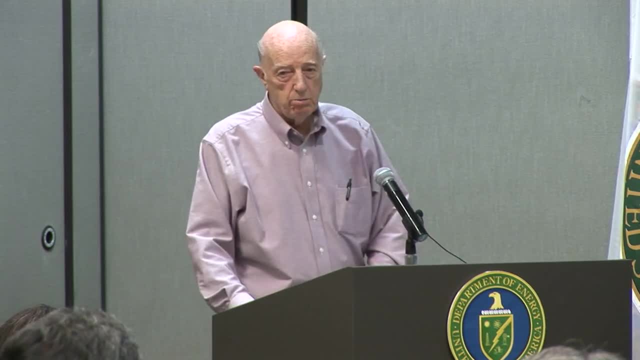 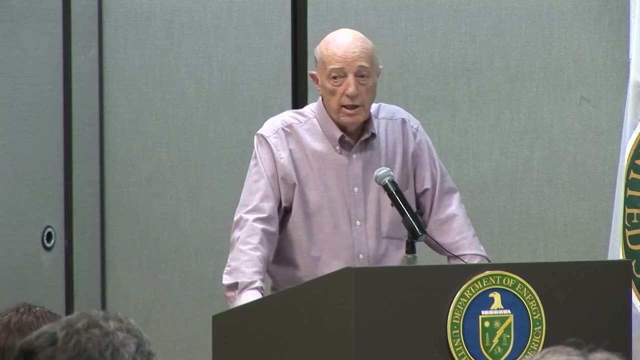 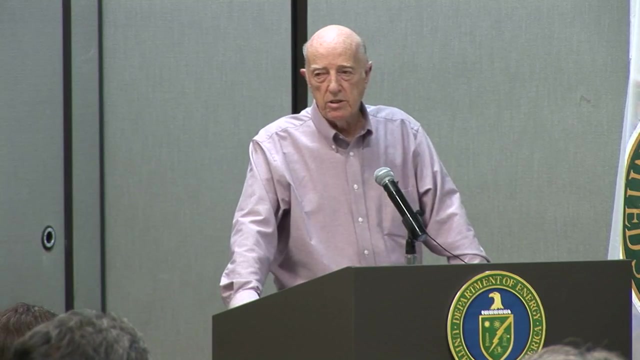 Now they had triple redundancy, but it really wasn't triple redundancy. when we started examining it, It was more like they had one and a half rather than three, because the real reason was because they had not given a whole lot of emphasis to what we had commonly referred to as common cause: failures. 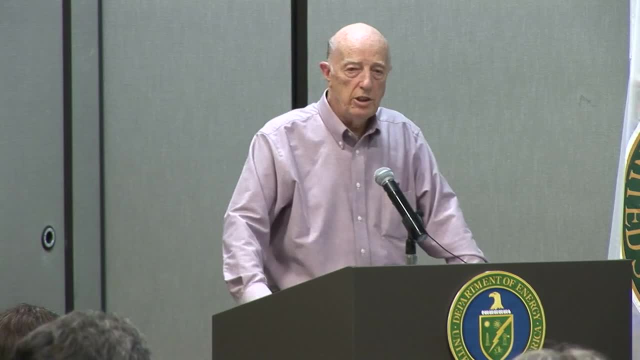 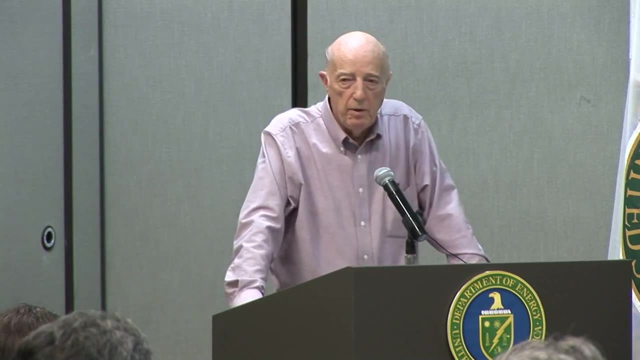 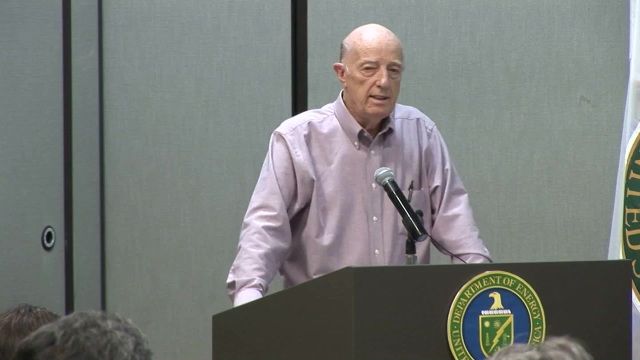 But that resulted in some real changes in thinking and increasing acceptance on the part of NASA of probabilistic approaches, because they were really down on probability. That all is rooted back way back to about 1956 or 7, when GE was asked to do a risk. 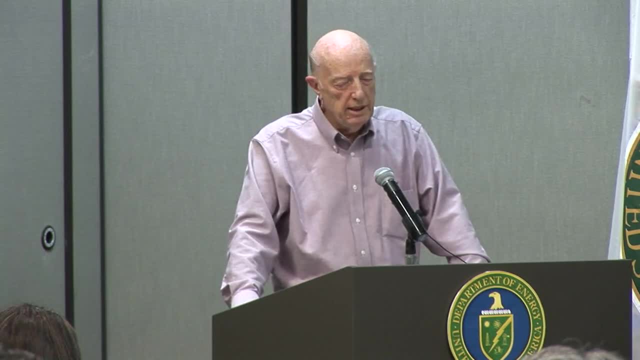 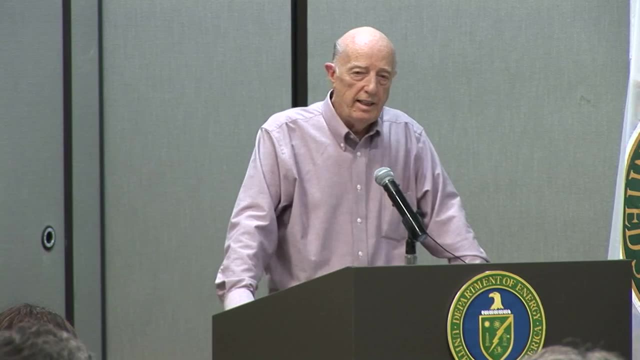 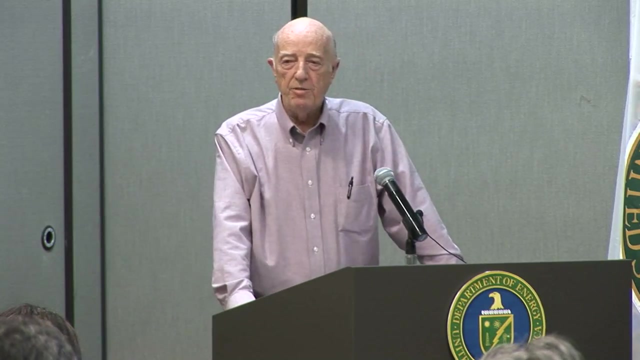 a risk, a probability analysis, of getting people to the moon and back, And the number they got was very low And that soured the agency and it took a long time to overcome that. Now, interestingly enough, they have a PRA group in headquarters. 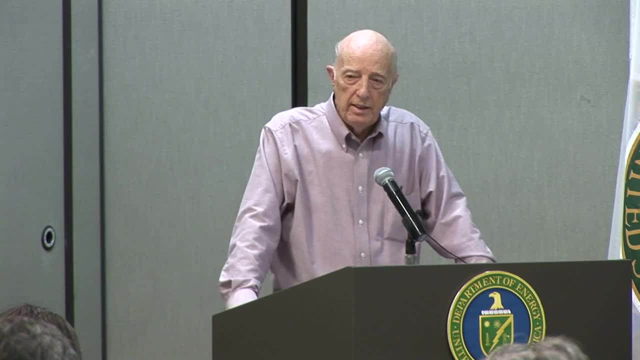 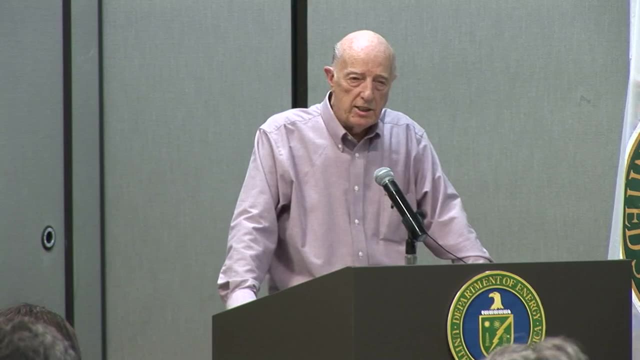 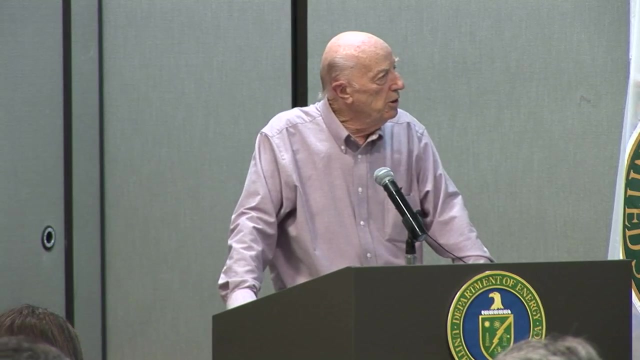 They happen to be headed by two former nuclear people, And I'm on a National Academy Committee right now looking at the risk of astronauts getting cancer from deep flight, deep space flights. So we're we're making progress there. So this is what we mean by a success diagram. 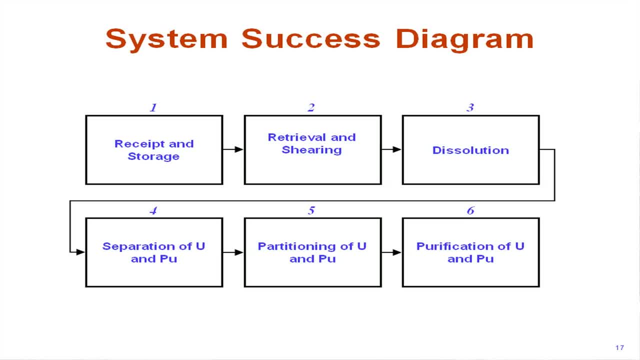 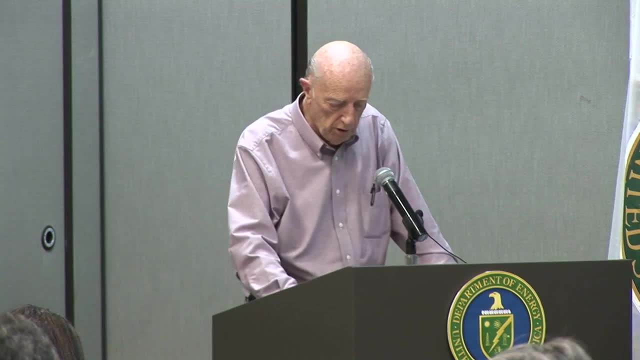 And I'm not going to- we're not going to- analyze each one. I mainly wanted to point out the process we go through in the in the development of what is called a success diagram and the linearization of the whole facility. We will talk a little bit about box number six. 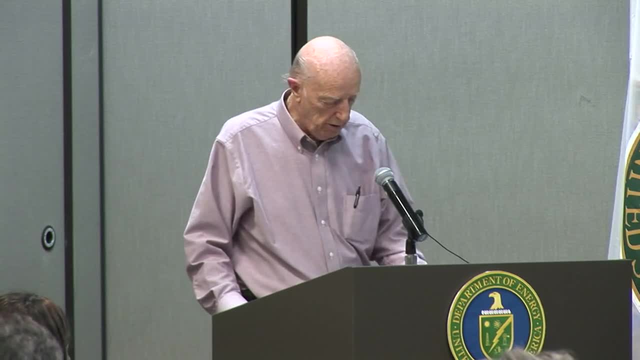 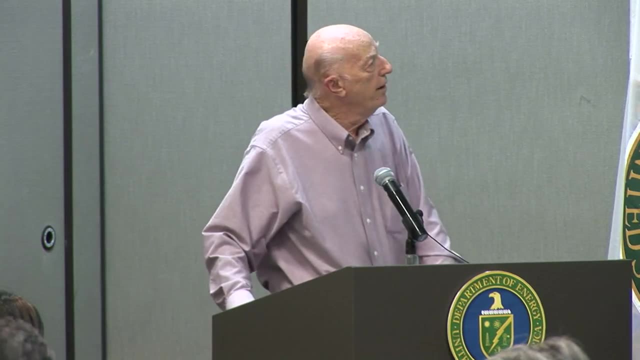 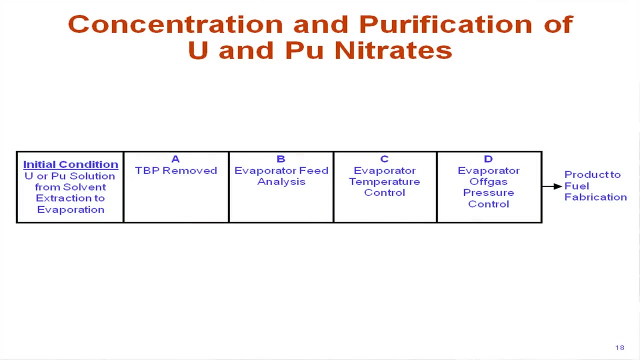 So if we decide we're going to analyze one of the boxes, then we turn up the microscope on that box. In this case, uh-oh, I went one too far. In this case, we decided we'd look at the concentration and purification of uranium and plutonium nitrates. 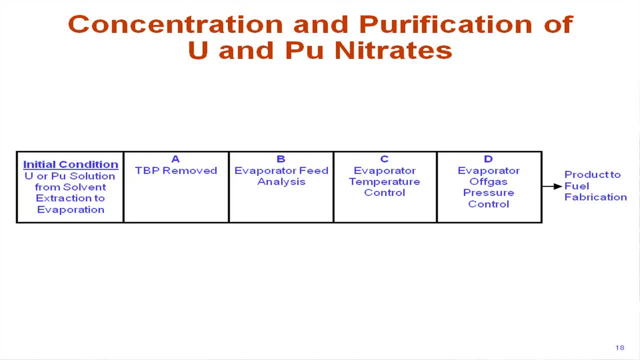 and ask the question: how would we analyze that? Well, this is what we would do: We would linearize it first, And- and what we're talking about here is that, in order for the evaporators to perform their intended function, 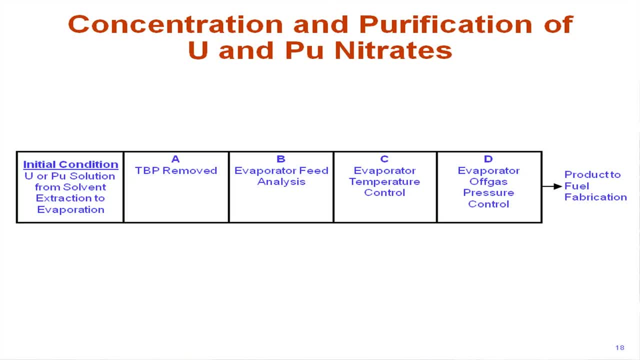 and without the high risk of a red oil incident. first, have to make sure that the TBP has been removed And, second, that the evaporator feed analysis is performed is indeed performed and appropriately acted on. Thirdly, that the evaporator temperature control 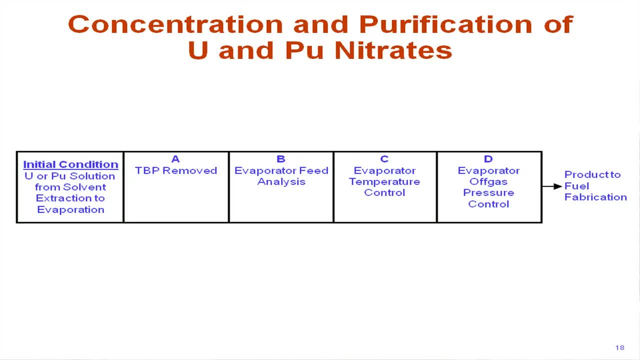 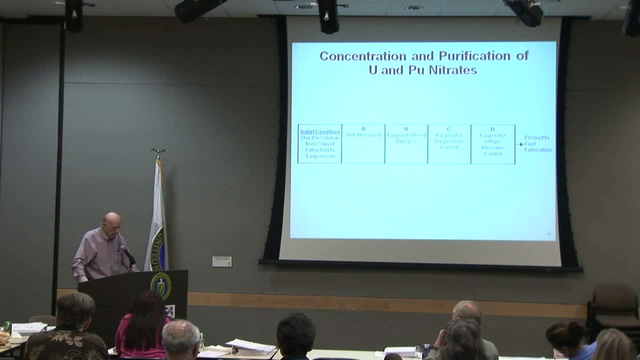 is keeping the temperatures below the prescribed threshold temperature, Maybe 120 degrees, And that the finally, the evaporator off-gas pressure control is is at its uh intended levels. And so this is we, we. 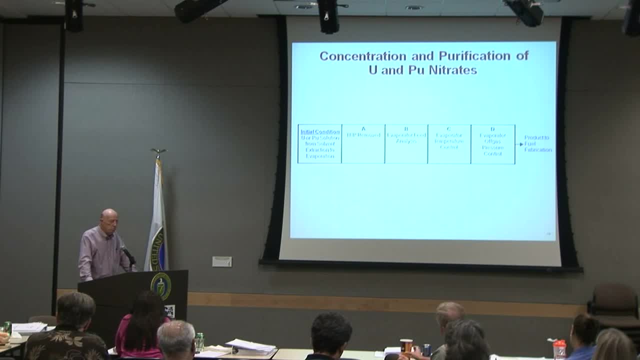 we uh really try to decompose the system uh into a, a, a point that it's uh manageable from an analytical standpoint and that it's uh useful from the standpoint when you're dealing with the people that really understand these. 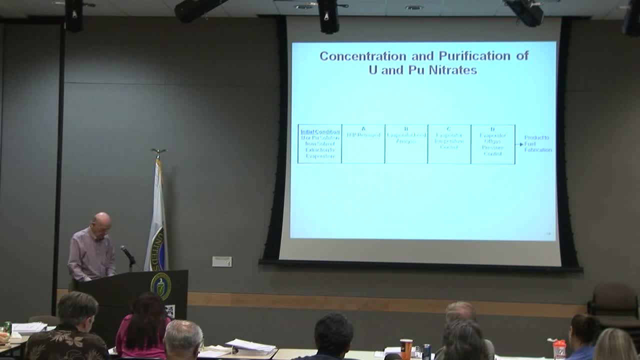 uh, how these things work, that they, they can interpret what we're trying to do. Okay, Step two: Identify and characterize the sources of danger. Well, we can get through this one in a hurry, because here we're only interested in. 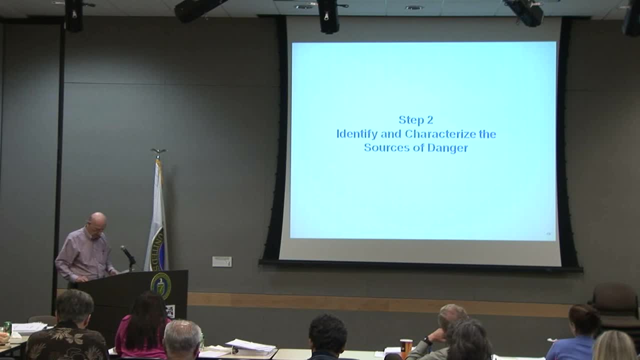 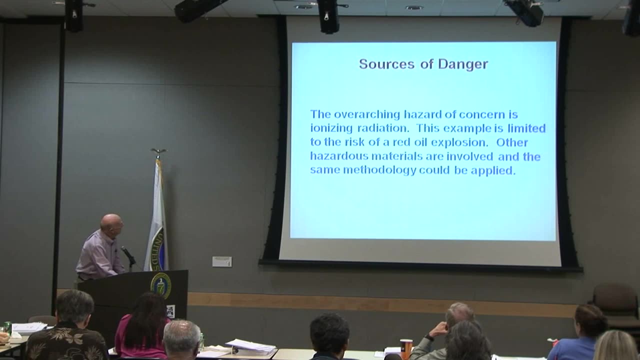 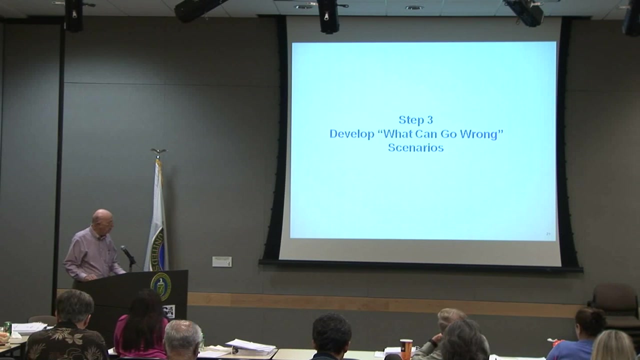 in radiation and uh uh. others are sometimes much more complicated than this. So, all right, What can go wrong scenarios? As I said earlier, this is the uh. this is the creative part of the work and this is where we needed the senior reactor operators. 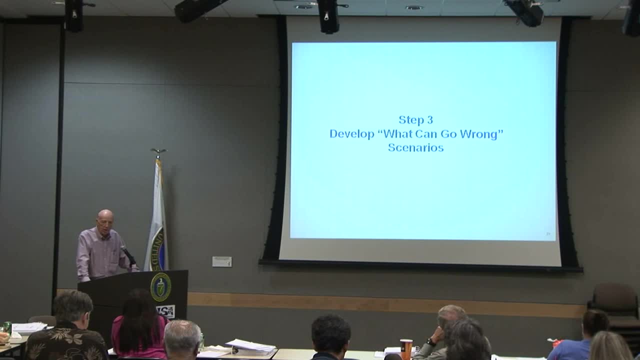 This is where you need the senior operators of any chemical plant and this is where you need to interact with the maintenance people and the designers. but you got to be careful with the designers, because what we found in collecting data from designers there's a tendency to be a little biased. 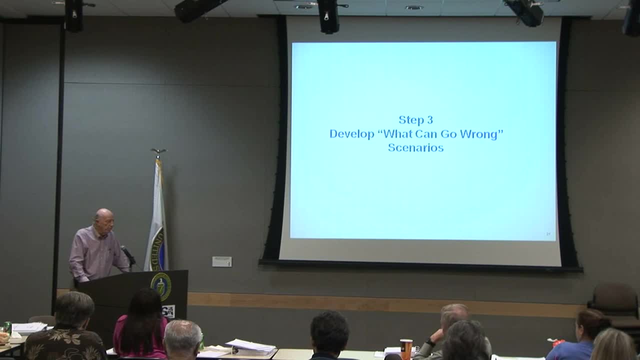 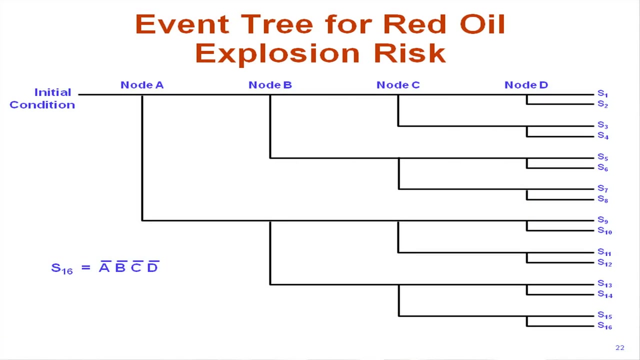 towards the six: the reliability of the system. And uh so, uh. how do we go about doing that? Well, uh, we the. the tool that's been most often used is the inductive logic model, or in the form of a. 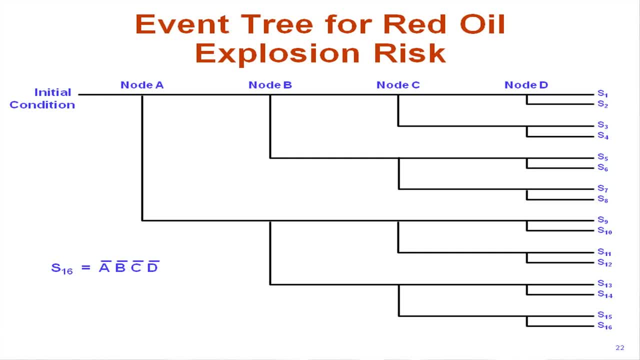 of an event tree, And so here, where we have uh A, we're really talking about, the box that I showed you earlier- is, uh, the. the answer is: has the TPP been removed? If the answer is yes, 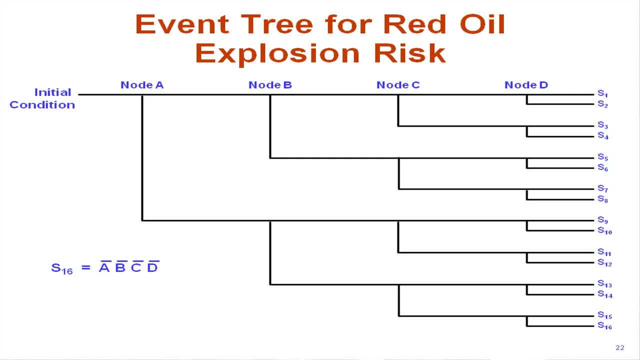 then you go to the right, And if everything is yes, if all the answers are yes, then that represents the success state, And if any of the answers are no, then you go downward into the, into the vertical state, And you can represent any single scenario. 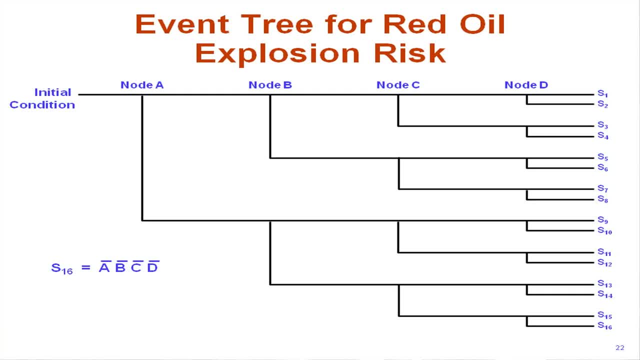 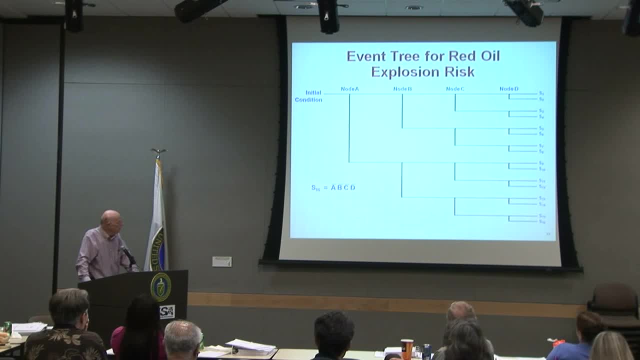 with a Boolean equation: And the A is that it's successful and A bar is that it's not successful. Uh, so this is an enormously useful structure within which to think. Uh, because we can represent this whole matrix with a simple operator. 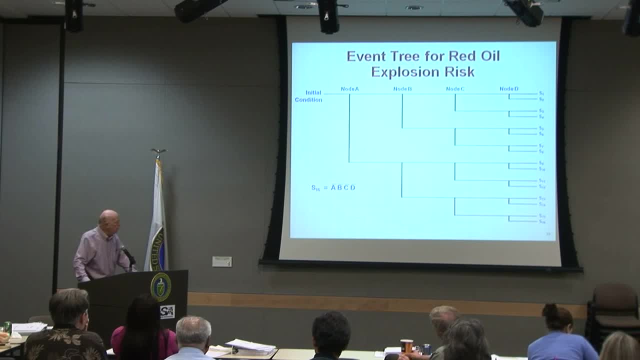 And, and we can do diagonals on that operator and answer the question: uh, given a certain input state, what's the likelihood of a a certain output state? And that becomes an extremely useful piece of of information. So we don't just calculate the risk. 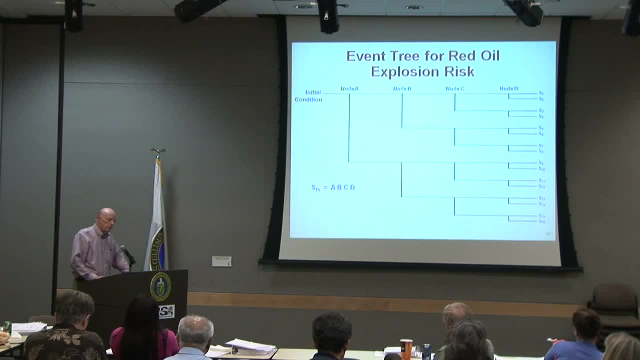 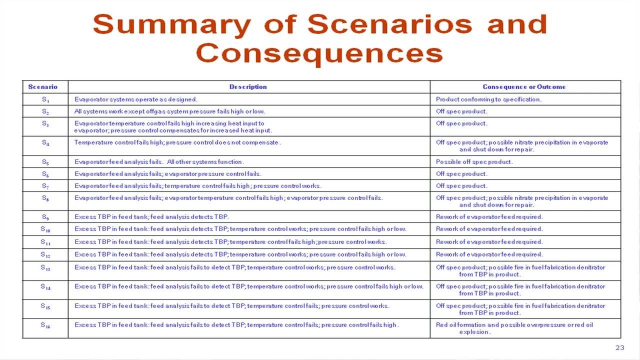 We really create, uh, the superstructure or the infrastructure of of the whole uh process. Uh, we put some information in this one, And this is- this is my token slide of that you can't read Uh, 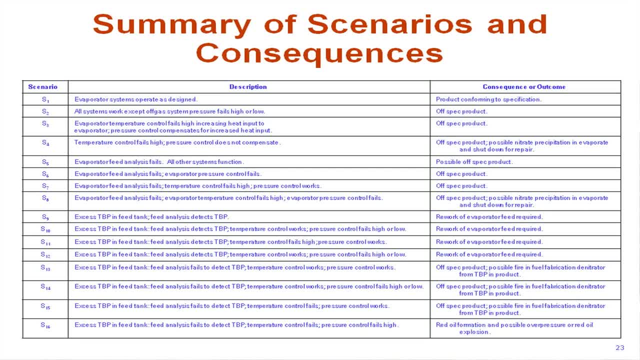 but uh it it was. it's done just to kind of illustrate how the process works. And except uh for uh, the last four, uh, the output state, the damage state, is pretty much uh uh. 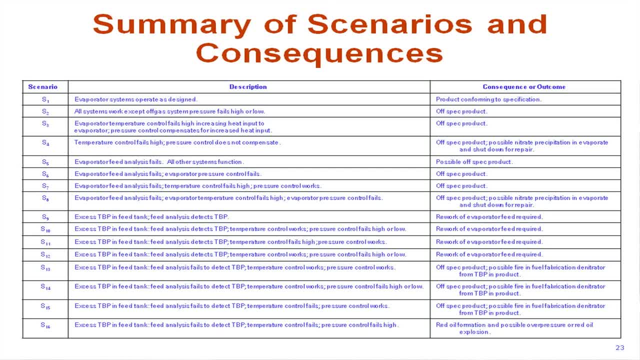 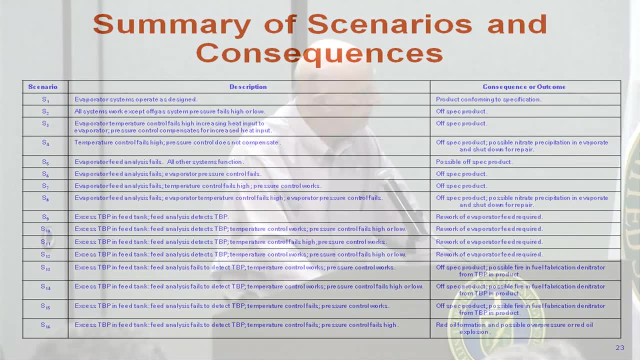 uh feed. that's off spec and it's very correctable. But you but down from S uh 13 to 16, you get into uh scenarios where you had more than one top event. uh uh not performing its intended function. 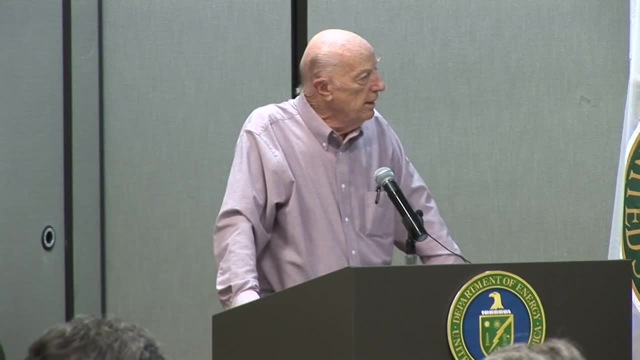 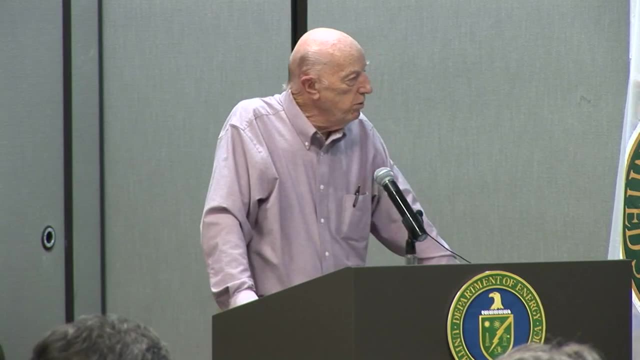 And you start to get get problems like fires and eventually, uh, something like an explosion or and the- and, of course, the red oil event is simply the distaste that uh, organics and nitrates have for each other. 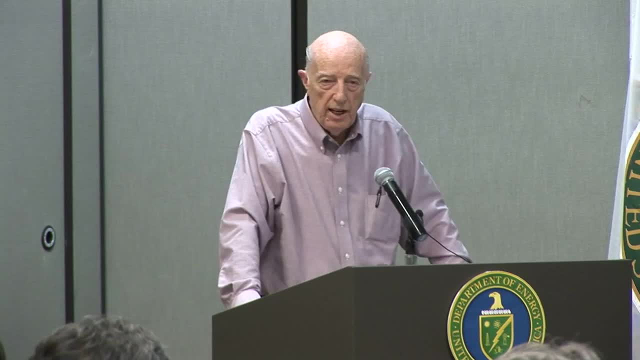 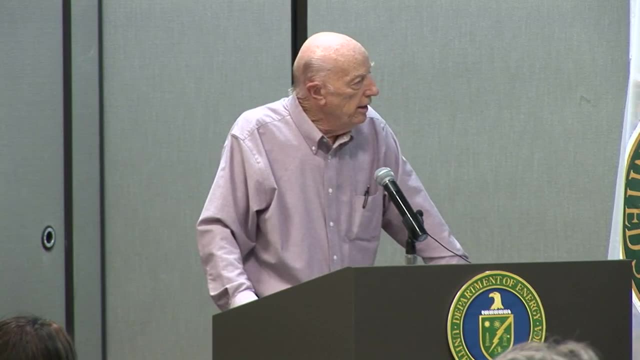 uh, and especially at elevated temperatures. And so if you have a TBP with its diluent, like kerosene or dodekane, uh and uh and uranyl nitrate or plutonium nitrate, uh, coming together at elevated temperatures. 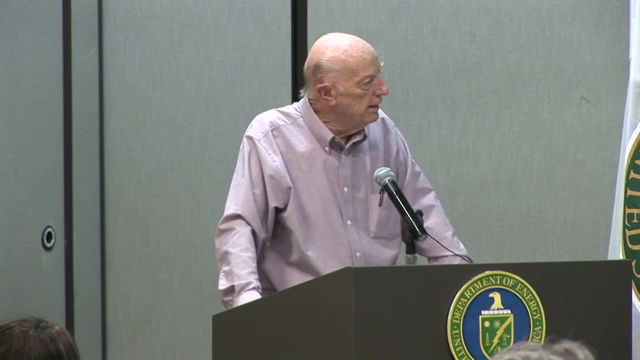 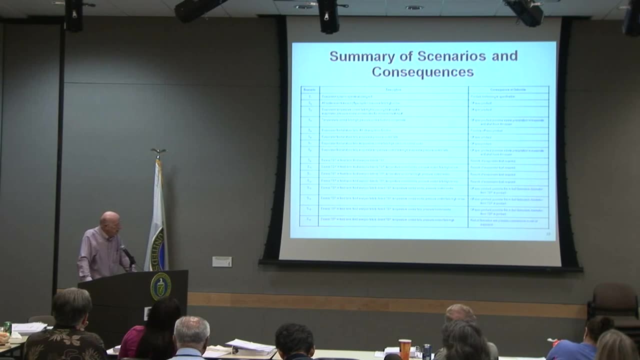 you get uh a degradation that, if uh uncorrected, uh creates a lot of uh uh gases, non-condensable gases, And uh the products include a lot of uh uh ice. 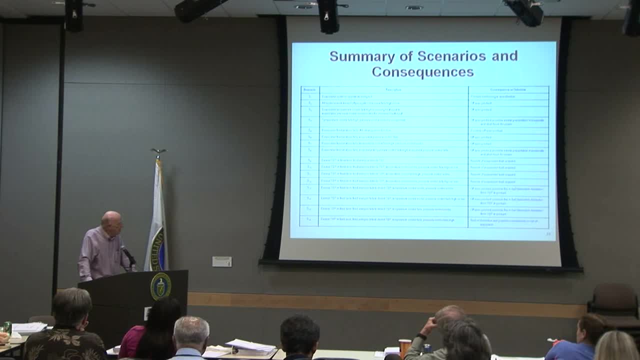 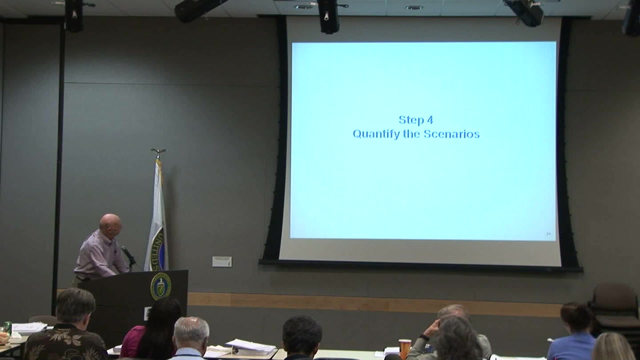 a lot of uh uh uh reaction products that uh can be very corrosive and sometimes explosive. So this is the type of information, Uh that you'd uh get out of the scenario. Now, as far as the quantifying the scenario, 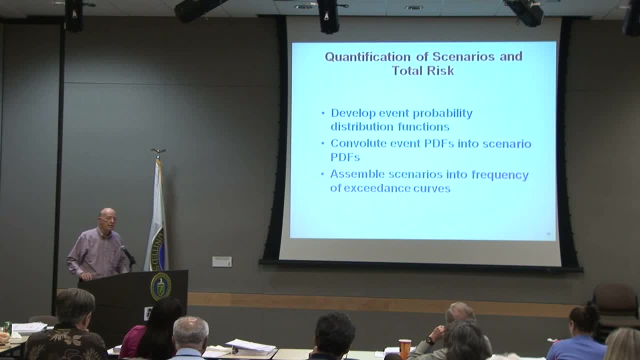 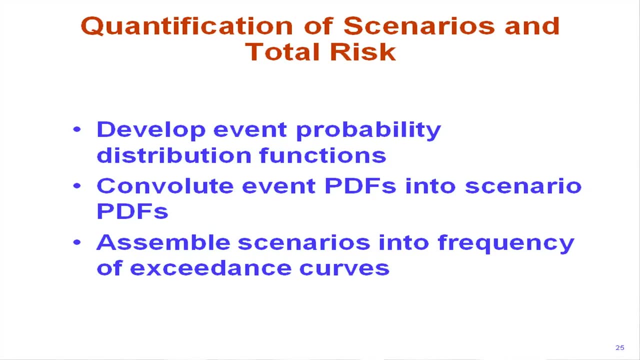 step four- this is the most fun to us- that uh studied applied mathematics and physics and neutron transport and what? uh? Yeah, I have a question In your eventually, all the knots you have there, there is any, uh. 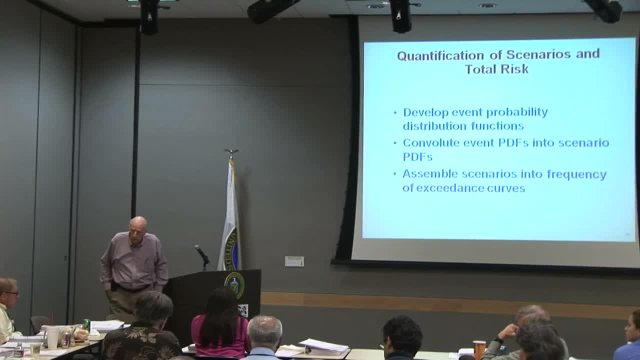 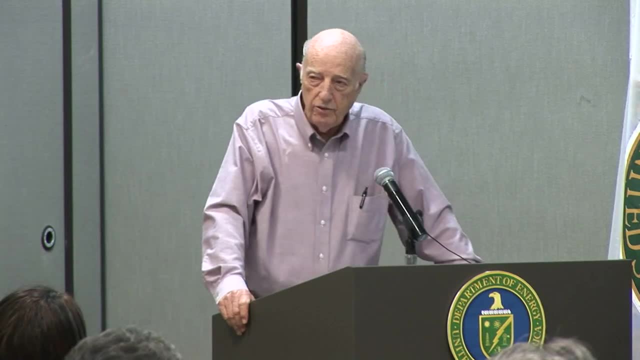 condition, uh, probability that happen, All of them supposed to be, you know right or wrong. Oh, what you're saying is: uh, we we're is it. is it a binary system? And uh, generally, 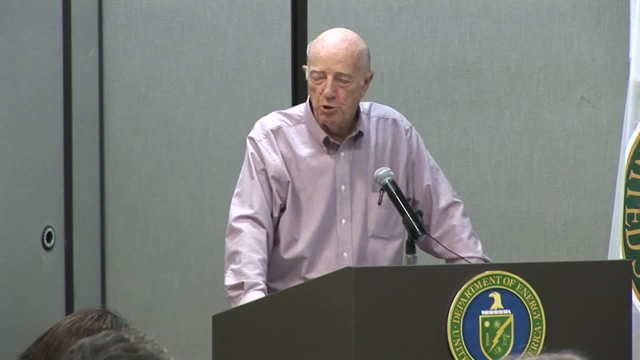 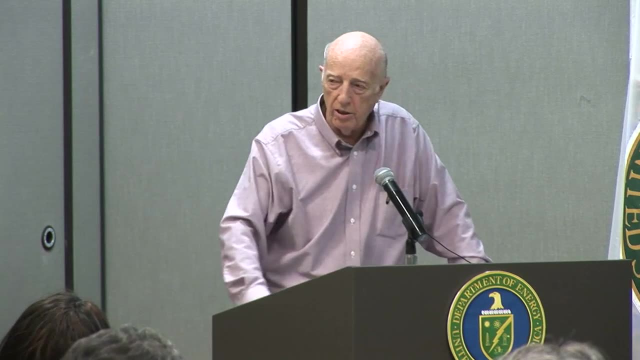 we can. yeah, There is a lot of uh uh, what if? what if? Sure, But you can get out of, out of the box. So Sure, No, we well the answer? the answer is: it depends on what you're looking for and the model. 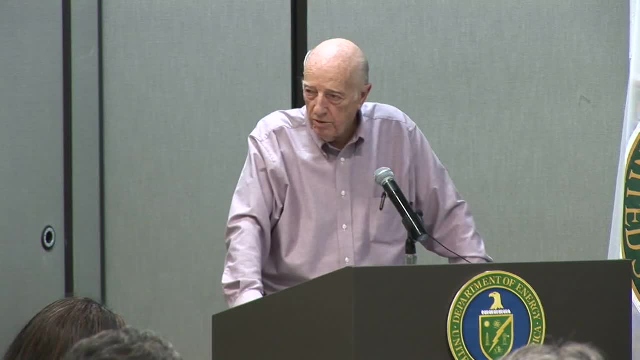 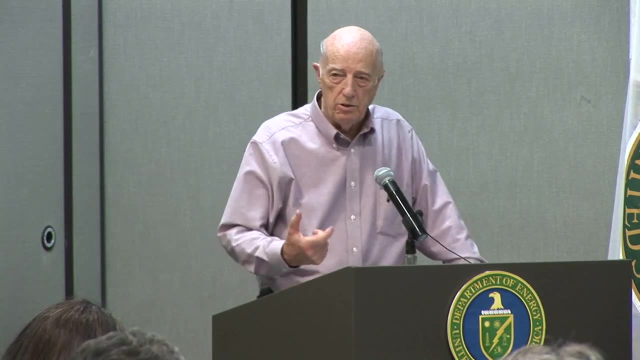 You don't have to have just two states. You can have multiple states, You can have degraded states. You can put that in the event tree as well. Uh, in most cases, what you do is you, you. you treat all of the. 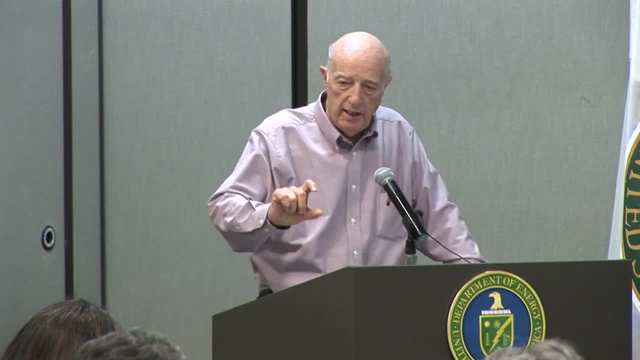 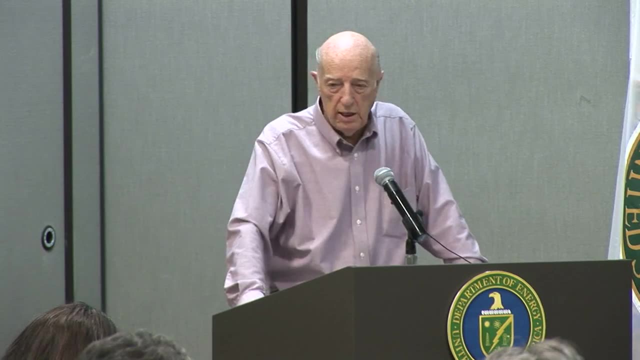 uh, conditions under which you can get failure. Uh, and that may be multiple states as one state. Uh and uh. that's that's why it's so important to put the time that's needed into defining the success state. 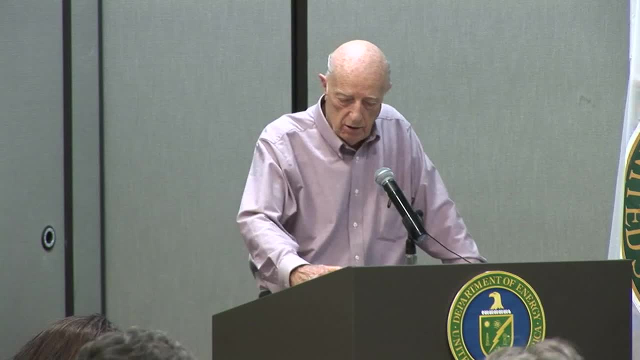 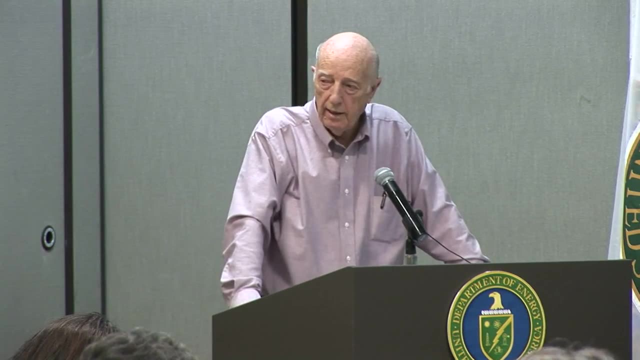 But no, there's no, no restriction on the mathematics. You can. you can uh uh. you can put uh uh. calibrate, you can calibrate different states and and and analytically analyze them. 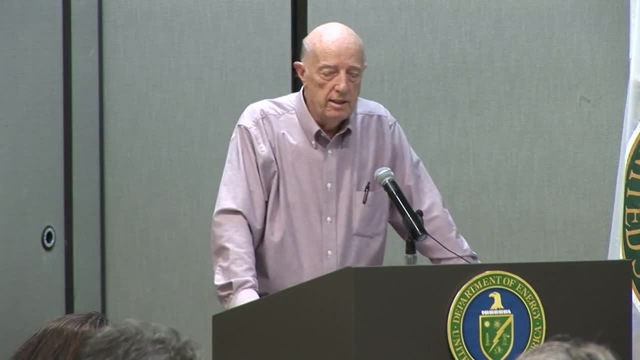 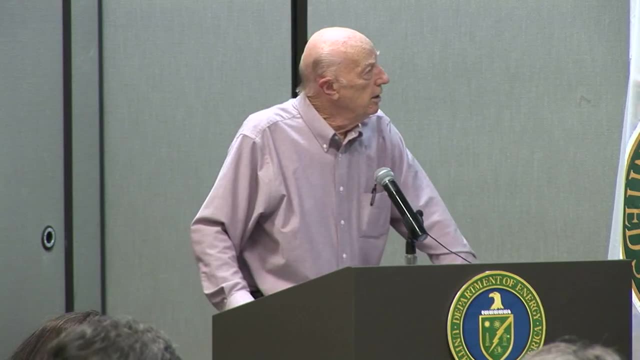 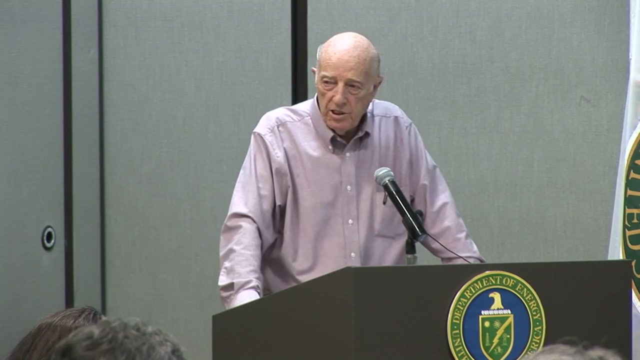 Okay, uh, so what? how do we analyze this? Well, we, we calculate our credibility factor, our probability, uh, distribution, uh, at each pa-, at each point along the way In the event tree. you first have to have the. 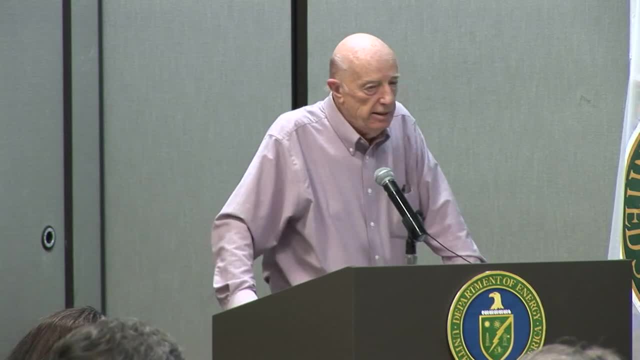 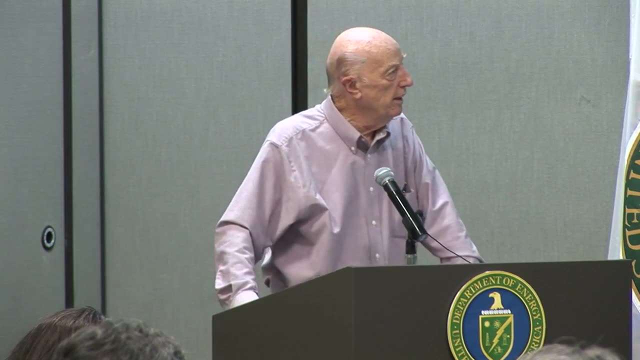 uh probability uh of uh the initiating event, And then you have to uh at the split fraction or at the branch point, have the probability of it going uh down rather than across, and so on. 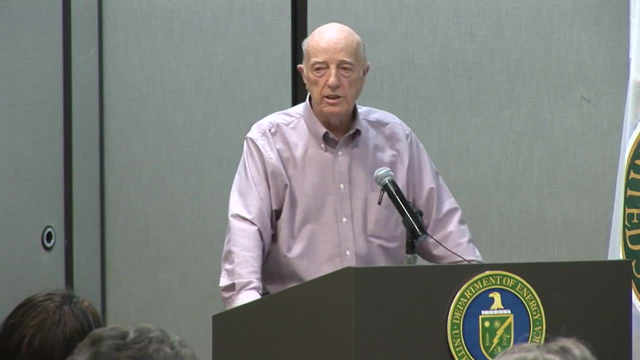 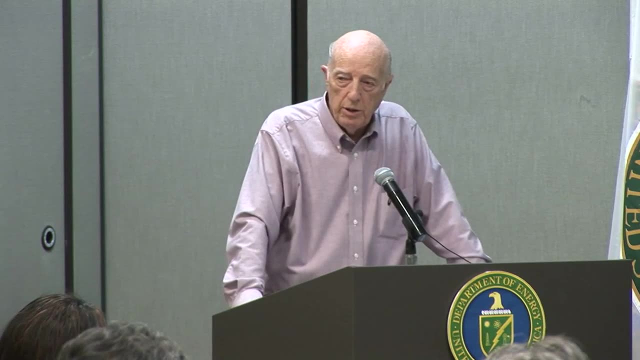 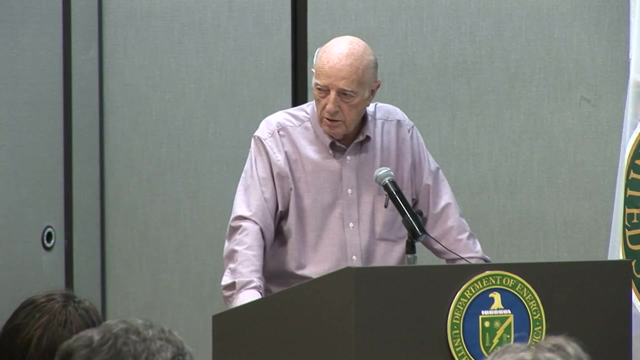 And, uh, you have to. uh, and the way we usually do this is: uh, we ex-. we usually adopt frequency as the measure of risk, but we also know that that frequency has uncertainty associated with it, So we put that frequency in a probability distribution. 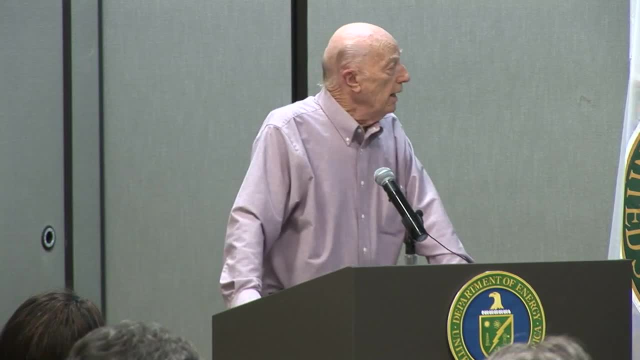 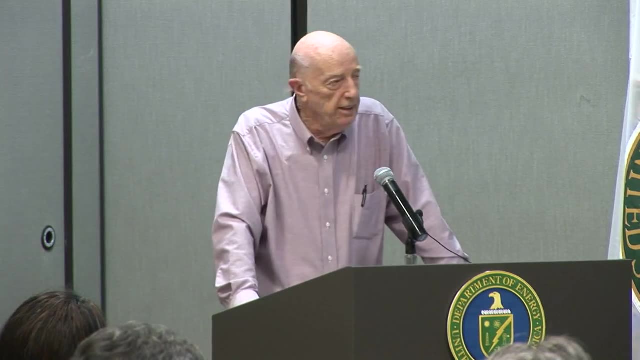 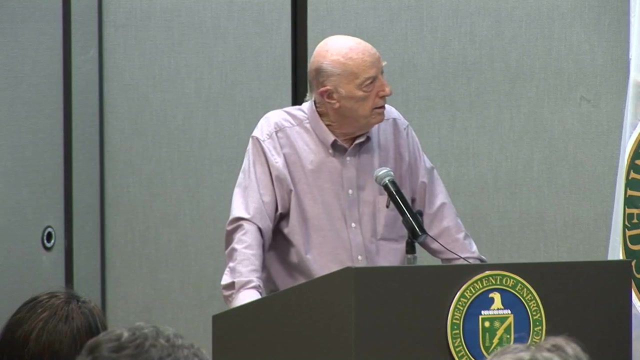 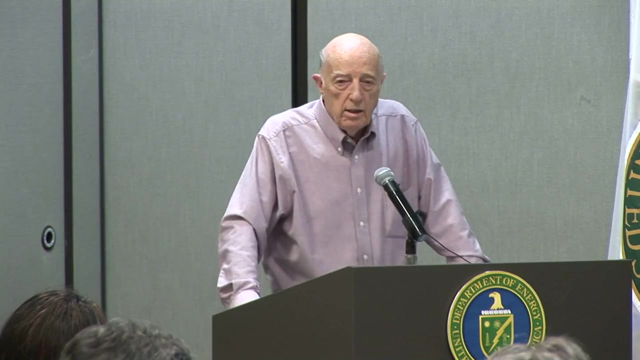 And that's the PDF. Uh, then we need to convolute, uh, the event PDFs into scenario PDFs And that's just uh, probability arithmetic, usually done by monochartal sampling or some other sampling method, And then we have to somehow assemble those results into frequency of exceedance curves. 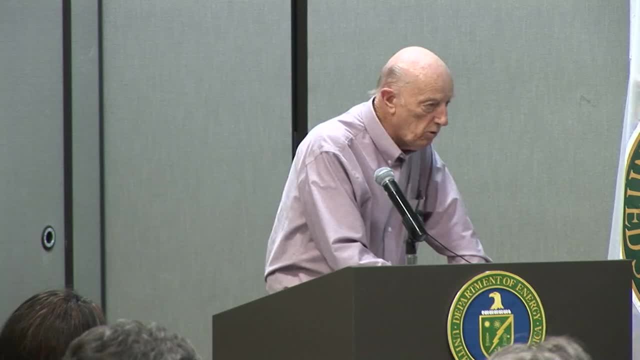 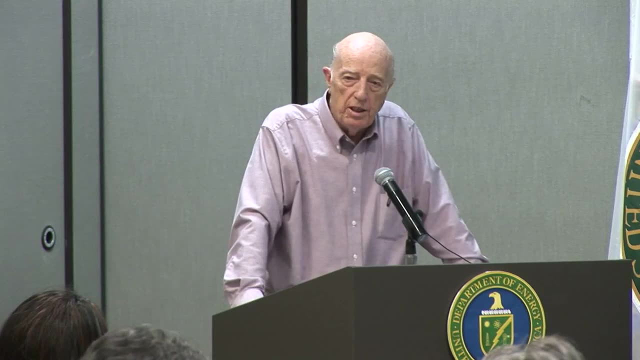 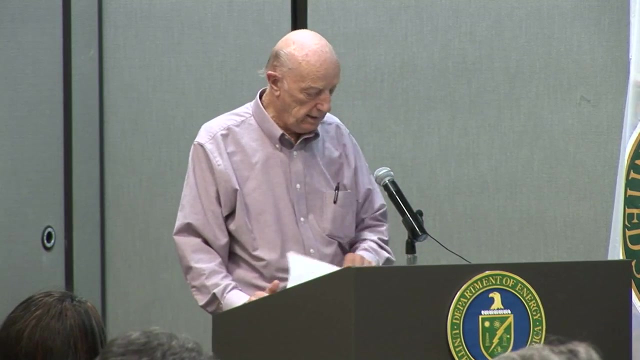 or the more esoteric label that uh. uh. Mike Vogel used the complementary cumulus cumulative distribution function. Uh, but the complementary cum- cumulative distribution function has sort of surfaced as the classic risk curve. Uh, so we go back to our 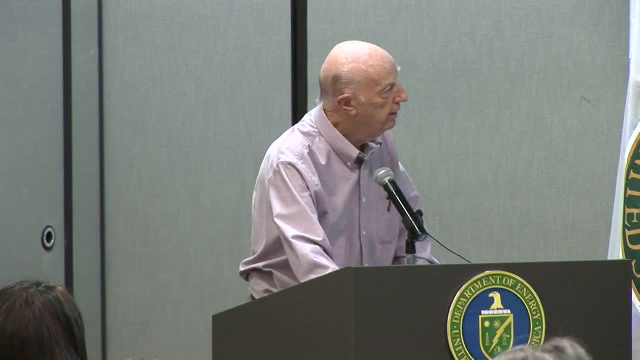 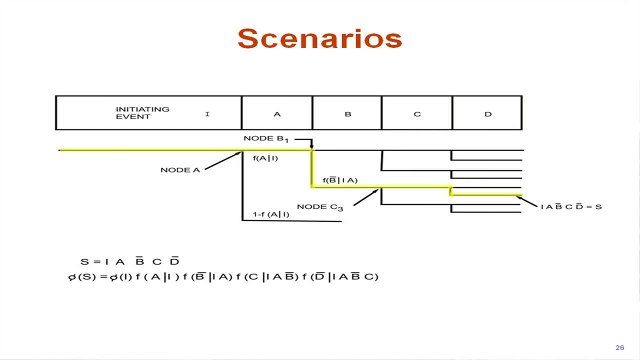 our event tree And this sort of illustrates the process. The A, B, C, D correspond to the success uh uh boxes that we showed. We showed earlier And we pick any path we want And, of course, what we end up doing is quantifying all the paths. 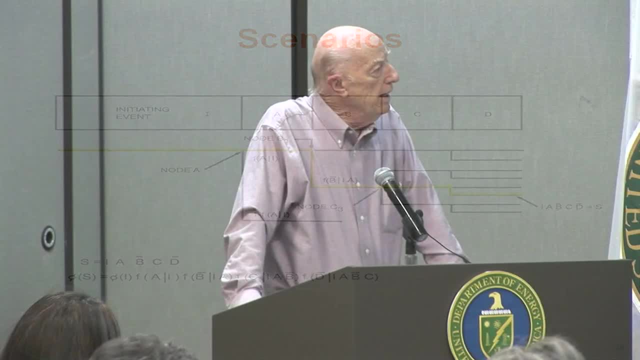 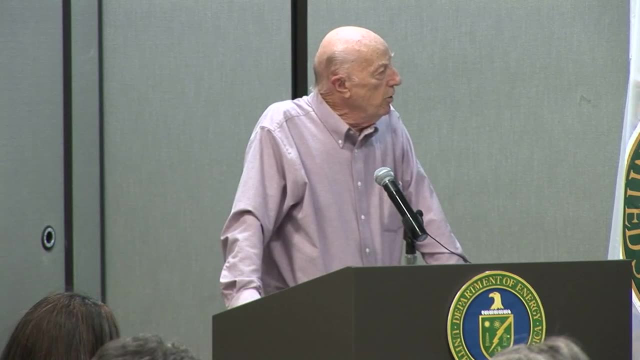 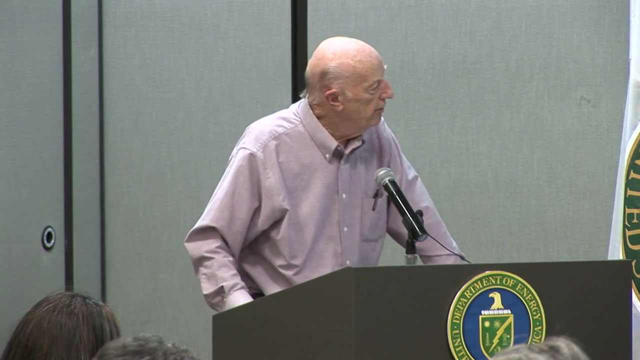 And we can uh, but if we pick the highlighted one, then on the lower left there you see the Boolean expression for that Uh, and then of course the frequency uh version of that is follows directly from that, And so now we have a. 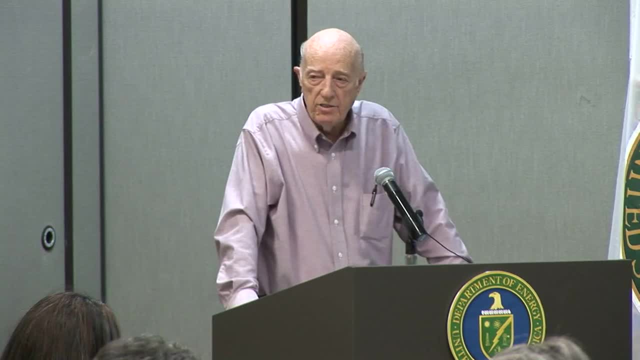 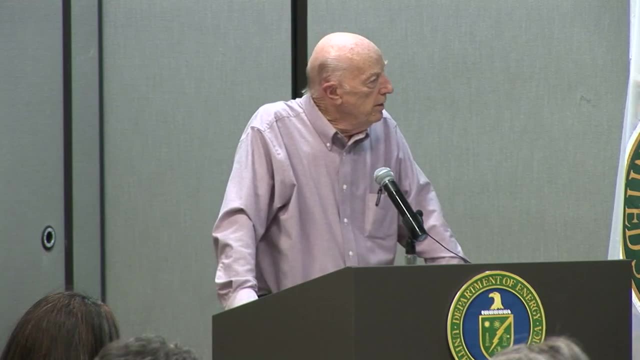 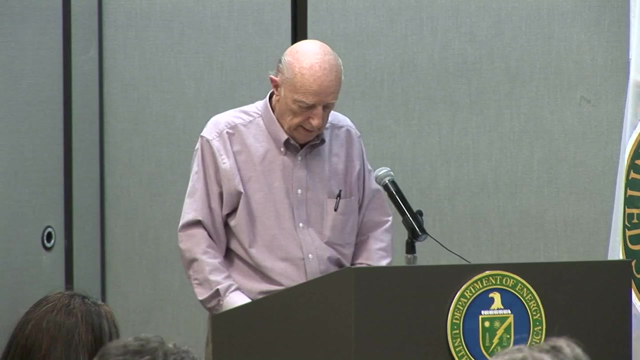 a Boolean equation for the frequency of occurrence of that scenario. And since that end state of that scenario is the damage state, we also have the uh frequency equation for that, for that damage state. Uh and uh, we will. 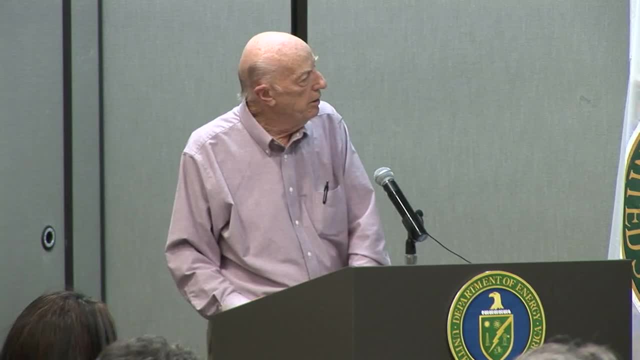 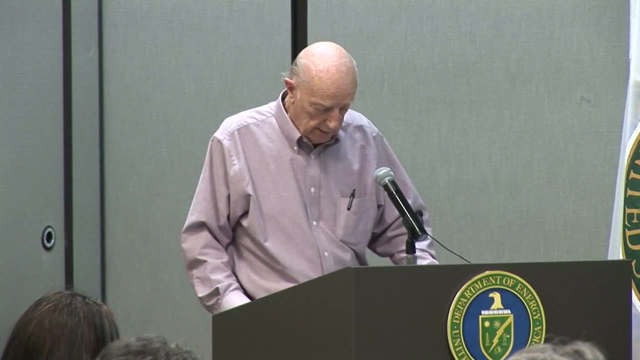 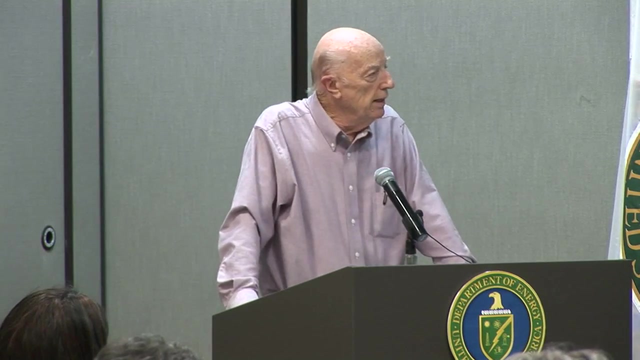 in a few moments. uh say, uh go, uh, talk about what the next step is after you get the Boolean expression Uh, but uh, if you pick one of the of the branch points, what you usually then do is: 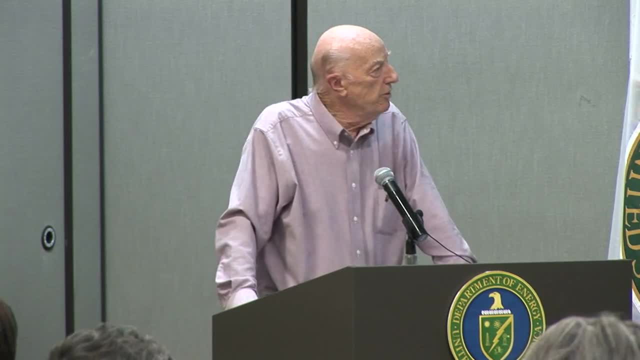 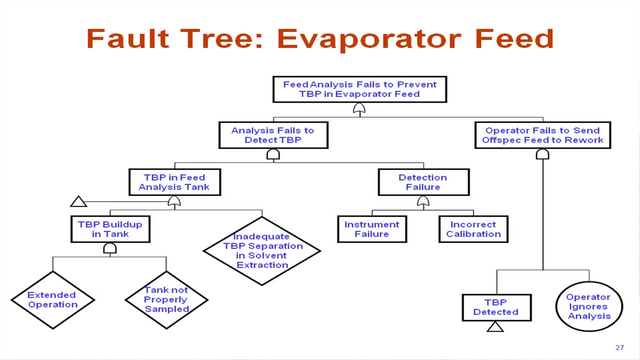 uh. another type of diagram: uh, in this case it was a fault tree. uh is used most often, although not always. uh to quantify the branch point. So the branch point that says feed analysis fails to prevent TBP in the evaporator field. 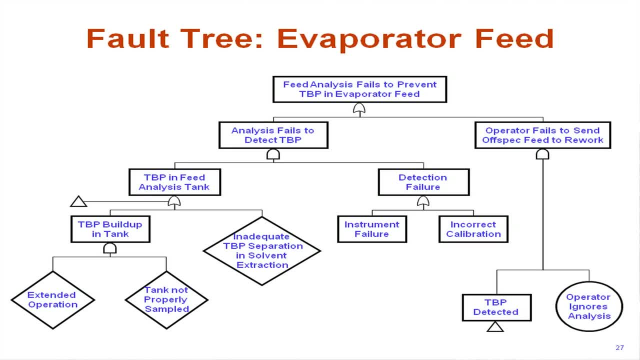 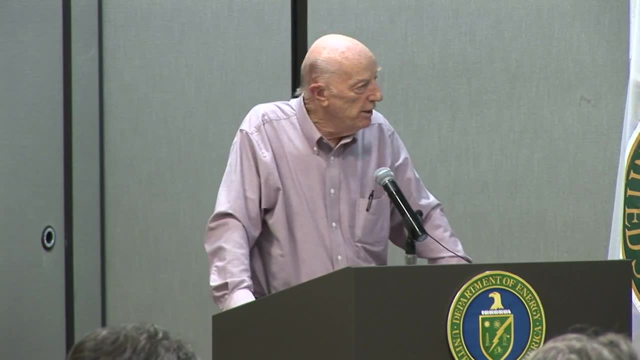 uh. well, that can happen only if analysis fails to detect the TBP, or uh the operator fails to send uh the feed, uh back, so to speak, And then you can kind of work your way down. The diamonds tend to indicate that it needs further development. 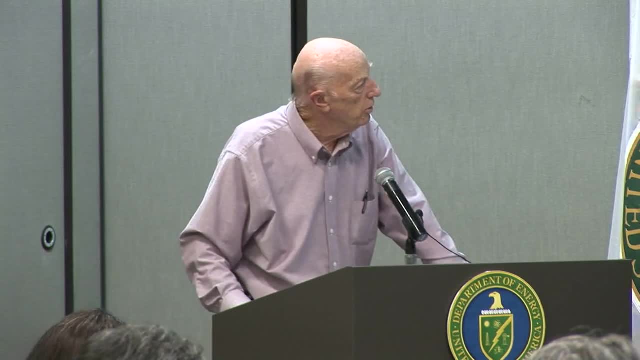 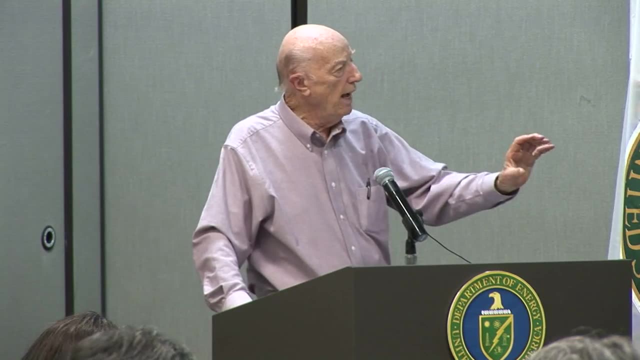 Uh. the basic events are usually denoted by the, by the circles And of course you have transfer points. Some part of your fault tree down below may be applicable to uh with respect to a feedback uh loop. 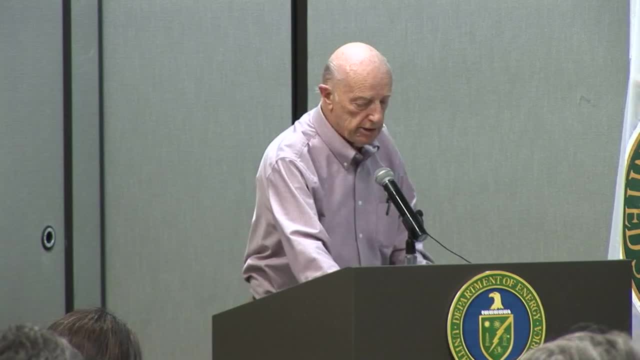 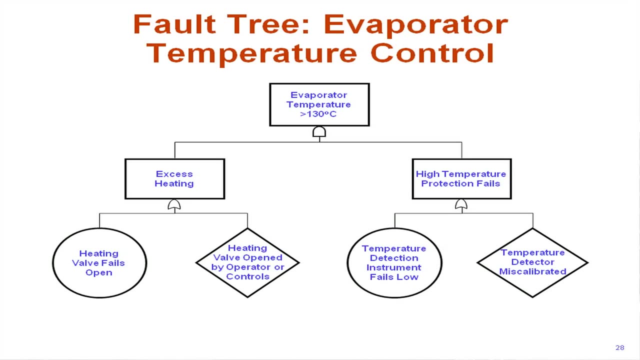 And so we here's, uh, the one for the evaporator, temperature control. Uh, you know, the whole issue is a a race between the evolution of heat and the dispersion of heat. And uh, if you, if you don't keep ahead of that race, 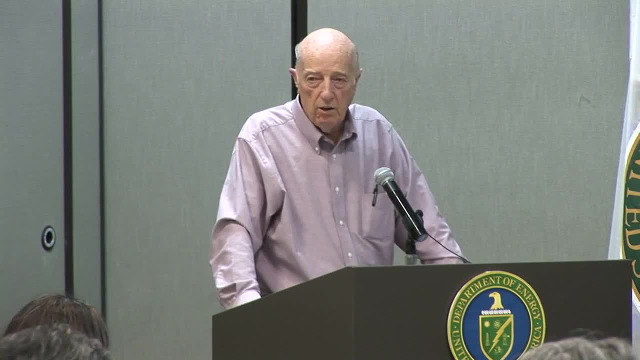 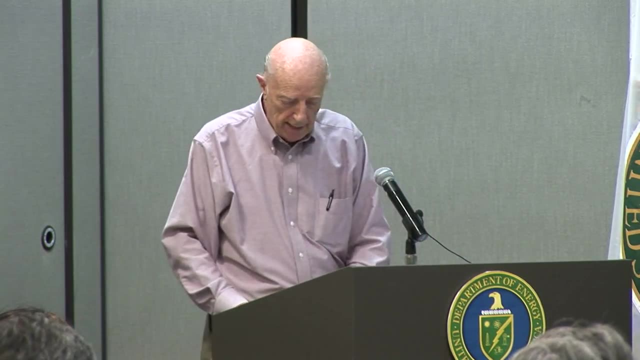 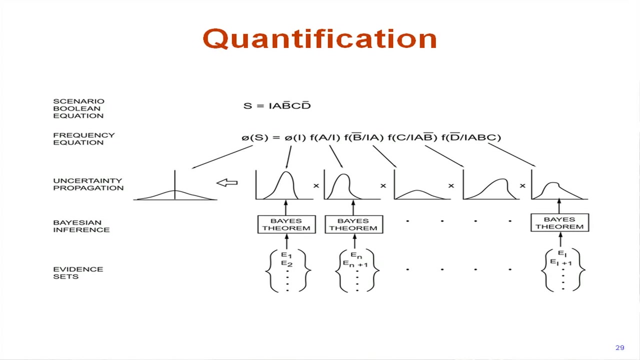 then you do get uh formation of gases and pressure and ultimately a pos, uh, a possible explosion. Okay, now back to the quantification. Uh, this is uh, basically probability arithmetic. So the, the, uh, the path that we had highlighted is illustrated here. 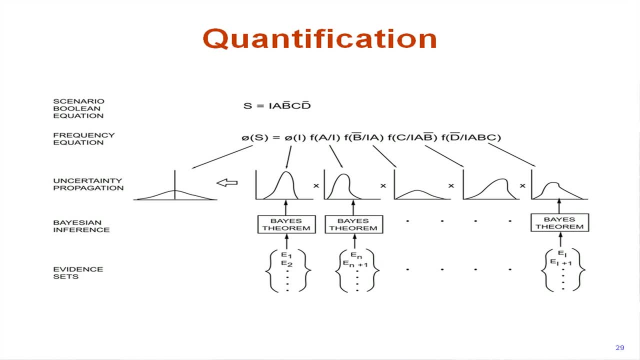 We started out with our uh scenario, Boolean equation- and we transformed that into the frequency equation. And then we, on the basis of uh all this supporting evidence that we could get, and keeping up with it through Bayes' theorem, 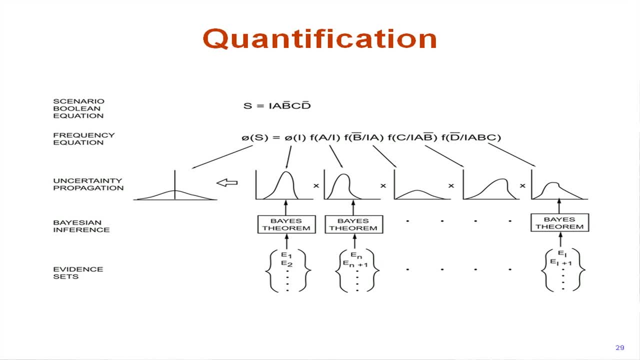 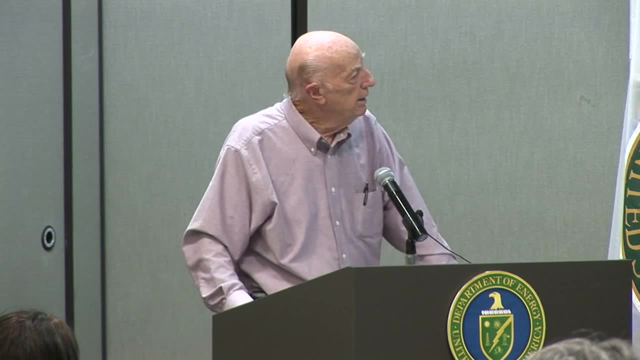 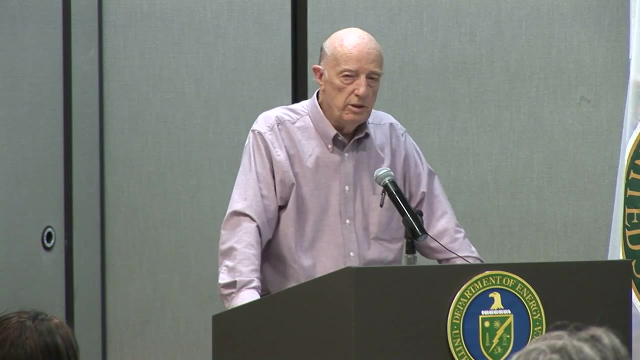 we developed the probability density functions for each uh uh branch points and the initiating condition or initiating event, And it's based on whatever evidence you can find, And that evidence doesn't just include uh failure rates, because sometimes you don't have much going for you there. 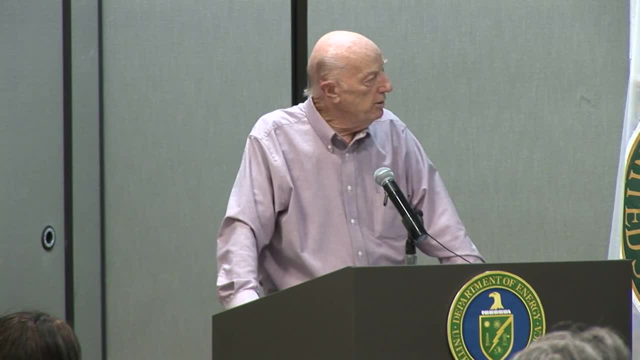 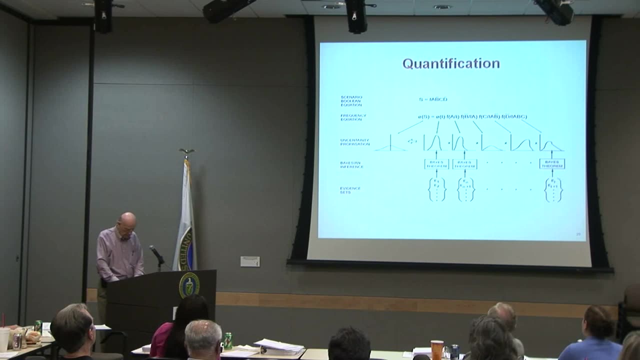 but it's expert judgment and uh experience and what whatever is seems to be uh relevant. Okay, The next step is uh the steps five and six, because I my only purpose here was to illustrate the process. 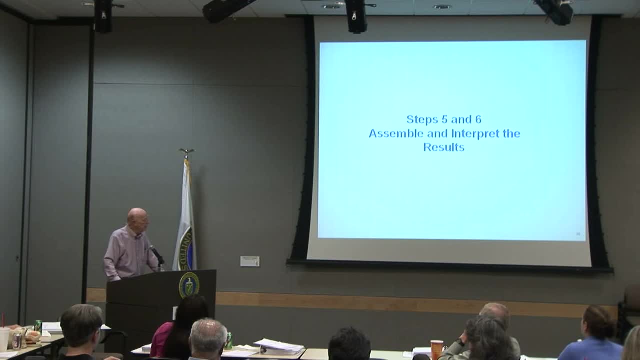 not to share with you a comprehensive analysis. If you uh want to go on West Valley's website and see an analysis of how this was applied to uh uh, a waste disposal facility. uh, that's easy to do Uh. 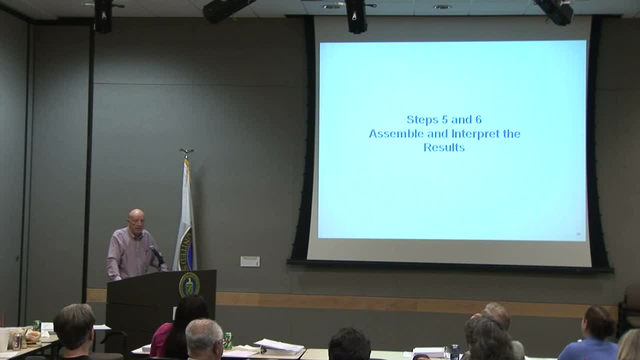 we've uh 700 page uh study. that was done in three months. Uh, and I remember my colleague at uh, Sandia, couldn't believe it when he he he was a reviewer of it. He was astonished that. 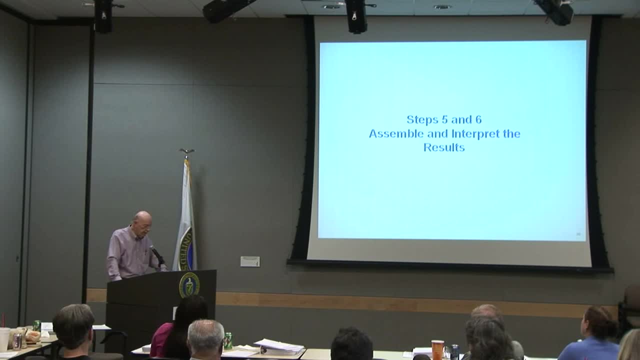 uh what we were able to do, I- and I think that's primarily because we uh have been doing it for a long, long time- and for all manner of things. We even uh analyzed the uh the risk of. 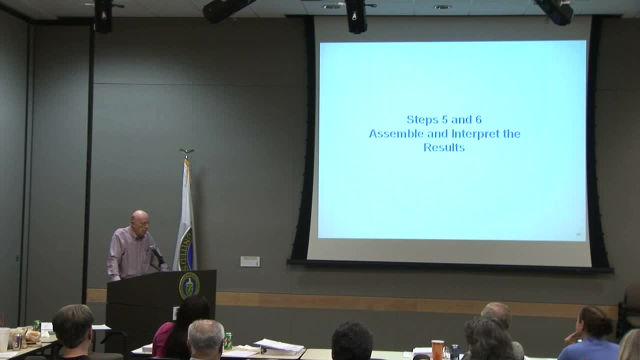 of the pickle factory being successful in in uh being able to uh uh generate or produce a certain quality of pickle Uh. my colleague Stan Kaplan uh worked for two or three years with the uh Department of Agriculture to bring this technology into the. 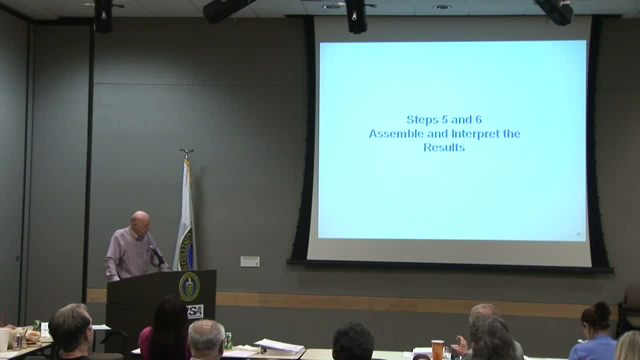 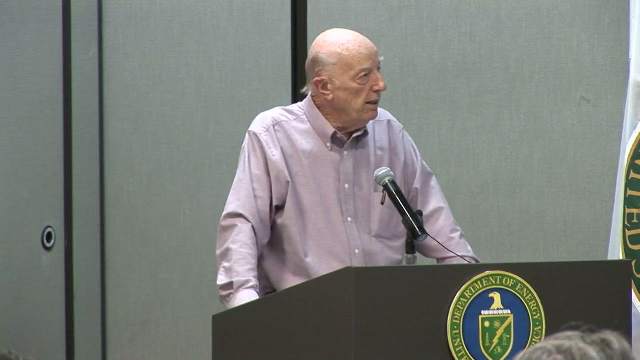 uh, food, food, uh quality business. Now I'm about done here. Uh, so these are the two principal uh displays that are you'll find, if it's a quantitative risk assessment And what I mean by that. 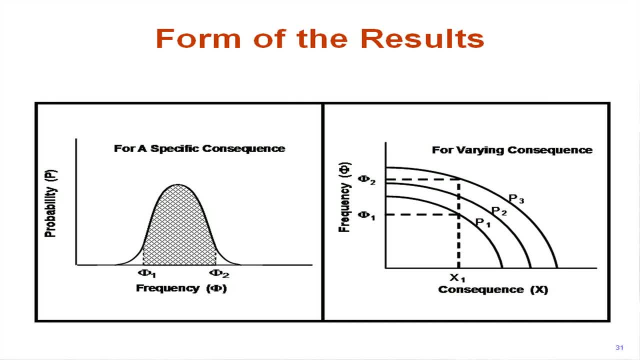 if it's a risk assessment that embraces the concepts of uncertain, the uncertainty sciences, Uh, if it's a specific event, like a specific level of damage or a uh specific dose, uh, the PDF is the. is the the way to do it? 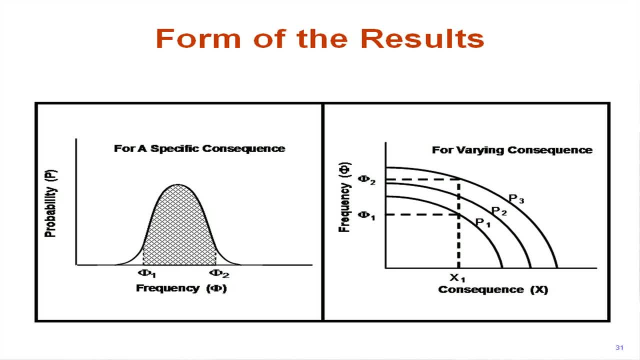 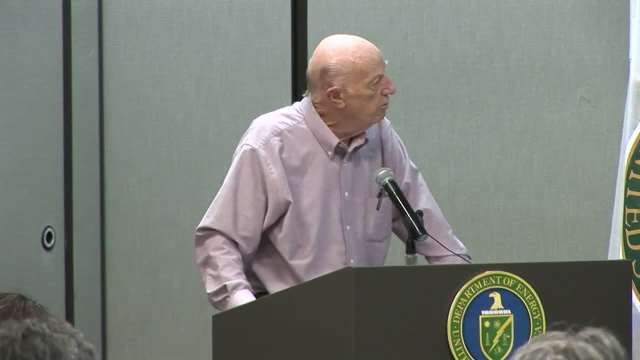 And all this portrays is that if the area under the curve that's cross-hatched is 90% of the area, then what that curve tells us is that we are 90% confident that the frequency of occurrence of that event is between phi 1 and phi 2.. 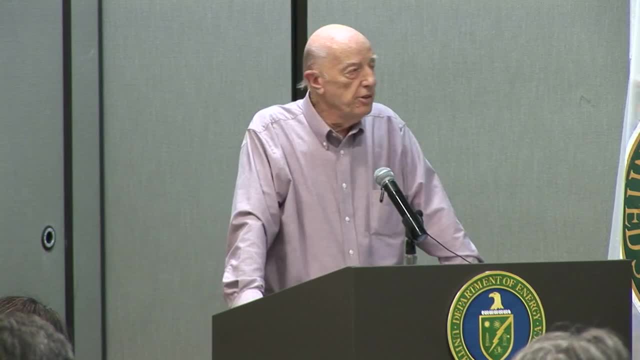 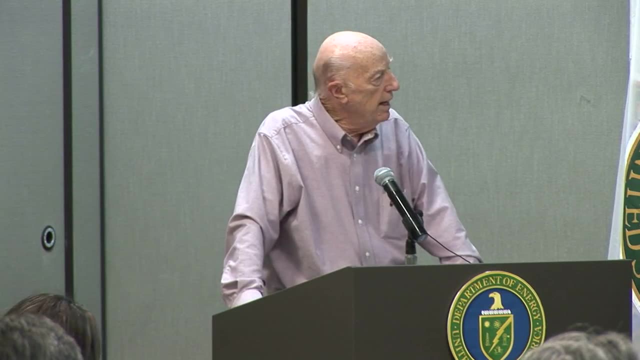 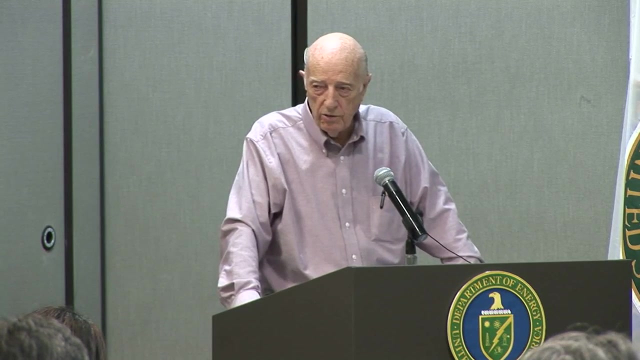 Uh, as to the integration process and the accumulation process, we go to a different kind of structure, And that one is achieved by taking all the PDFs of the, all the scenarios and accumulating them from the bottom to the top. You first. 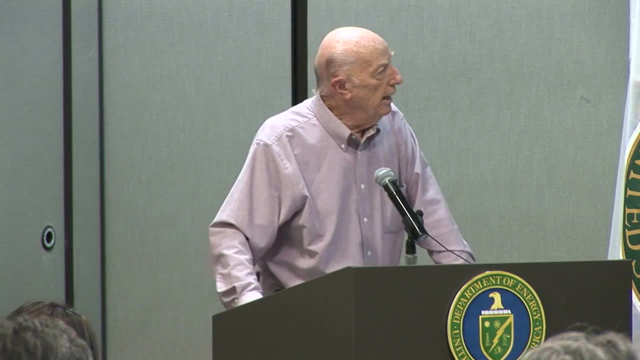 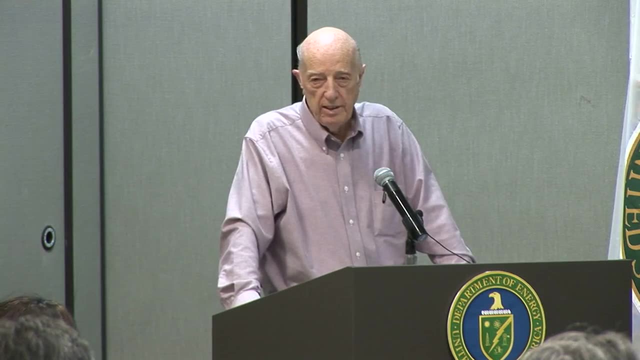 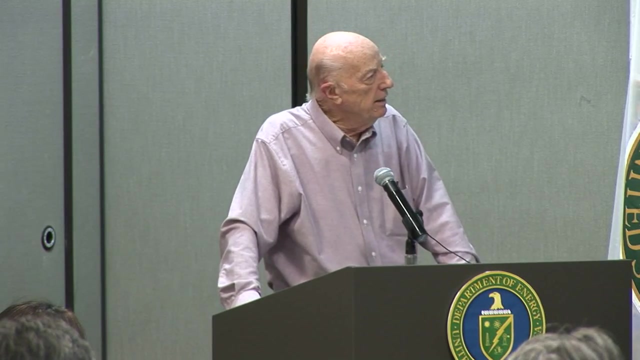 you have to arrange them in order of increasing damage and create what we referred to earlier as the frequency of exceedance curve. This is a very useful curve And it took us a long time to get the whip. uh, uh, format, uh. 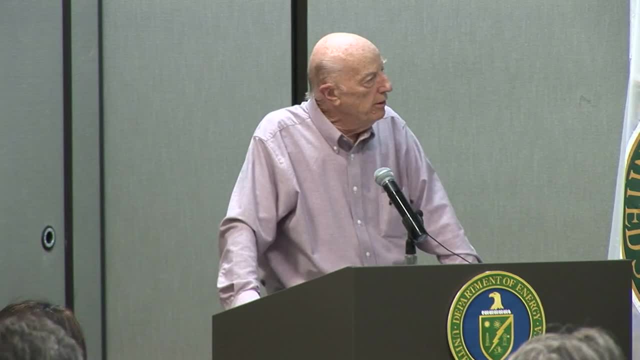 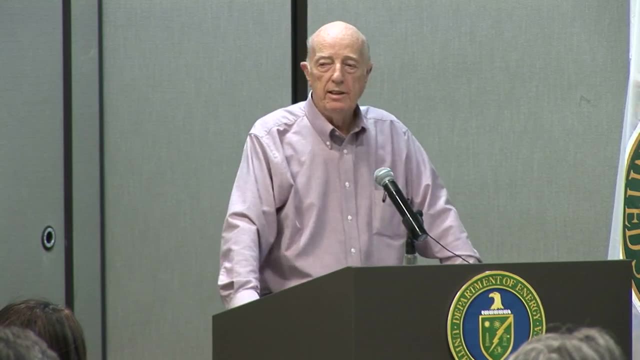 in in in this way And we even had some trouble in the early days of getting Yucca Mountain. And uh, I was in two different capacities In whip. I was uh on the National Academies Committee on whip and for 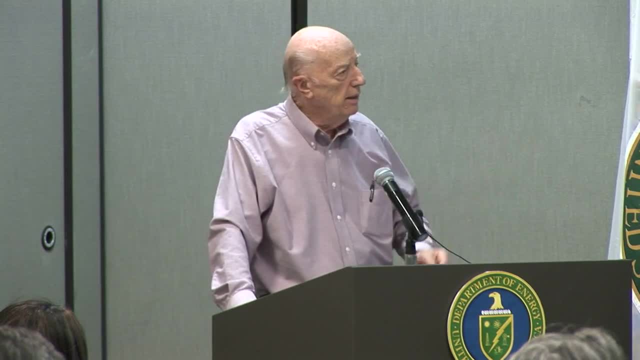 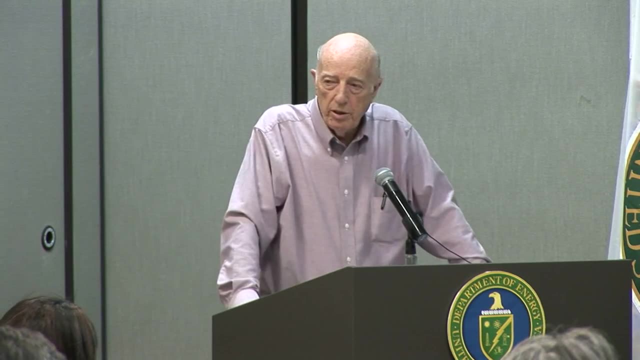 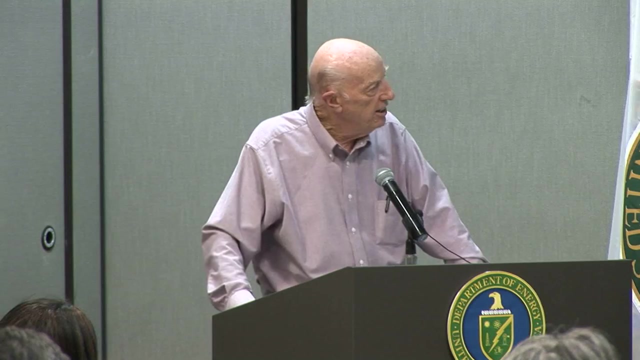 uh time chair of it And in the case of uh uh the uh Yucca Mountain, uh, my whipping platform was the board board uh Nuclear Waste Technical Review Board, which is a presidentially appointed board in which I currently chair. 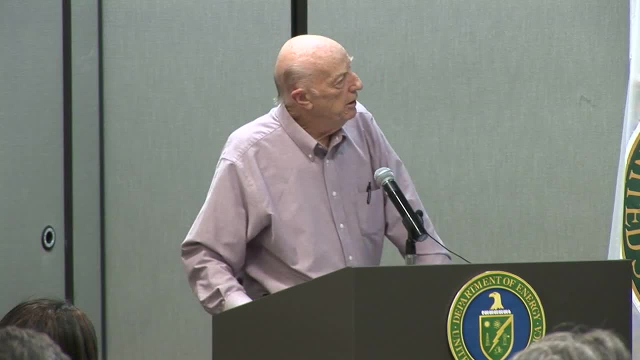 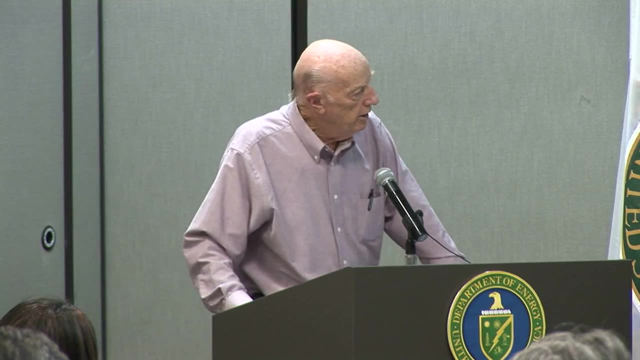 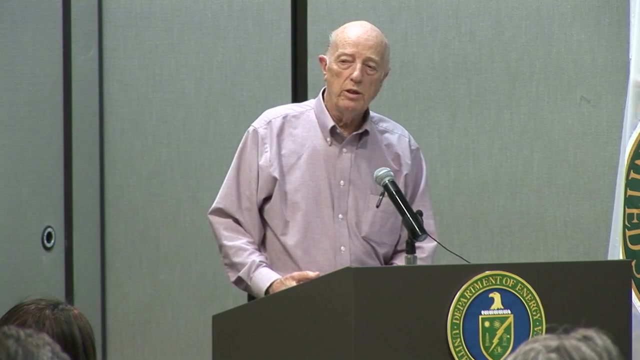 But this curve really, uh is uh a powerful piece of information. Uh, this one is useful with respect to, uh, individual scenarios. Uh, and then there's a whole raft of other things that go with these results, The most important of which is the importance ranking of all the contributors to the risk. 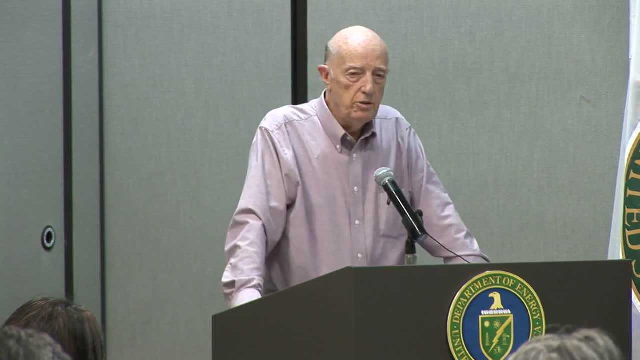 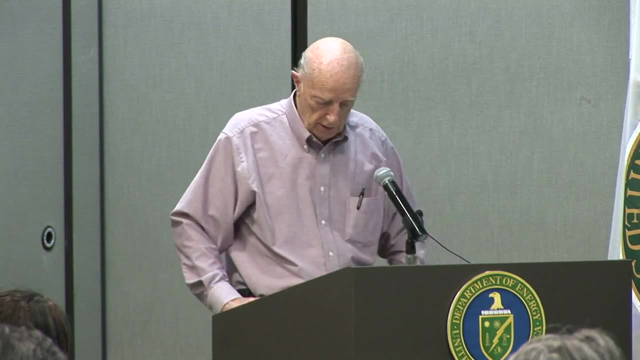 That is really turns out to be and that was just enormous eye-opener in a lot of these facilities, including uh nuclear power plants. So I think that's about all I have that I want to cover Uh. 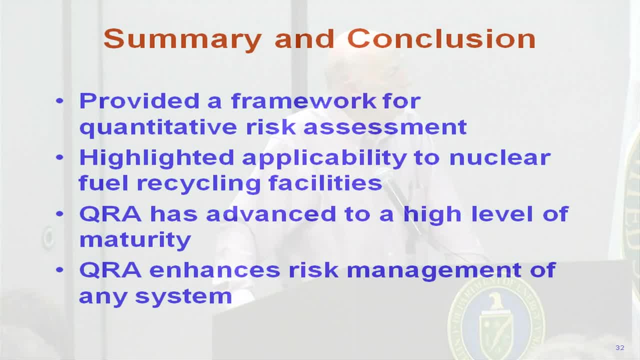 I have the usual conclusion side which says nothing much Uh, but uh, the, the, the businesses uh matured, uh. from the standpoint of, of the government's use of of PRA and its extensions of the